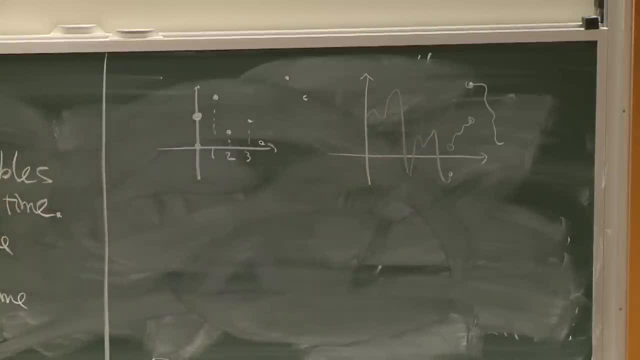 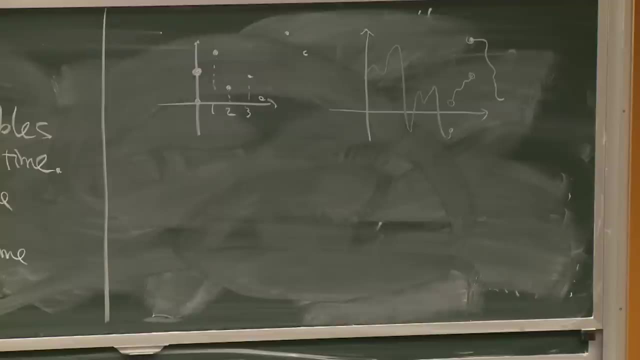 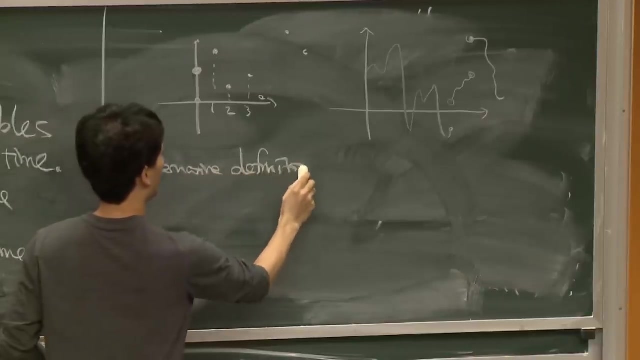 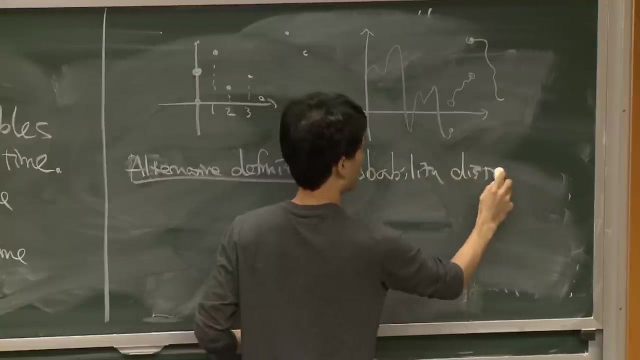 And all these values are random values. okay, That's just a very informal description And a slightly a different point of view which is slightly preferred when you want to do some math with it. is that different? alternative definition? It's a probability distribution over passes. 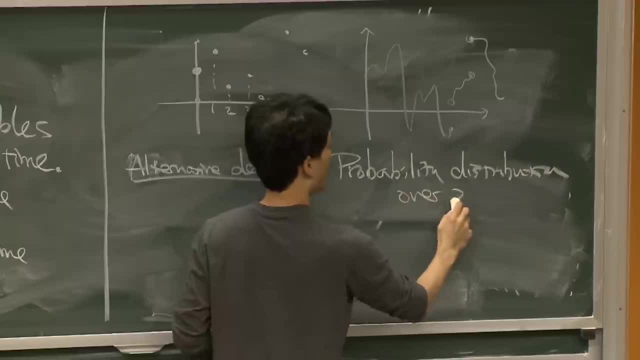 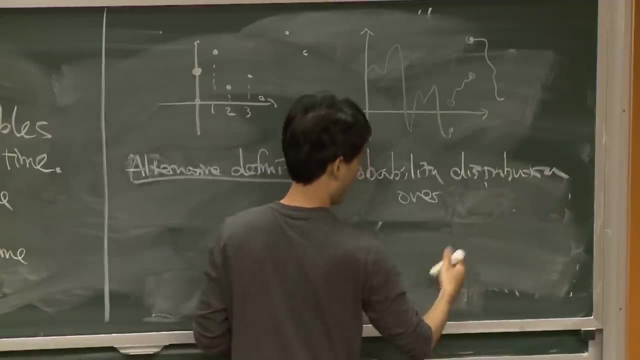 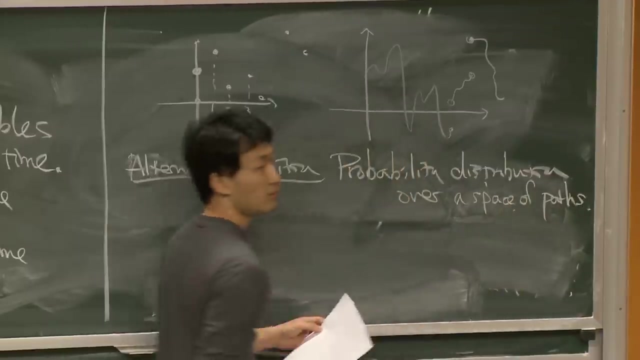 Okay, So, Okay, Okay, Okay. And what is the probability distribution? Okay, What do thesedesịch over a space of partially? So you have all bunch of possible passes that you can take and you're given some probability. 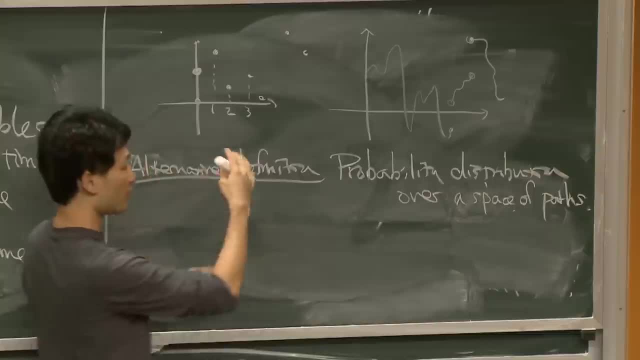 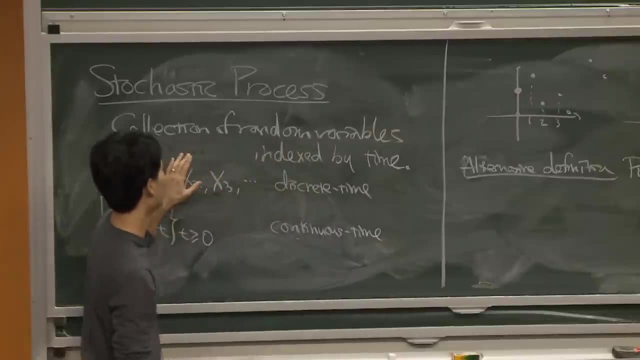 distribution over it, And then that will be one realization. another realization will look something different, and so on, Okay, Okay that it's a collection of random variables indexed by time. But that one, if you want to do some math with it. 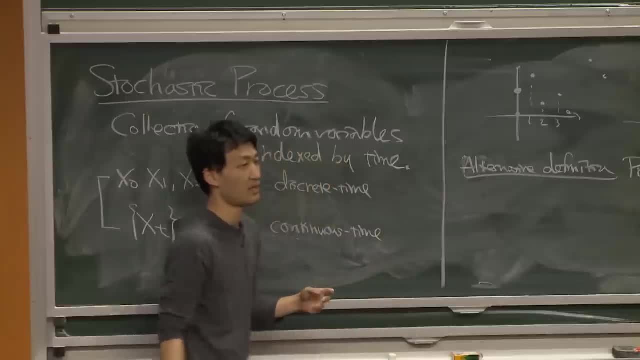 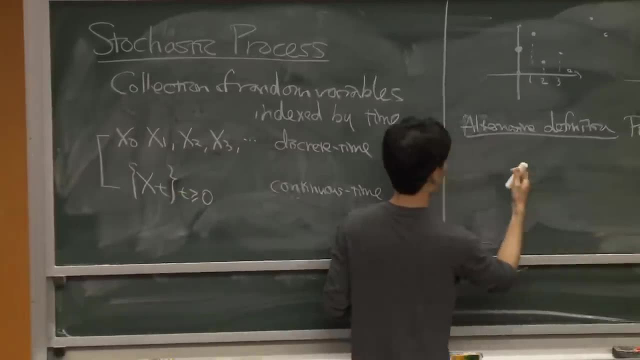 from the formal point of view that will be more helpful, And you'll see why that's the case later. So let me show you some more examples, For example to describe one stochastic process. this is one way to describe stochastic process. 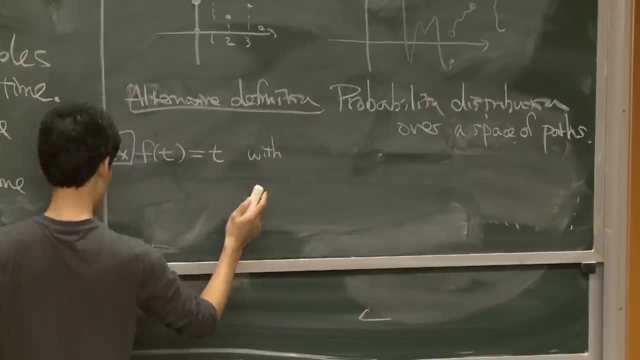 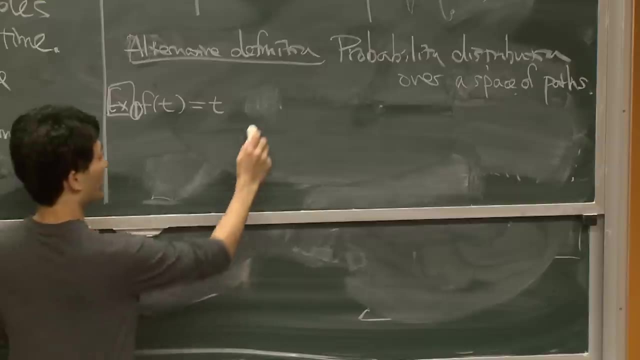 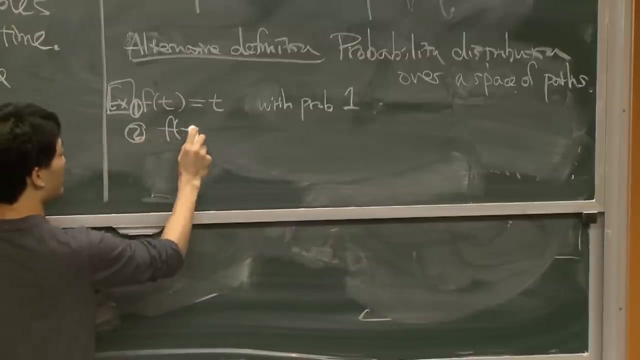 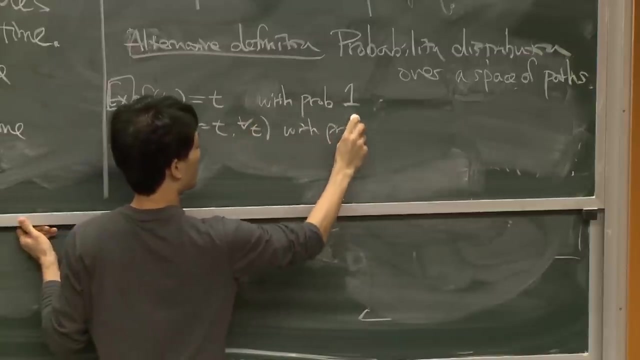 t was. let me show you three stochastic processes. So number one: f t equals t, And this was probability one. Number two: f t is equal to t or all t, with probability half r, f t is equal to minus t. 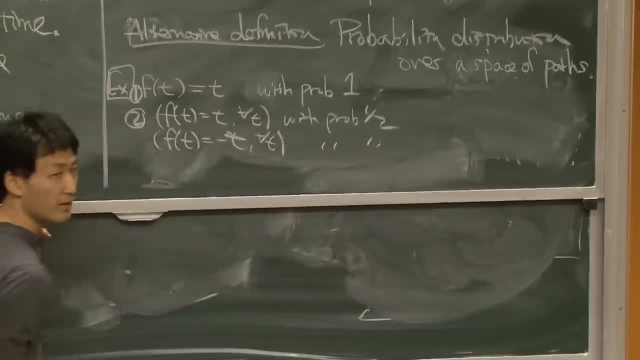 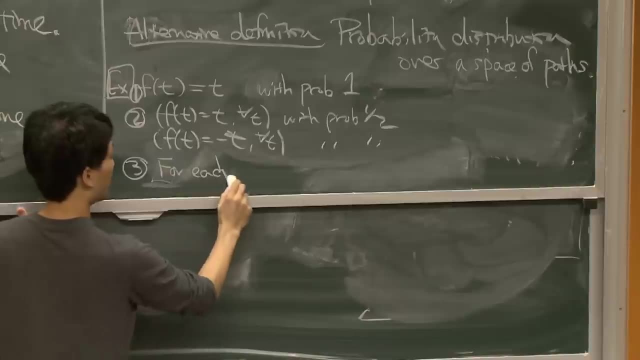 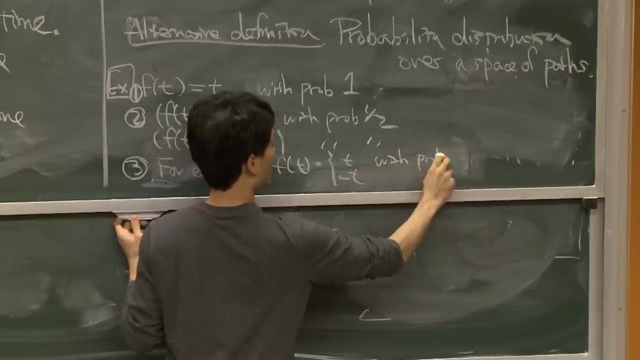 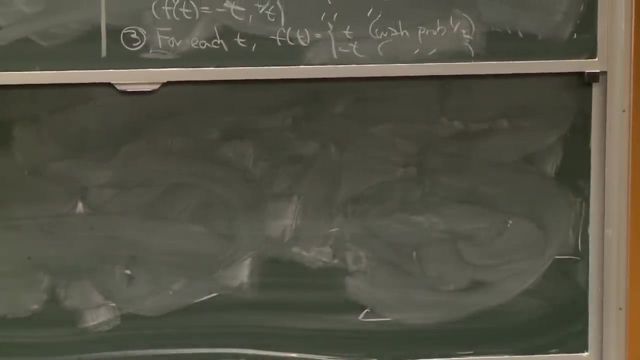 For all t with probability half, And the third one is for each t, f t is equal to t or minus t with probability half. The first one is quite easy to picture. It's really just not even a random. 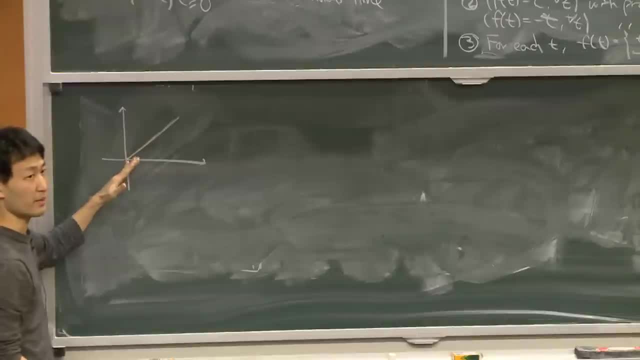 There's nothing random in here. This happens with probability one. Your path just says f, t equals t, And we're only looking at t greater than or equal to 0 here. So that's number one. Number two is either this one or this one. 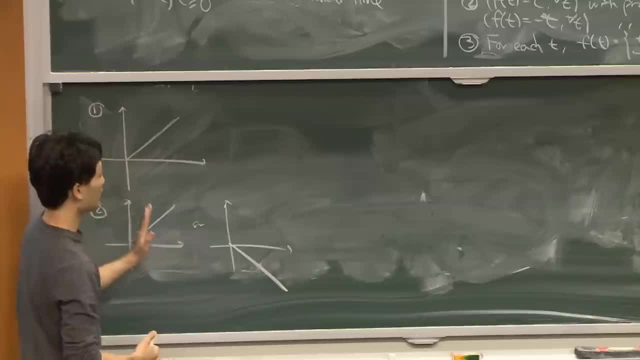 So it is a stochastic process. If you think about it this way, it doesn't really look like a stochastic process, But under the alternative definition you have two possible passes you can take. You either take this path, with 1 over 2,. 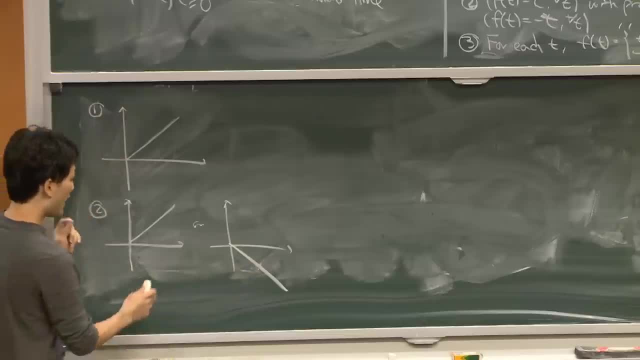 or this path with 1 over 2.. Now, at each point t, your value x. t is a random variable. It's either t or minus t And it's the same for all t, But they are dependent on each other. 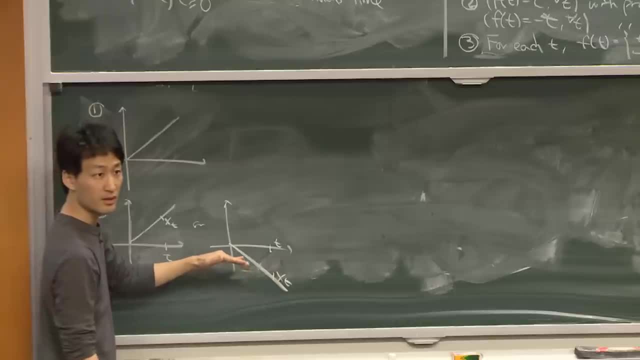 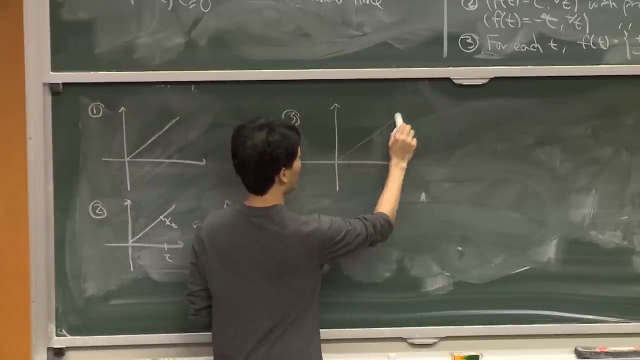 So if you know one value, you automatically know all the other values. And third one is even more interesting. Now, for each t, we get rid of this dependency. So what you'll have is you'll have these two lines going on. 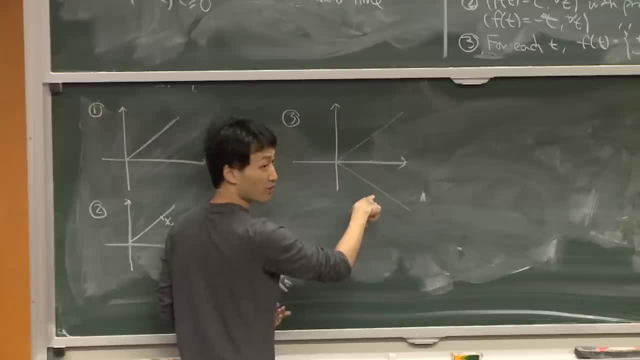 I mean at every single point you'll be either top one or bottom one. But if you really want to draw the picture, it will bounce back and forth up and down infinitely. often It will just look like two lines OK. 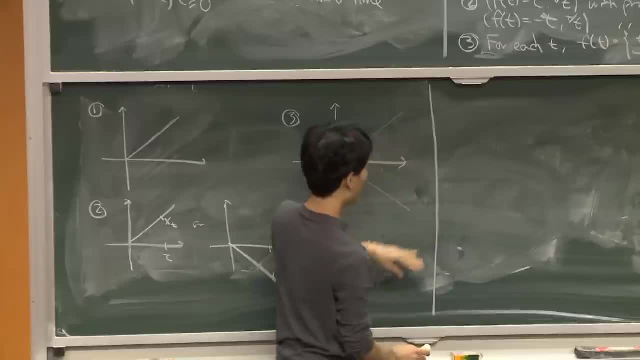 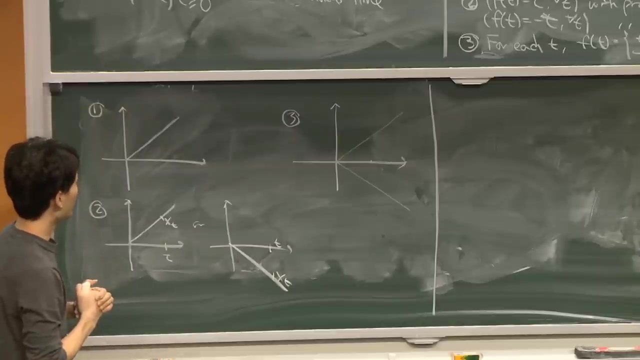 So I hope this gives you some feeling about stochastic processes. I mean why we want to describe it in terms of this language. Just a tiny bit. Any questions? OK, So when you look at a process, when you use stochastic process to model a real life something, 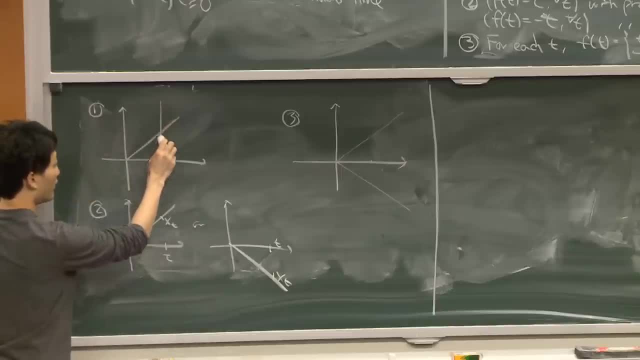 going on like a stock price. usually what happens is your standard time t And you know all the values of the past know, And in the future you don't know. But you want to know something about it. You want to have some intelligent conclusion. 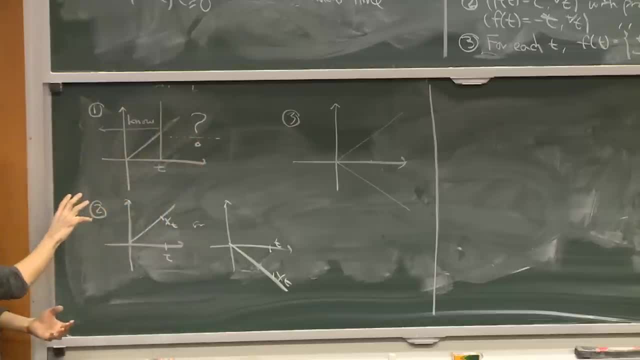 intelligent information about the future based on the past. For this stochastic process it's easy: No matter where you stand at, you exactly know what's going to happen in the future. For this one it's also the same, Even though it's random, once you. 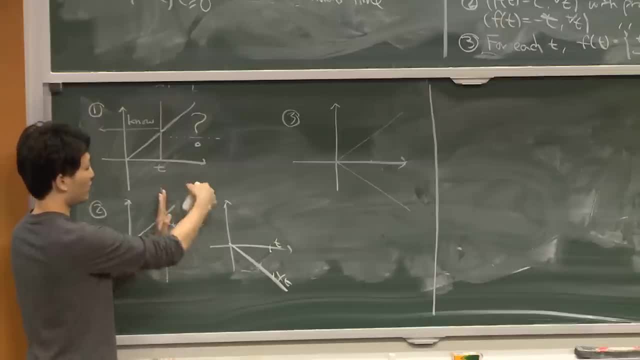 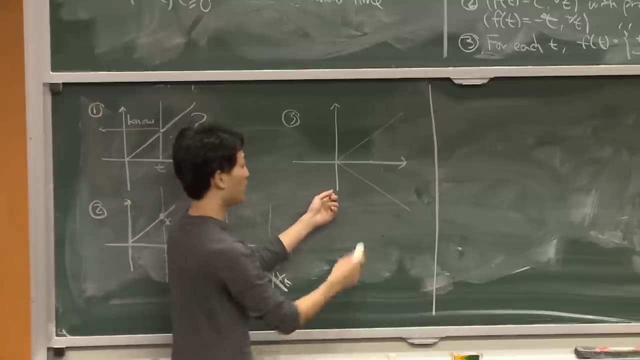 know what happened at some point, you know it has to be this line if it's here and this line if it's there. But that one is slightly different. No matter what you know about the past, even if you know all the values of the past, what happened? 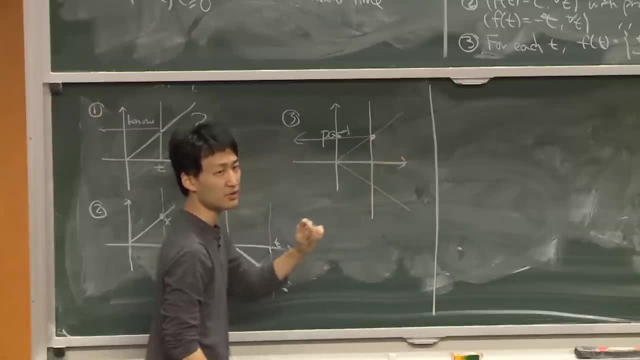 it doesn't give any information at all about the future. Well, it's not true if I say any information at all. We know that each value has to be t or minus t. We just don't know what it is. So when you're given a stochastic process, 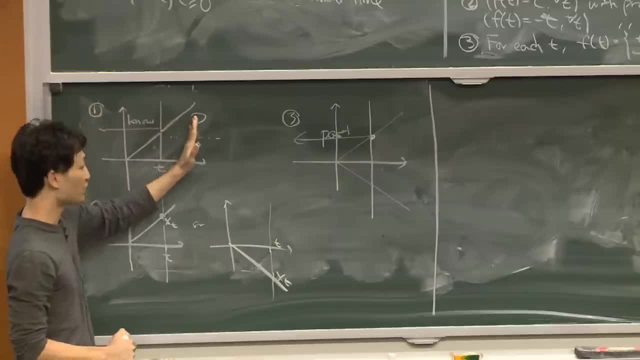 and you're standing at some time. your future? you don't know what the future is, But most of the time you have at least some level of control, given by the probability distribution. Here it was. you can really determine the line. 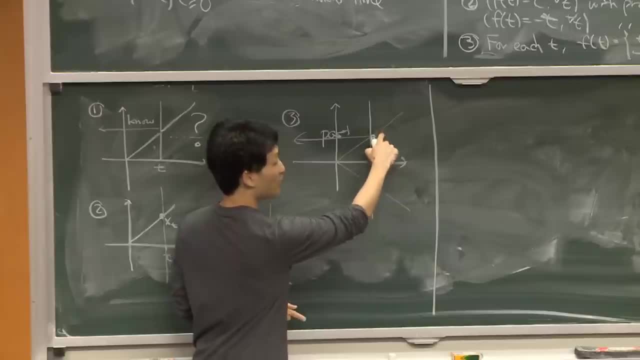 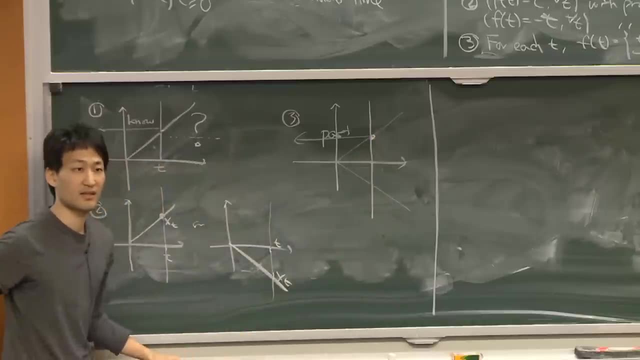 Here, because the probability distribution at each point only gives t or minus t. you know that each of them will be at least 1. That's one of the points, But you don't know more than that. So the study of stochastic processes: 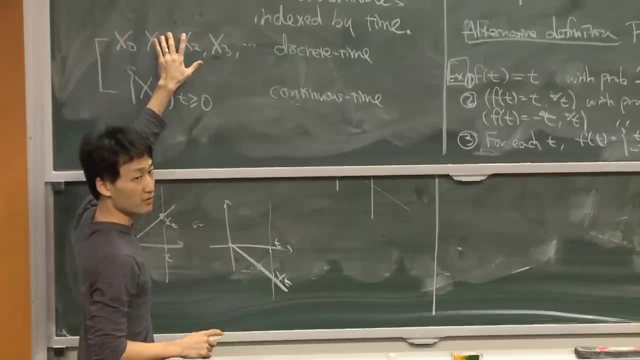 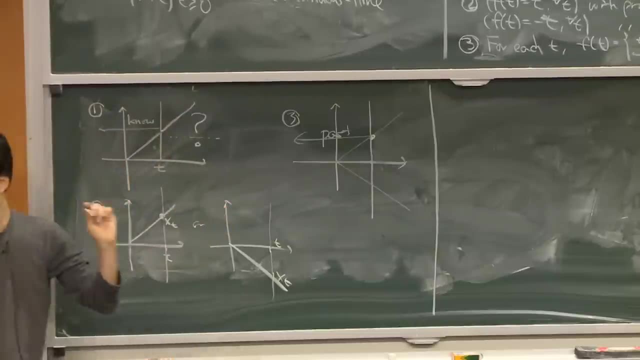 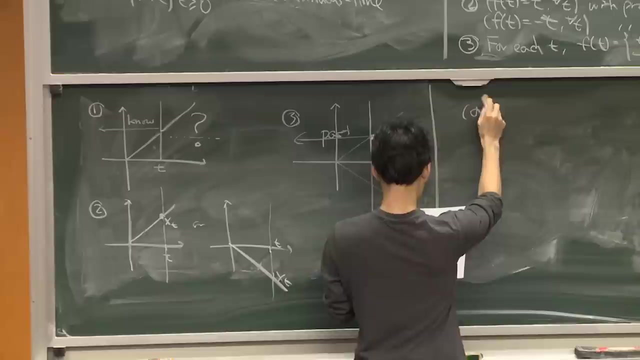 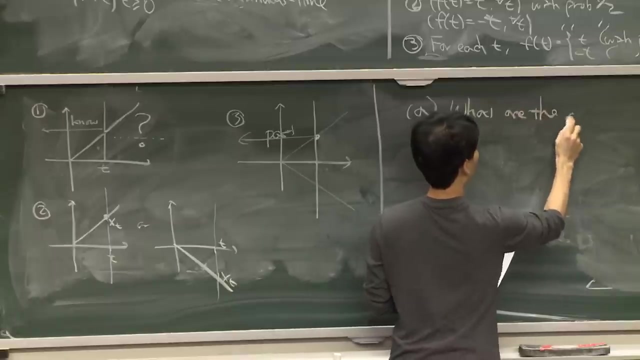 is basically: you look at the given probability distribution and you want to say something intelligent about the future as t goes on. So there are three types of questions that we mainly study here. So A first type is: what are the dependencies in the sequence of values? 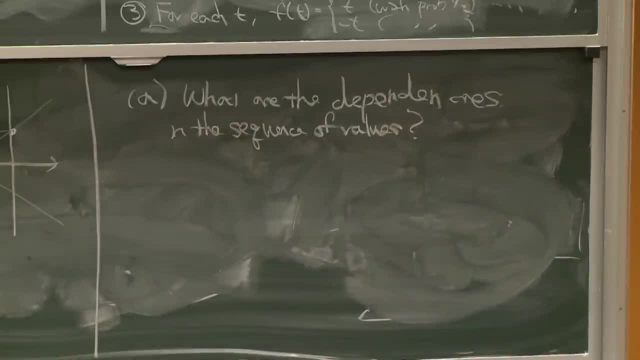 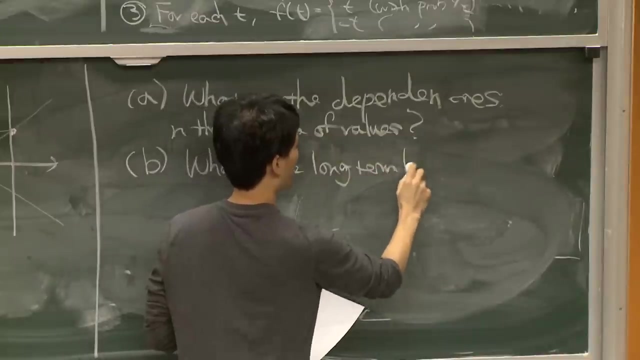 For example, if you know the price of a stock on all past dates up to today, can you say anything intelligent about the future stock prices? Those type of questions. And B is, what is the long-term behavior of the sequence? So think about the law of large numbers. 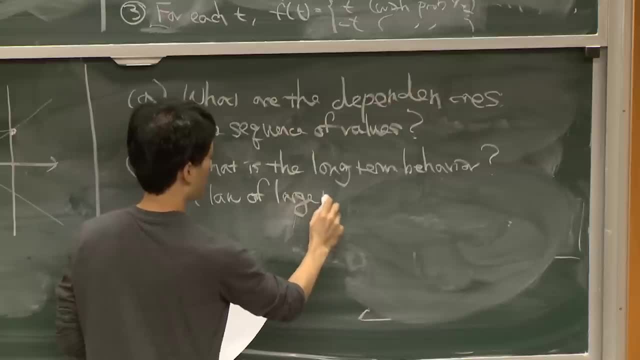 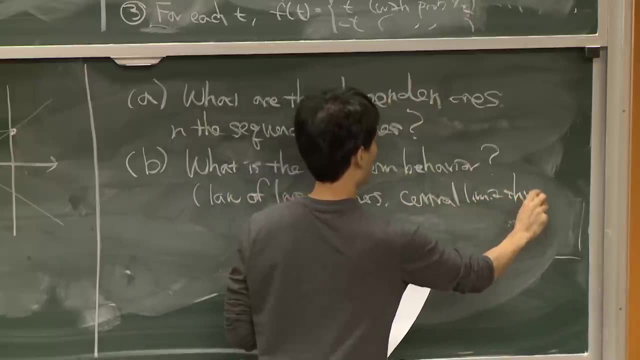 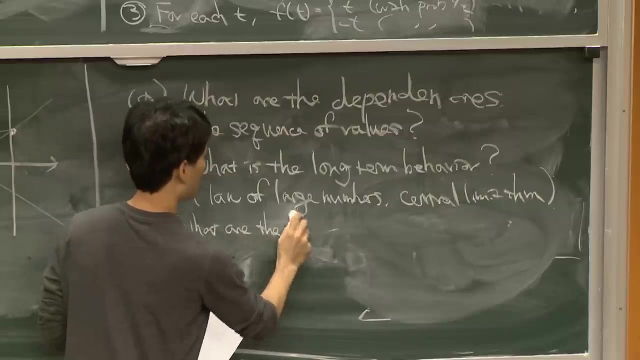 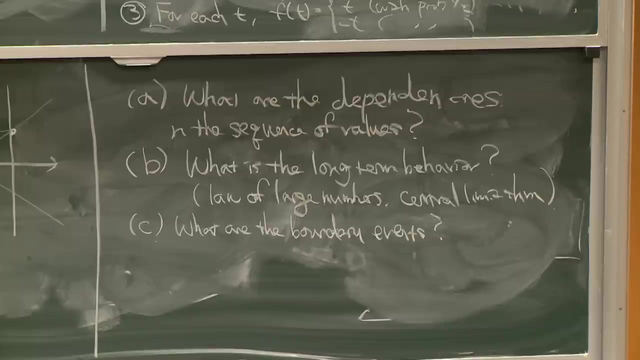 that we talked about last time, our central limit theorem, The third type. this one is less relevant for our course. I'll just write it down. What are the boundary events? How often will something extreme happen, Like? how often will a stock price drop by more than 10%? 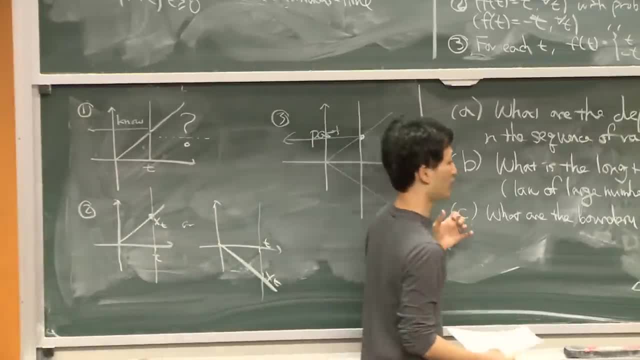 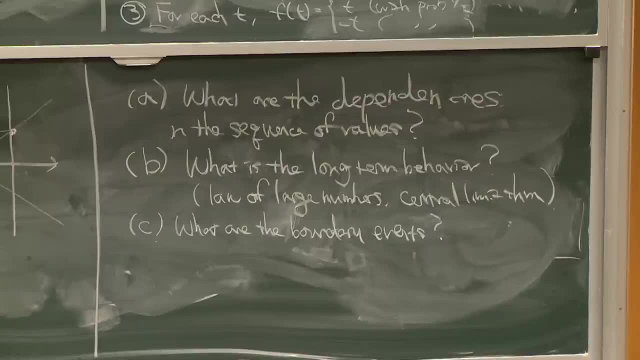 for consecutive five days. It's these kind of events. How often will that happen? Yeah, And for a different example, if you model a call center and you want to know, over a period of time, the probability that at least 90% of the phones 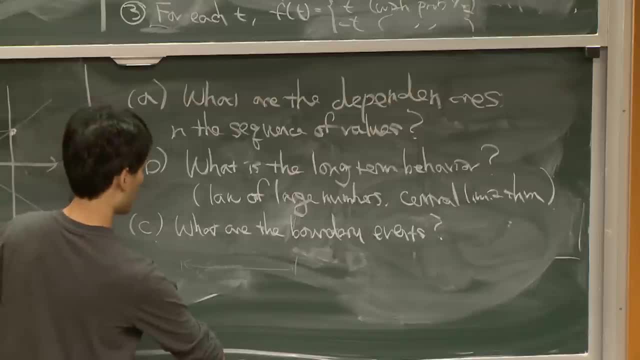 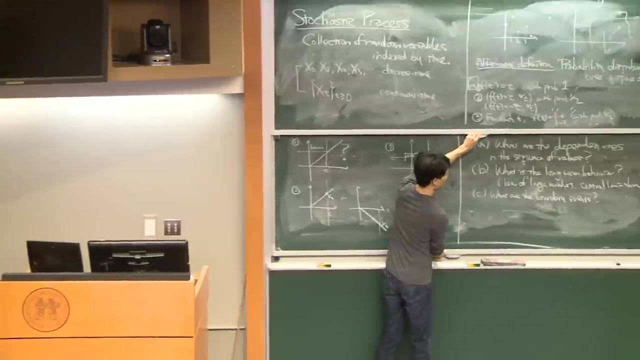 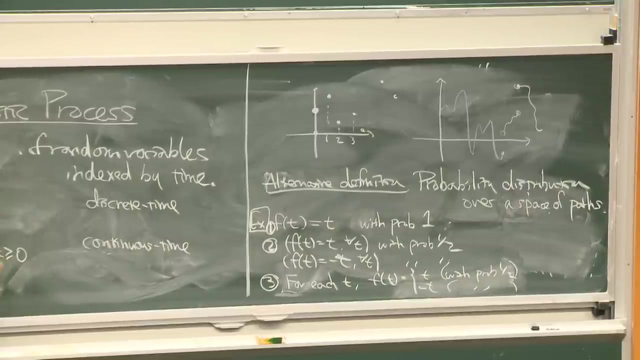 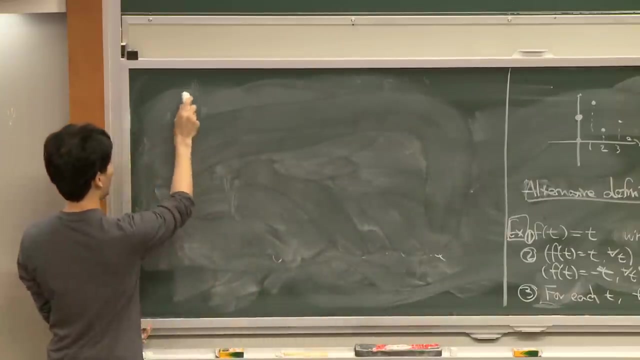 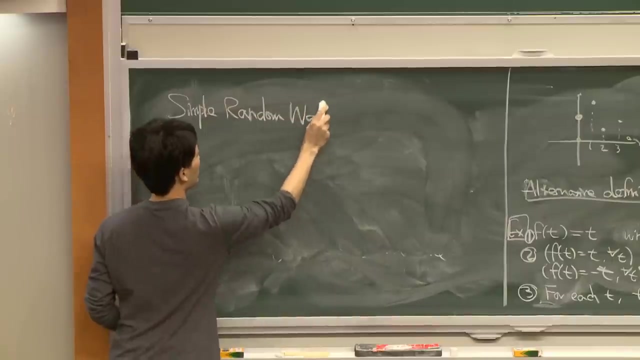 are idle or those kind of things. So that was the introduction. Any questions? OK, Then there are really lots of stochastic processes. One of the most important ones is the simple random walk. OK, So today I will focus on discrete time. 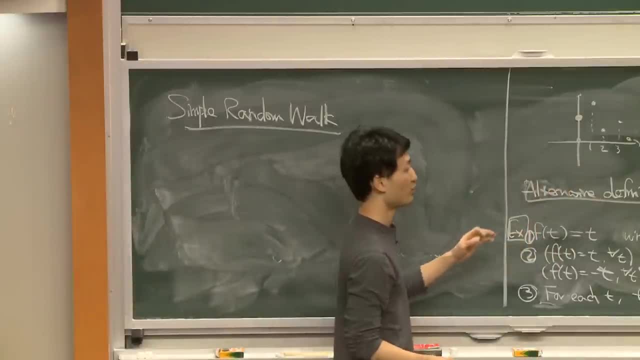 Discrete time stochastic processes. Later in the course we'll go on to continuous time stochastic processes And then you'll see, like Brownian motions And what else Ito's lemma and all those things will appear later. Right now we'll study discrete time. 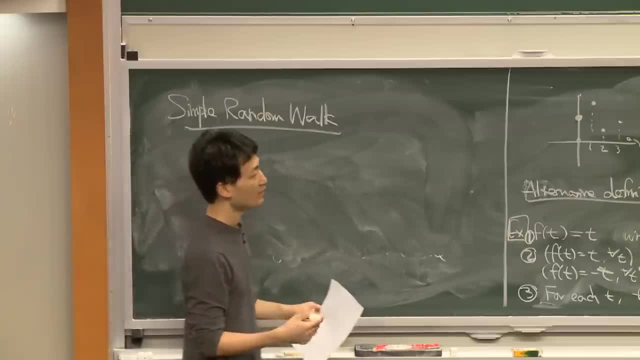 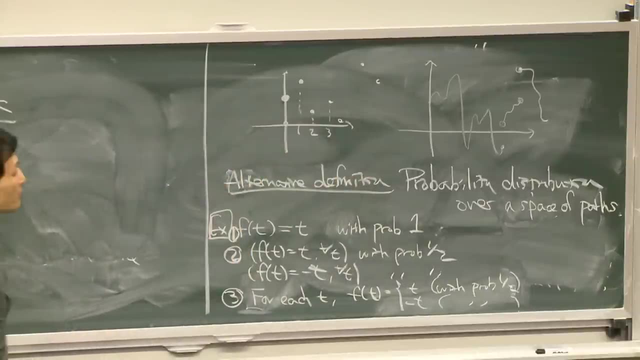 And later you'll see that it's really just an. what is it? They're really parallel. So this simple random walk, you'll see the corresponding thing in continuous time stochastic processes later. So I think it's easier to understand discrete time processes. 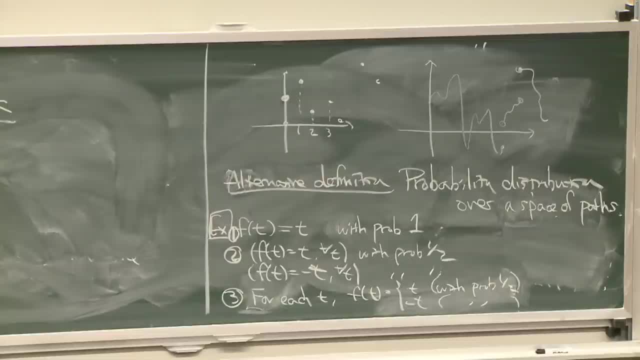 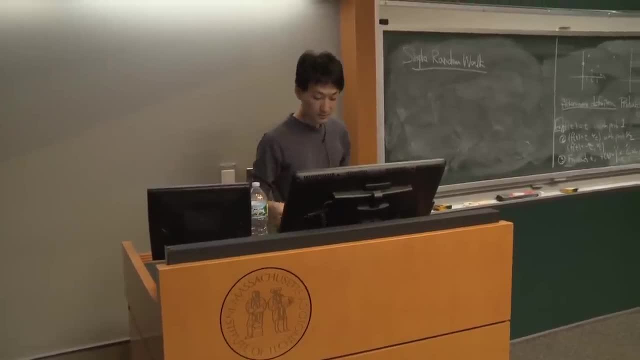 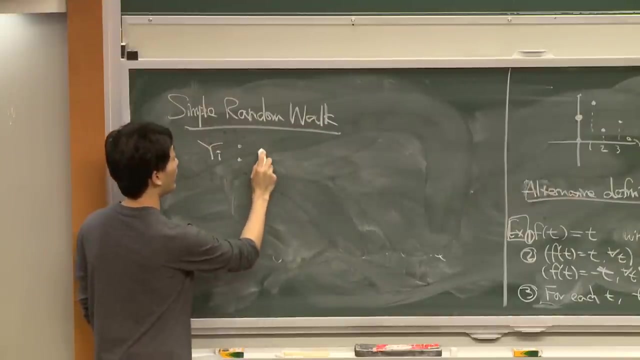 That's why we start with it, But later it will really help if you understand it well, Because for continuous time it will just carry over all the knowledges. What is a simple, random walk? Let A, y, i, b, i, i, d, identical and independently. 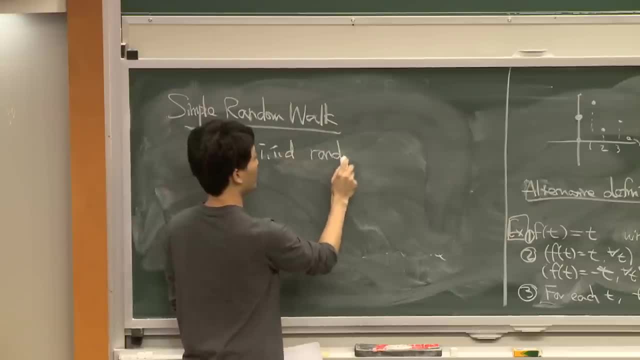 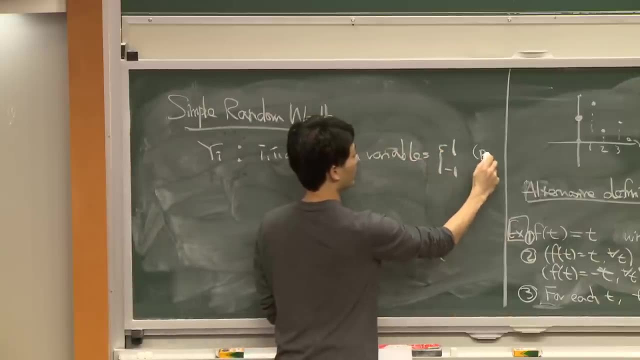 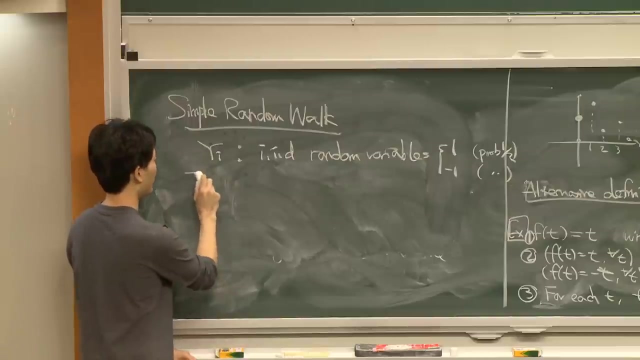 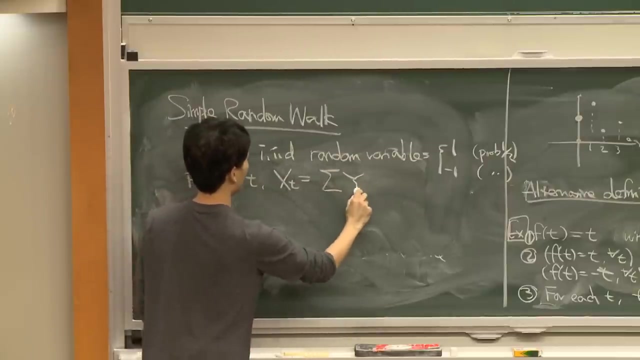 independent And then identically distributed random variables taking values 1 or minus 1, each with probability 1 half. Then define for each time t, x sub t, as the sum of y, i from i equals 1 to t. 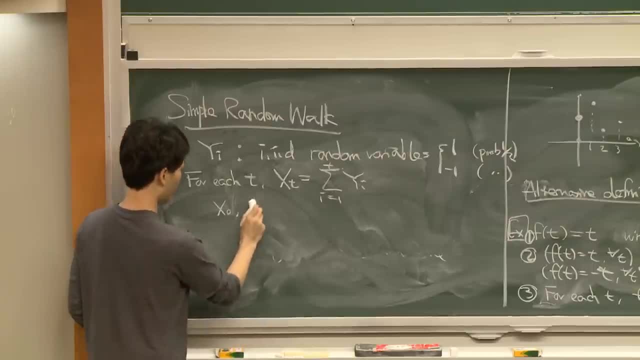 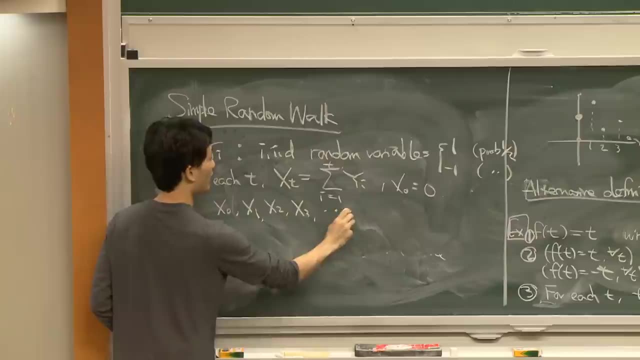 Then the sequence of random variables, and x0 is equal to 0.. x0, x1, x2, and so on is called a one-dimensional, simple random walk, But I'll just refer to it as simple random walk or random walk. 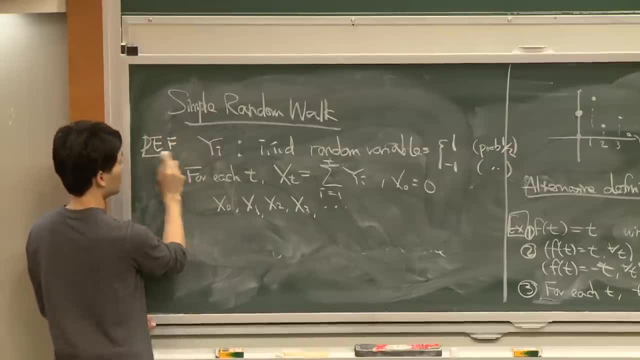 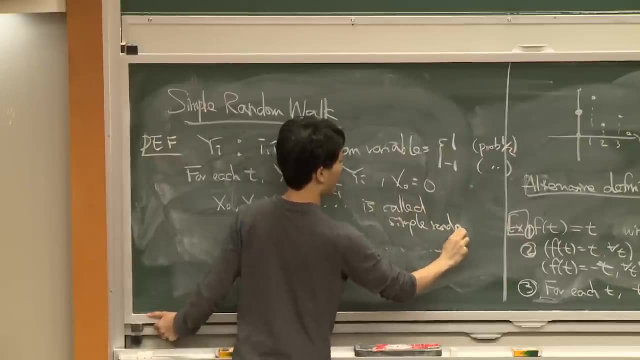 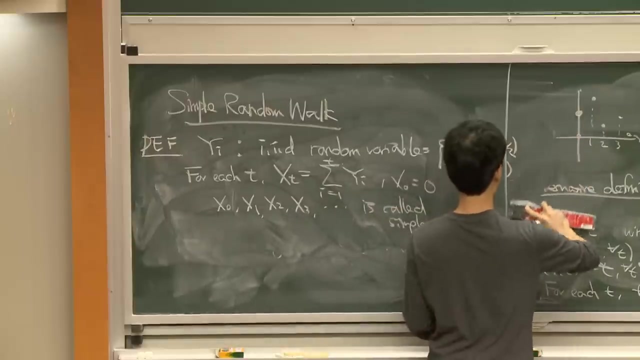 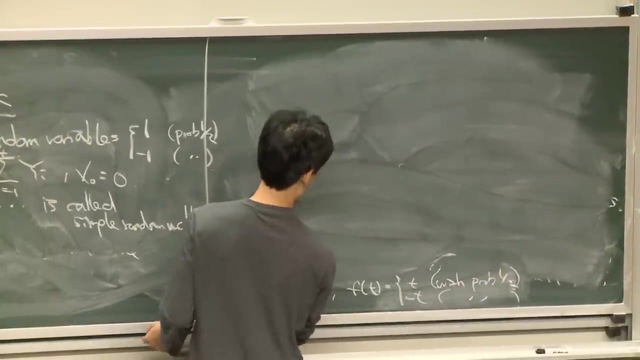 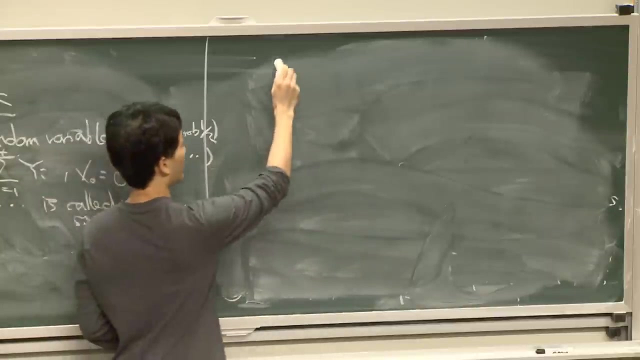 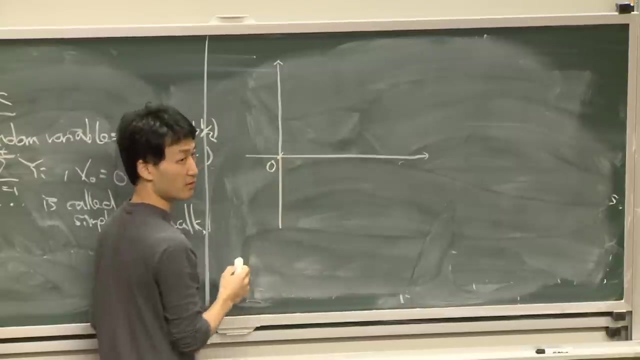 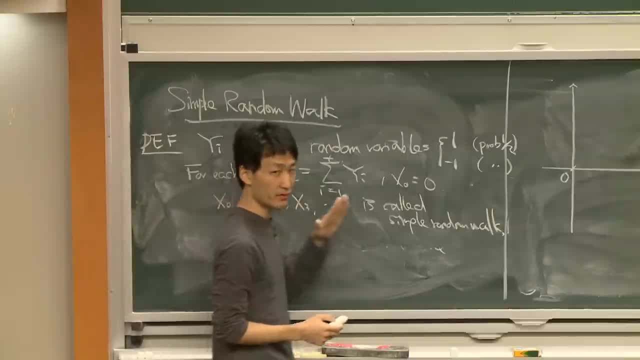 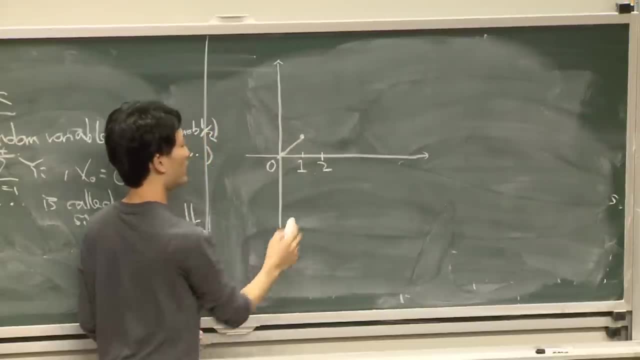 And then you start at 0. And then you start at 0.. Depending on the value of y1,, you will either go up or go down. Let's say we went up, That's at time 1.. Then at time 2, depending on your value of y2,. 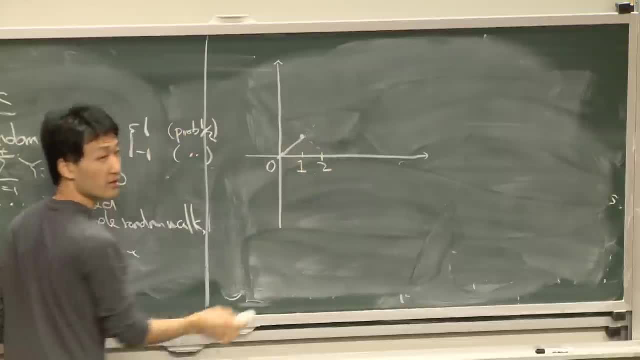 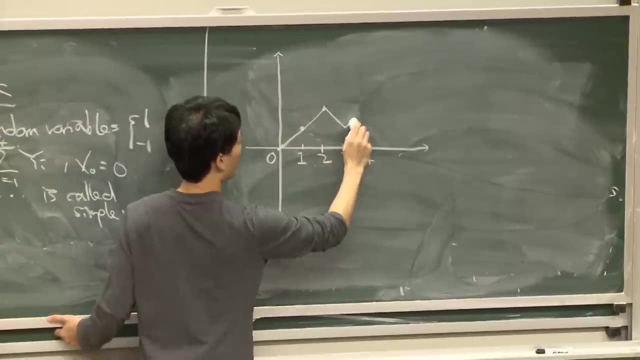 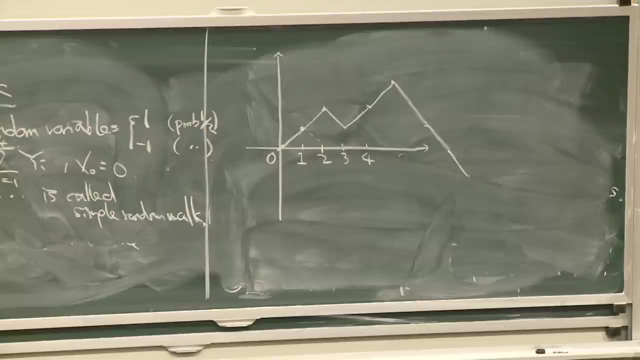 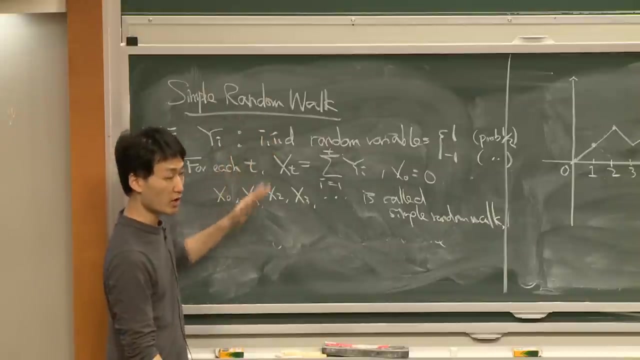 you will either go up one step from here or go down one step from there. So let's say we went up again, Down, up up, something like that, And it continues. Another way to look at it, the reason we call it a random walk. 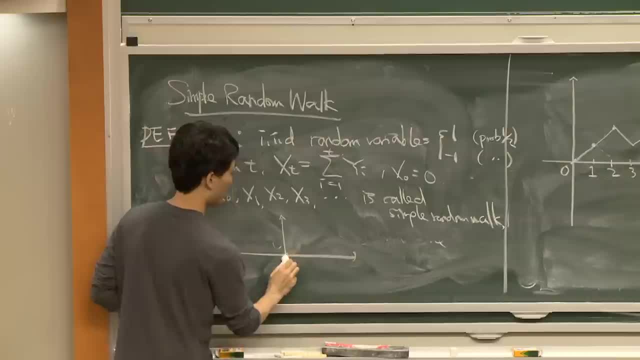 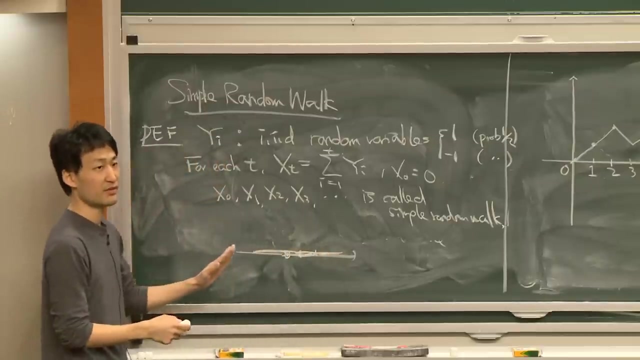 is, if you just plot your values of xt over time on line, then you start at 0. You go to right, So you go to right, right, left, right, right, left, left, left, left. So the trajectory is like a walk you take on this line. 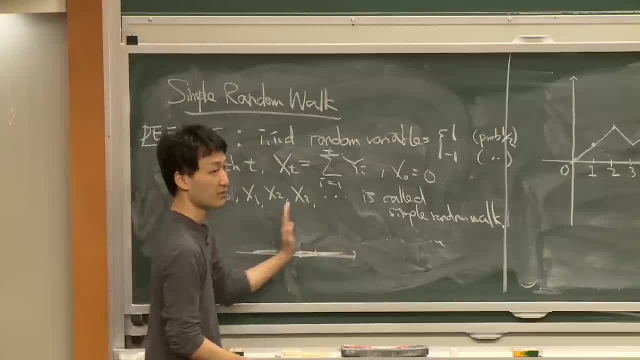 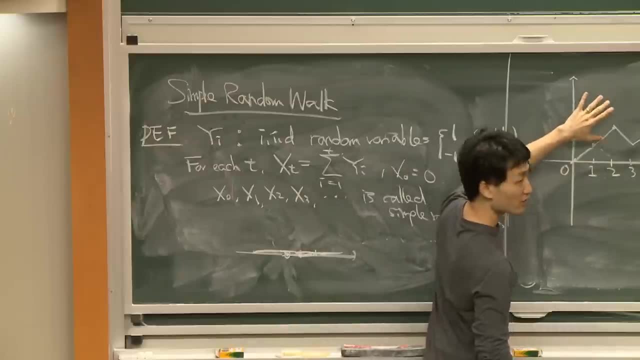 But it's random And each time you go to the right or left, right or left, right or left. So that was two representations. One is this picture looks a little bit more clear Here. I just lost everything I drew. 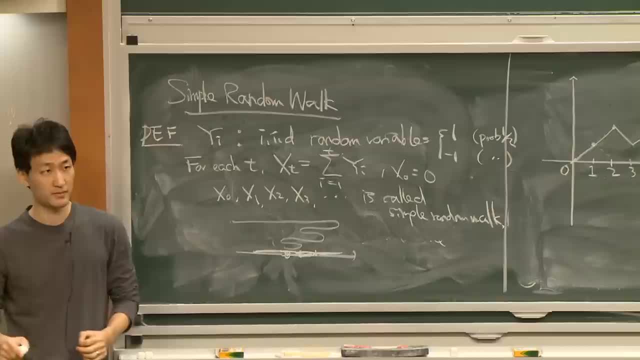 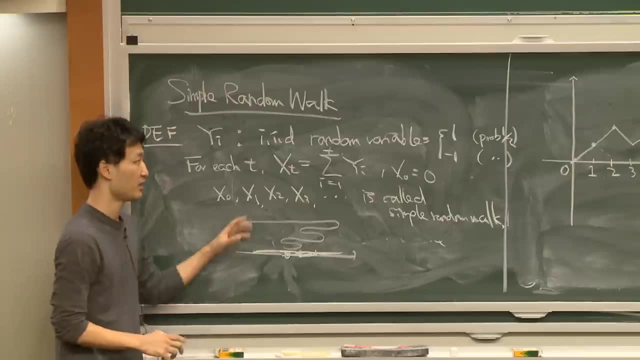 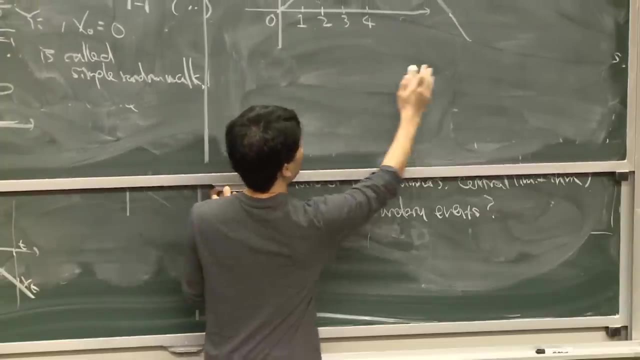 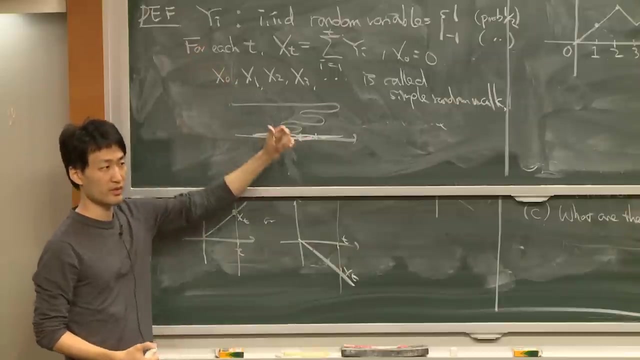 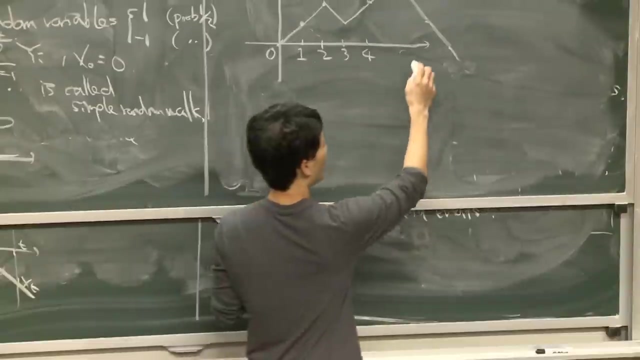 Something like that, The trajectory. OK, So from what we learned last time, we can already say something intelligent about the symbol or the box, For example. If you apply central limit theorem to the sequence, what is the information you get? So over a long time, let's say t is way far away. 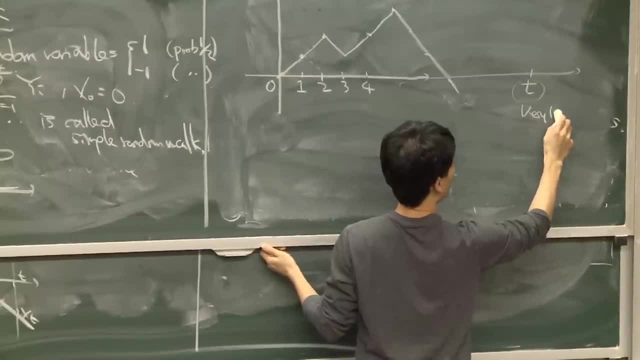 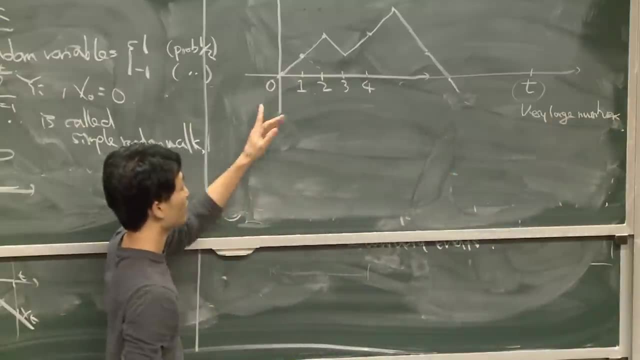 like a huge number, very large number. What can you say about the distribution? You can say: well, it's a big number. What can you say about the distribution? What can you say about the distribution of this? at time t It's close to 0.. 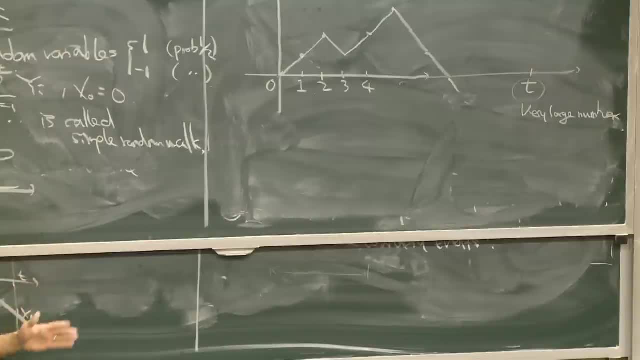 Close to 0.. But by close to 0, what do you mean? The scale. There should be a scale. I mean some people would say that 1 is close to 0.. Some people would say that 100 is close to 0.. 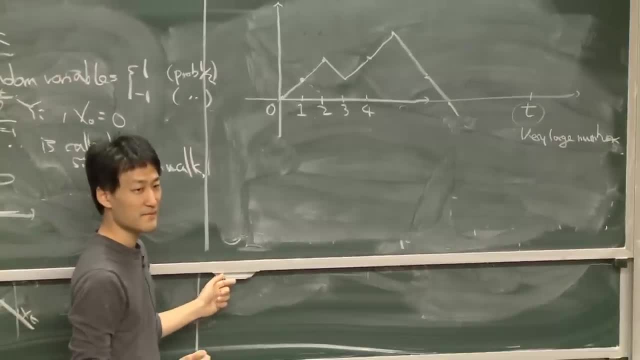 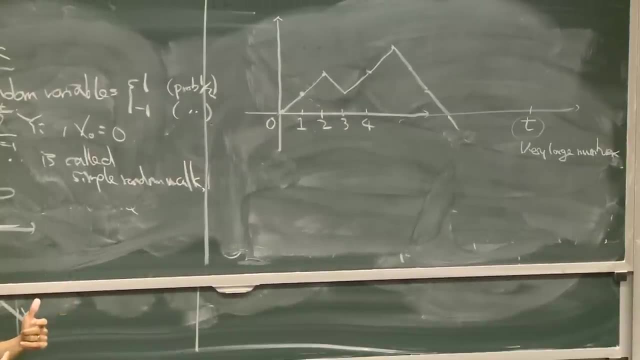 Do you have some degree of how close it will be to 0?? Anybody, Variance will be small. Sorry, Variance. Variance will be small. About how much will the variance be? 1 over n. 1 over n. 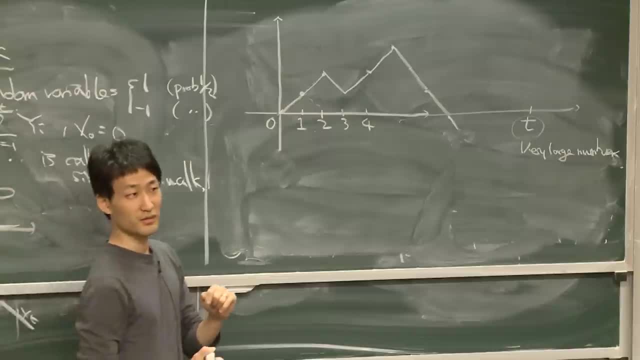 1 over n, 1 over t. Anybody else? 1 over t. squared 1 over square root t Variance will be 1 over t. Oh right, Sorry. Variance will be 1 over t. 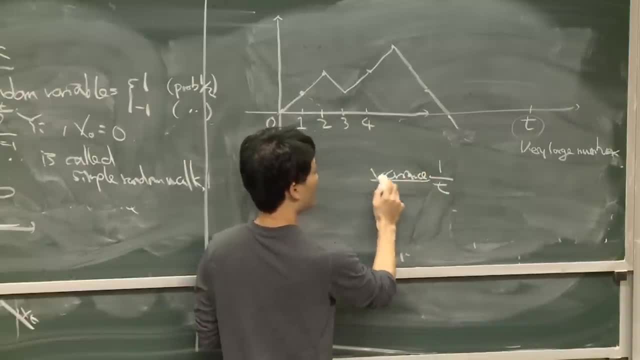 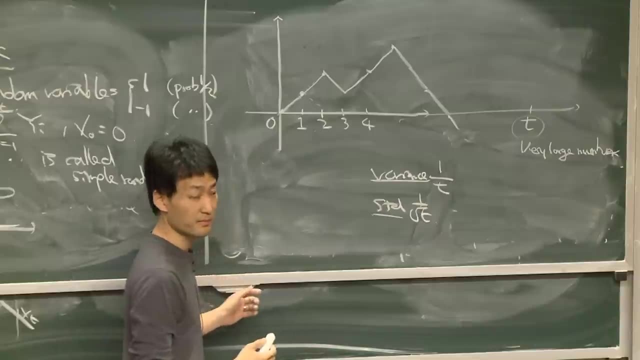 Yeah, And standard deviation will be 1 over square root t. What I'm saying is. What I'm saying is my central limit theorem. Are you looking at the sum or are you looking at the? I'm looking at the xt. 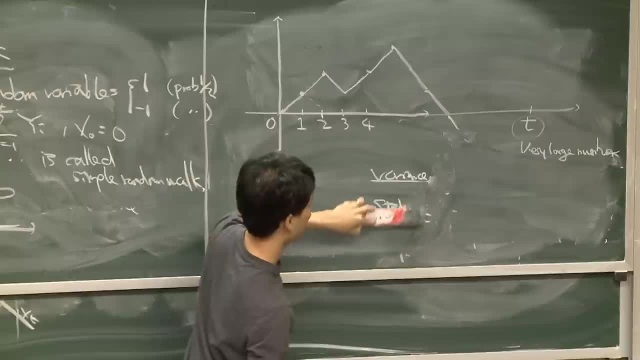 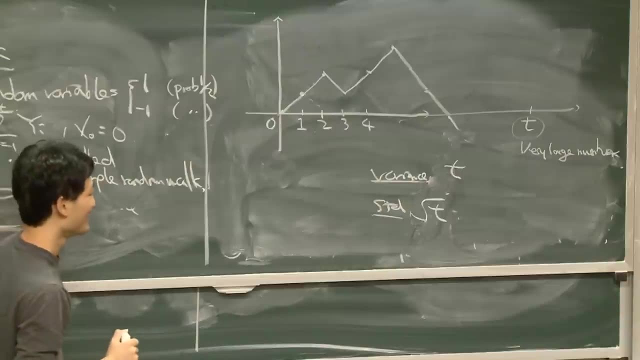 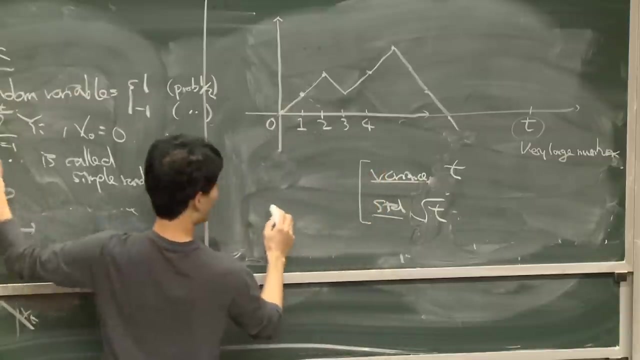 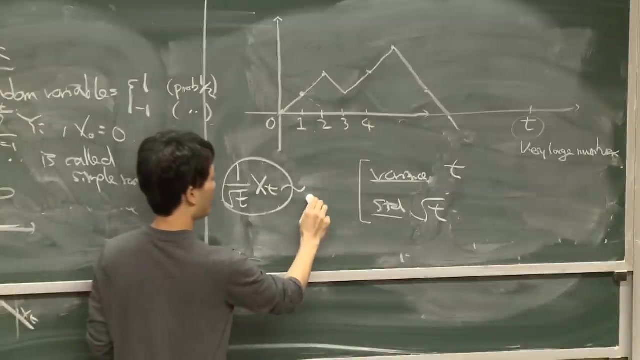 Ah, That's a very good point. t n squared t. Thank you, Very different to that. Yeah, Very, very different. Yeah, Sorry about that. The reason is because xt 1 over square root t times xt. we saw last time that this, if t is really really large. 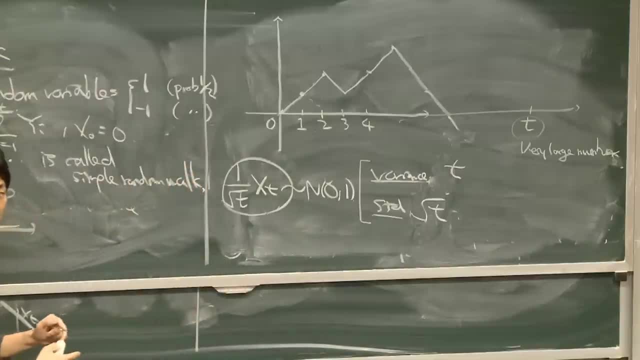 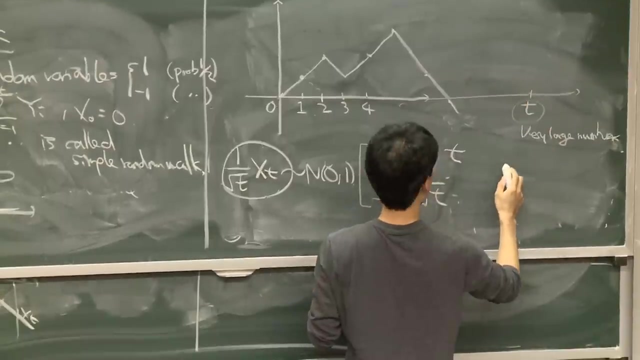 this is close to normal distribution: 0, 1.. So if you just look at it, xt over square root t will look like normal distribution. That means the value at t will be distributed like a normal distribution, with mean 0 and variance squared t. 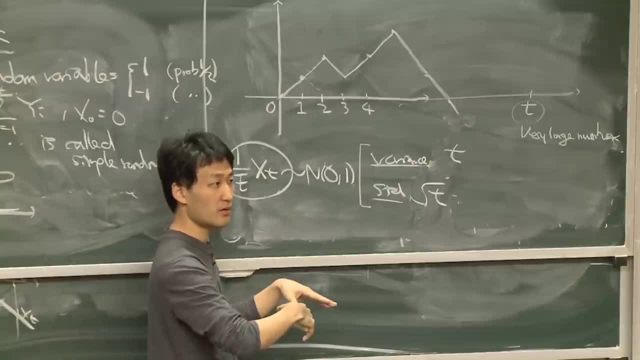 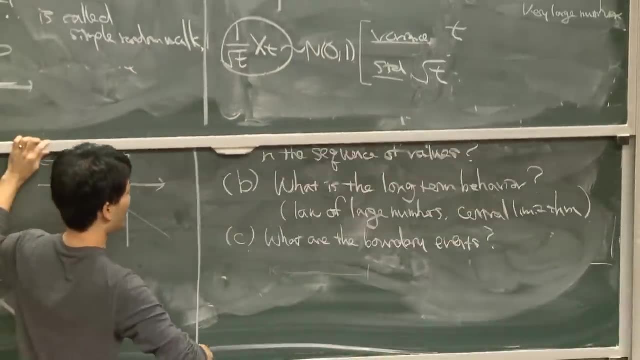 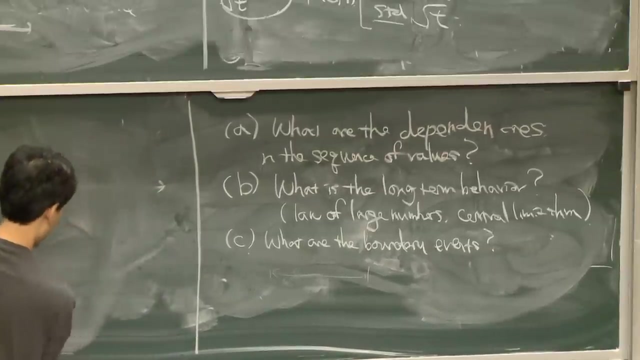 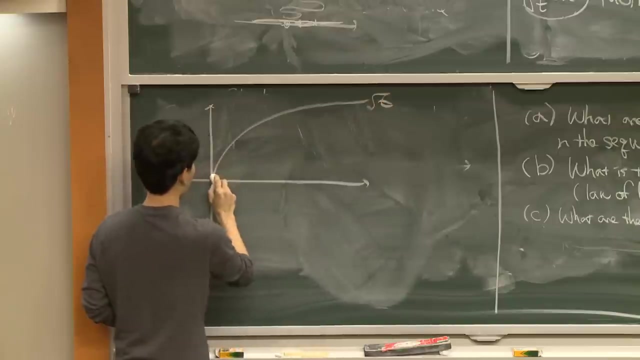 So what you said was right. It's close to 0.. And the scale you're looking at is about square root t, So it won't go too far away from the 0.. That means, if you draw these two curves, square root t. 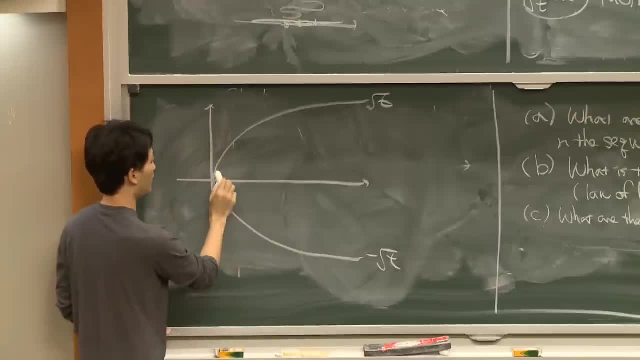 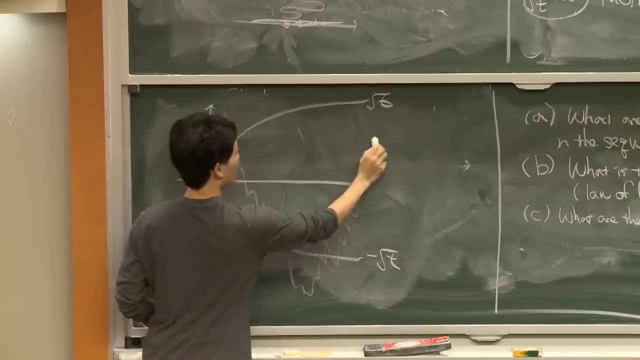 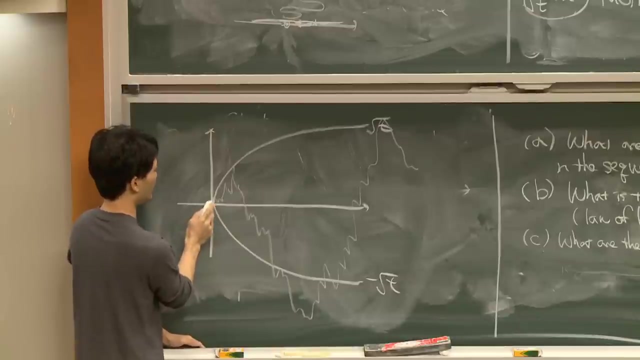 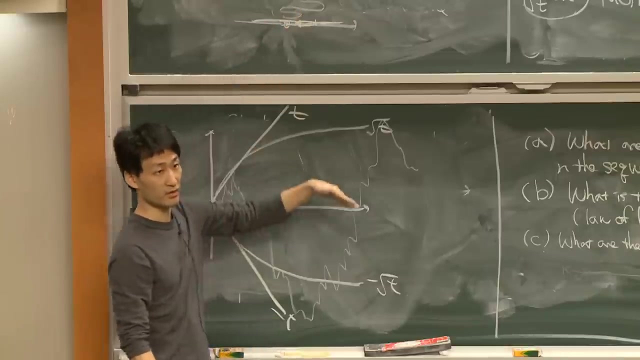 minus square root t. your simple random walk on a very large scale won't go too far away from these two curves, Even though the extreme values you can take- I didn't draw it correctly- is t and minus t, Because all values can be 1 or all values can be minus 1.. 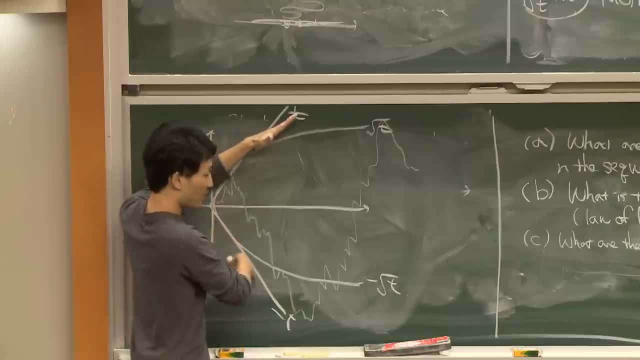 Even though, theoretically, you can be that far away from your x-axis, in reality what's going to happen is you're going to be really close to 0.. You're going to be really close to this curve square root t. You're going to play within this area mostly. 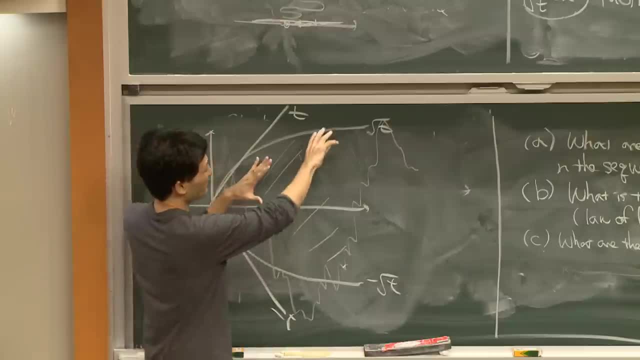 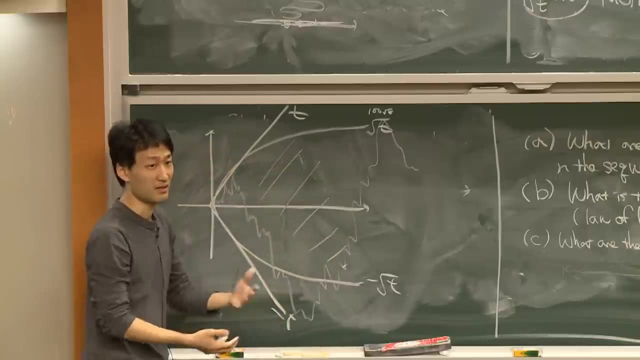 So yeah, that was a very vague statement. You won't deviate too much. So if you take 100 square root t, you'll be inside this interval like 90% of the time. If you take this to be like 10,000 times square root t, 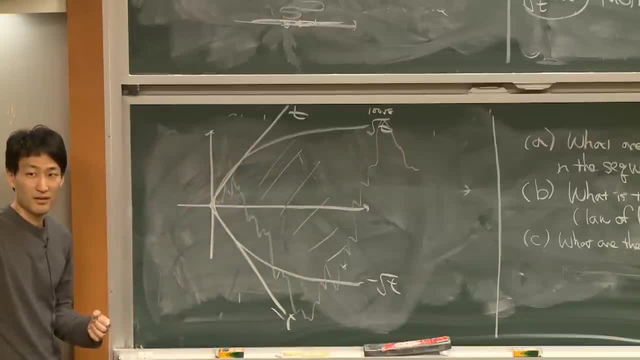 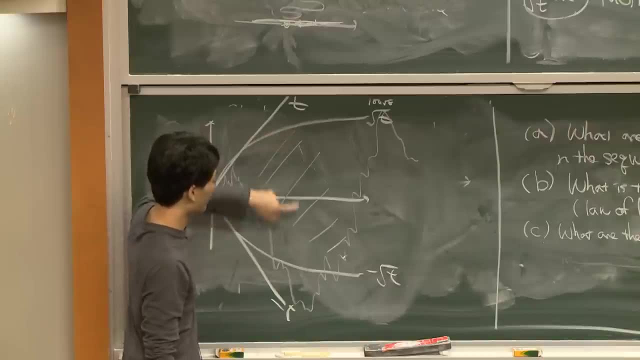 almost 99.9%, Something like that. And there's even a theorem saying you will hit these two lines infinitely often. So if you go over time a very long period, for a very, very long time, you live long enough. then, even if you go down here, even in this picture, 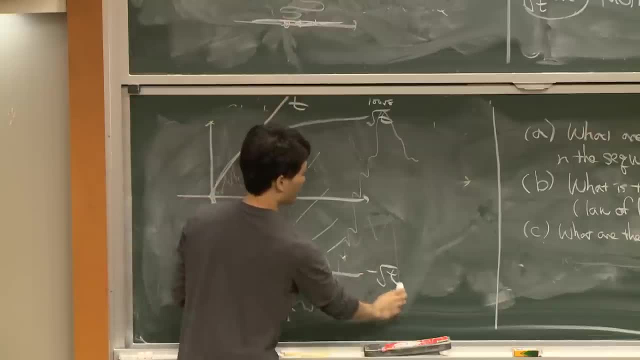 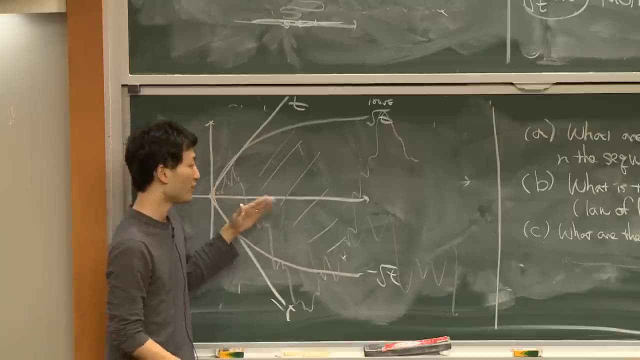 you might think: OK, in some cases it might be the case that you always play in the negative region. Yeah, Yeah, Yeah, Yeah, Yeah, Yeah. There's a theorem saying that that's not the case with probability 1.. 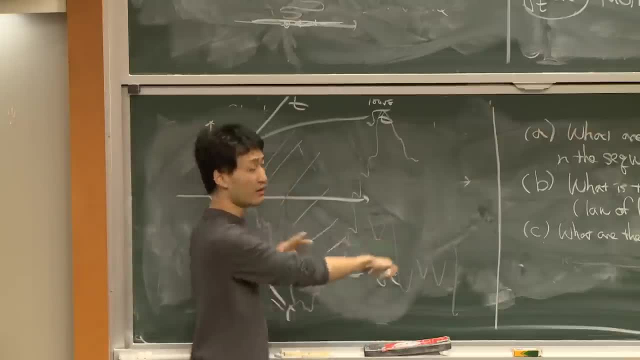 If you go to infinity, you will cross this line infinitely often And in fact, you will meet these two lines infinitely often. OK, So those are some interesting things about simple random mock. really There are a lot more interesting things, but I have. 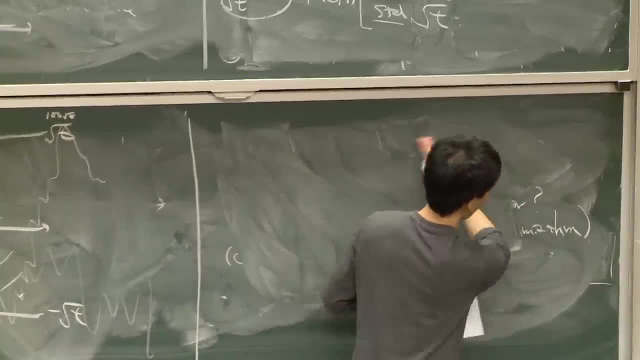 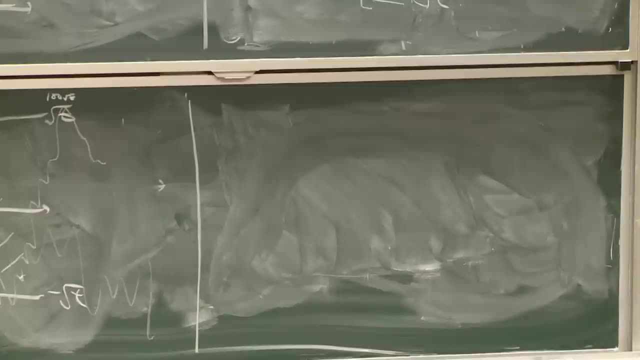 I'm just giving an overview in this course, So Unfortunately I can't talk about all of these fun stuff. But let me still try to show you some properties and one nice computation on it. So proposition, So some properties of random walk. 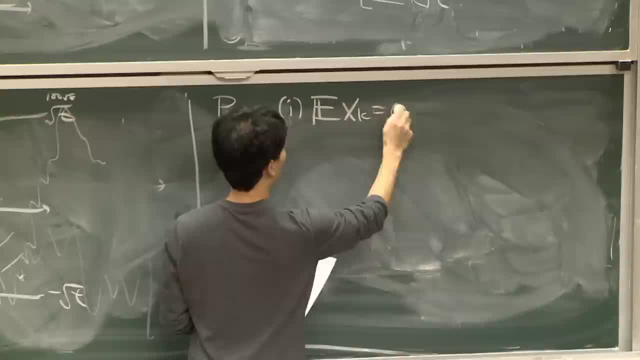 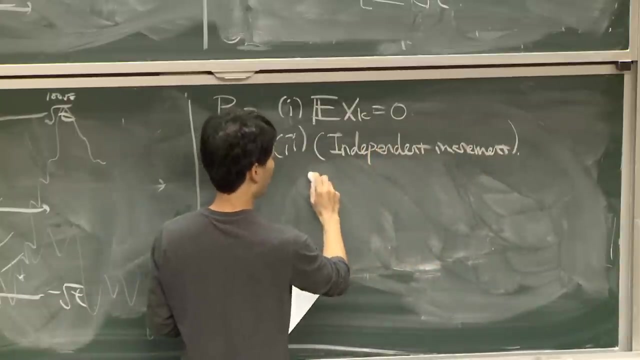 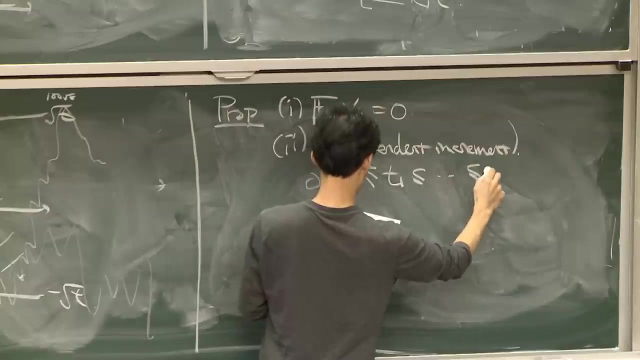 First expectation of xk is equal to 0.. That's the expectation of xk. That's really easy to prove. Second important property is called independent increments. So if you set- look at these times- t0,, t1, up to tk. 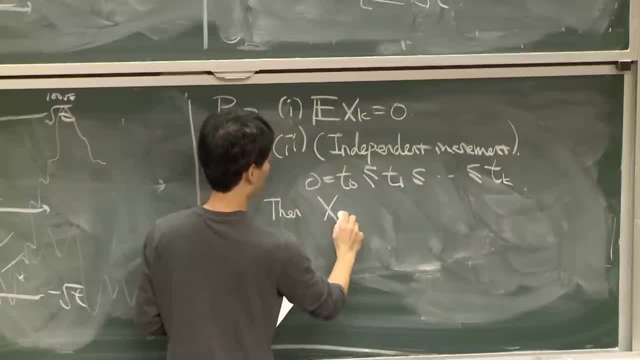 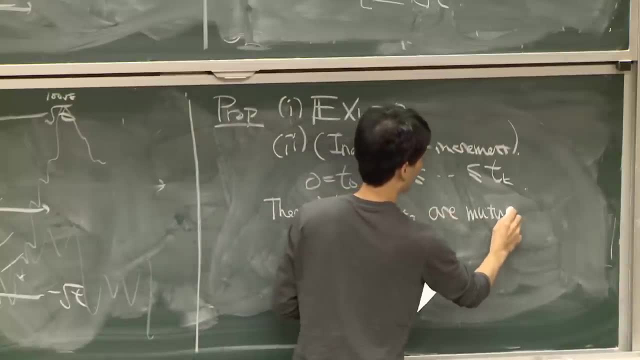 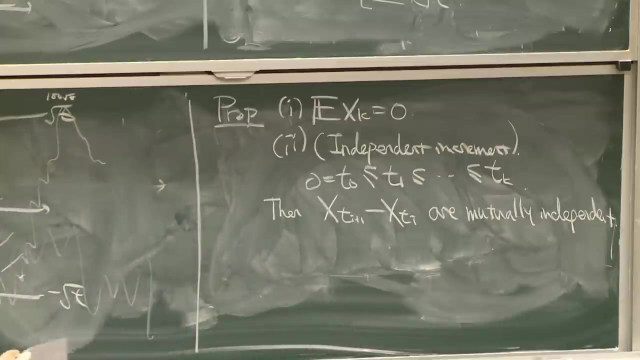 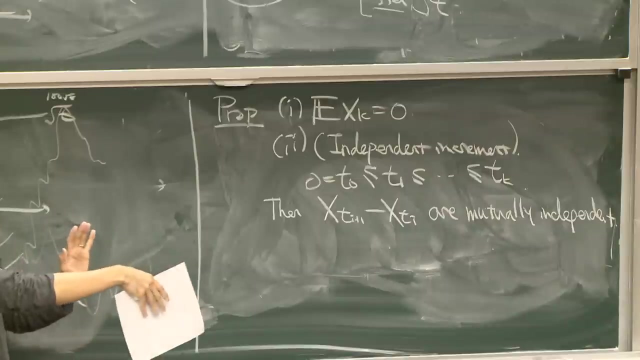 then random variables- x sub ti, plus 1, minus 1, plus 1, plus 1, minus x sub ti are mutually independent. So what this says is, if you look at what happens from time 1 to 10, that is irrelevant to what happens from 20 to 30. 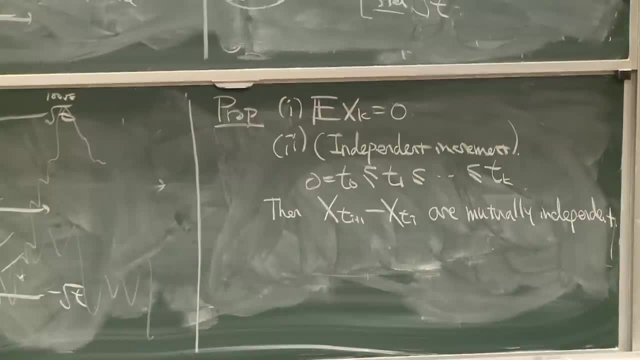 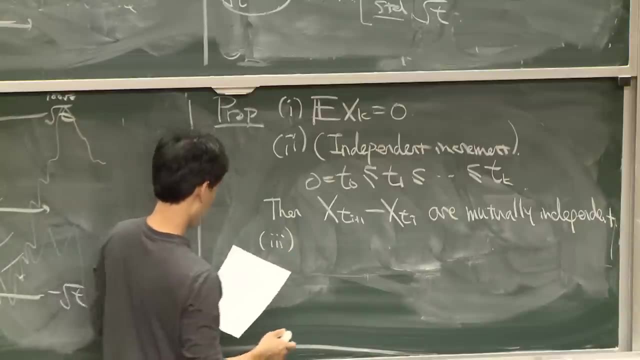 And that can easily be shown by the definition. I won't do that, but I'll try to do it as an exercise. 30. 30., 30., 30., 30. 30. 31 is called stationary. 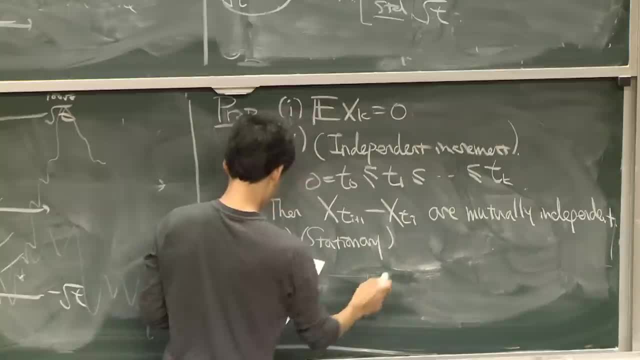 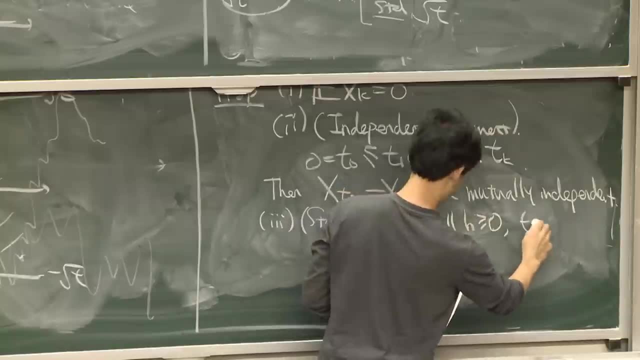 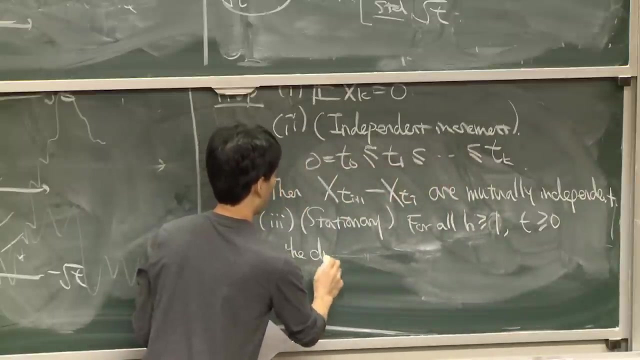 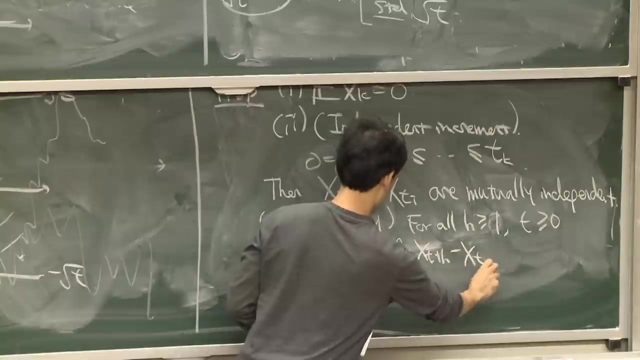 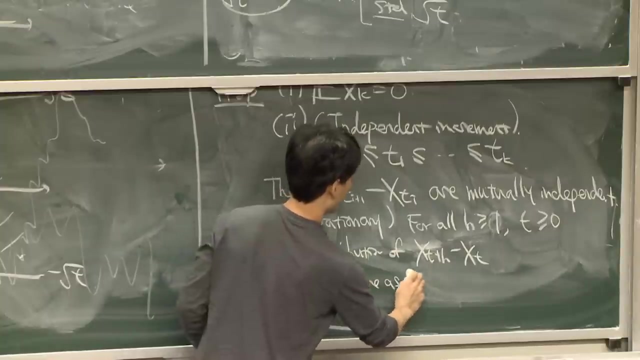 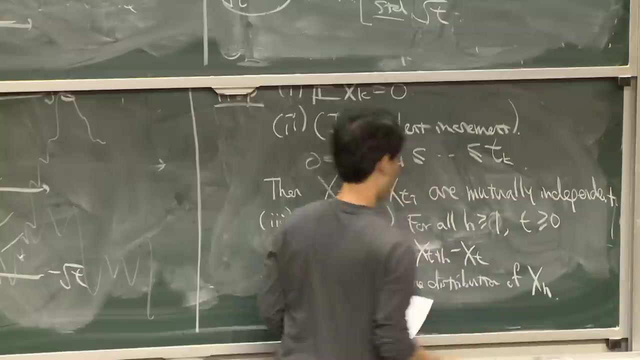 So that's a property That means for all h greater than or equal to 0, and t greater than or equal to 0, h equal to 1, the distribution of xt plus h minus xt is the same as the distribution of x of h. 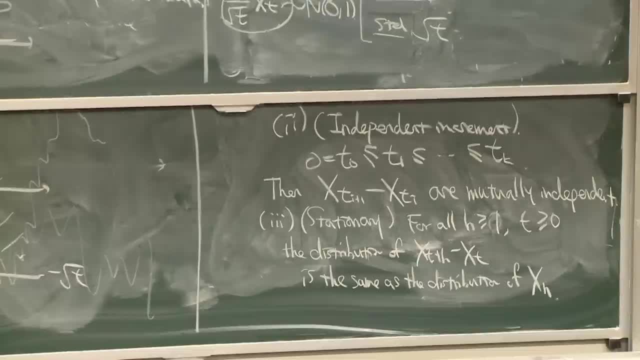 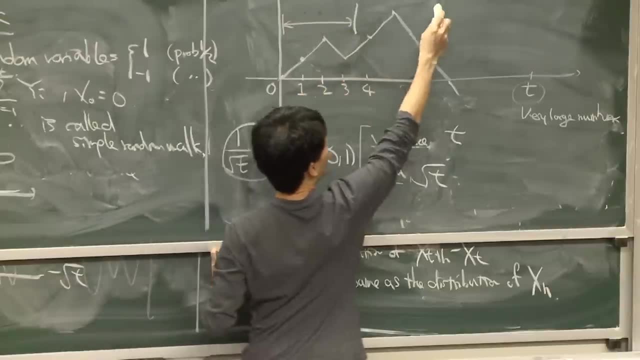 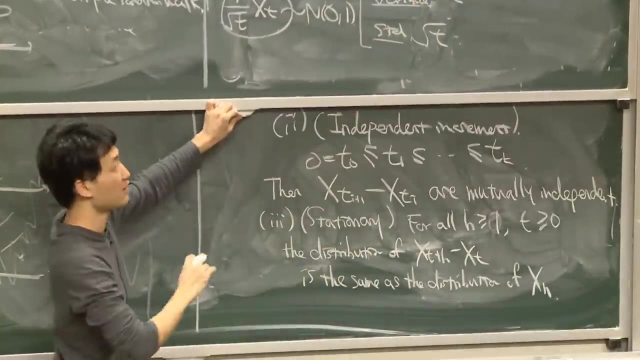 And again, this easily follows from the definition. What it says is: if you look at the same amount of time, then what happens inside this interval is irrelevant of your starting point. The distribution is the same And, moreover, from first part, if these intervals do not, 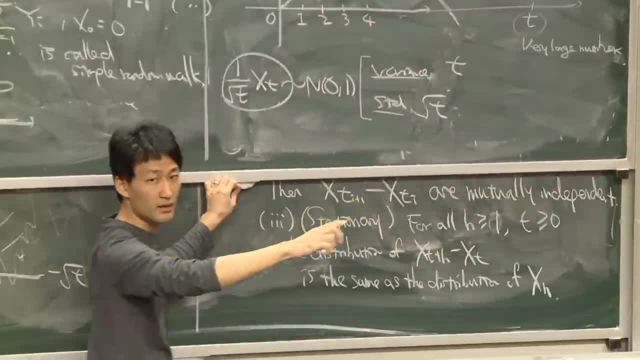 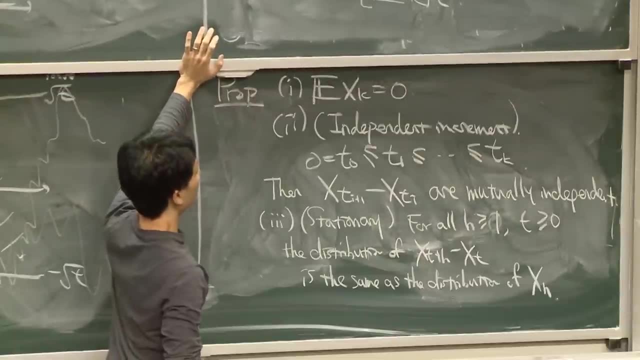 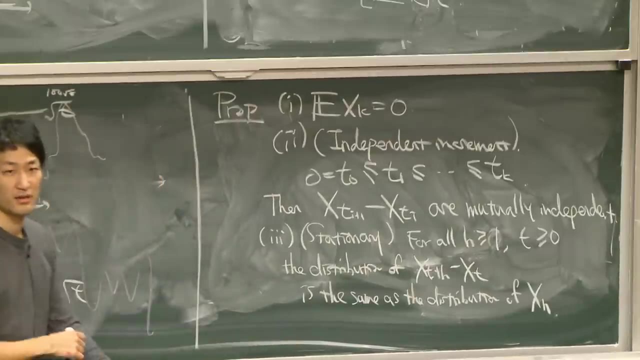 overlap, they're independent. So those are the two properties that we're talking here, And you'll see these properties appearing again and again, because these stochastic processes having these properties are really good. in some sense, They are fundamental, They're stochastic processes. 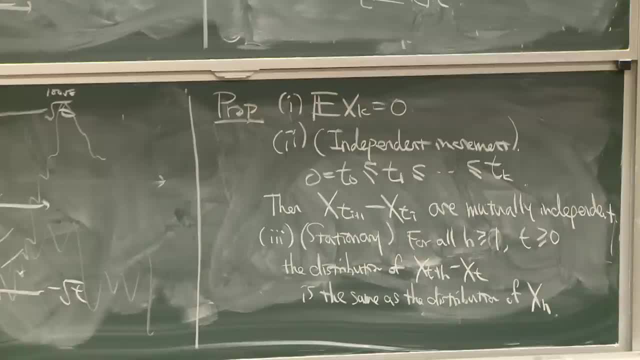 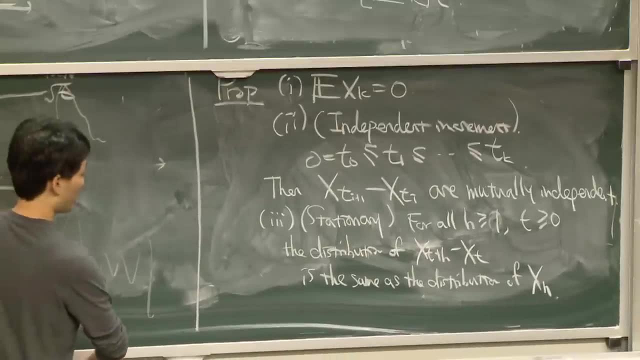 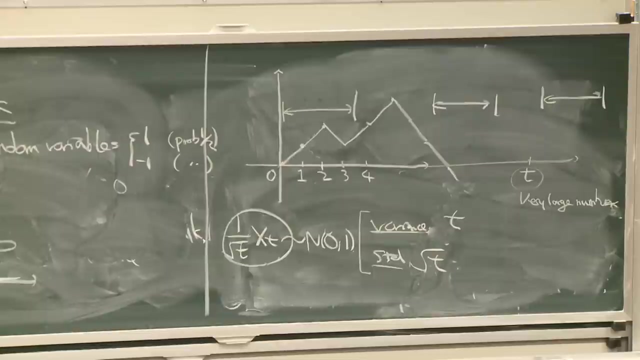 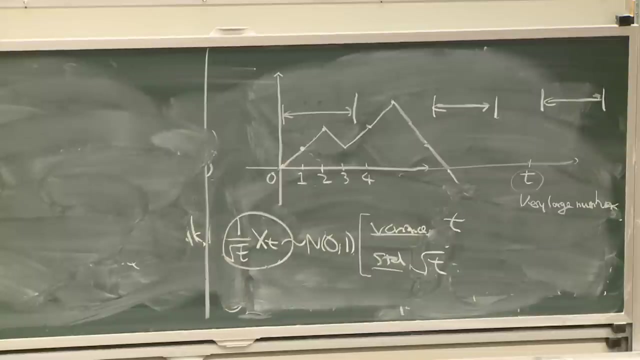 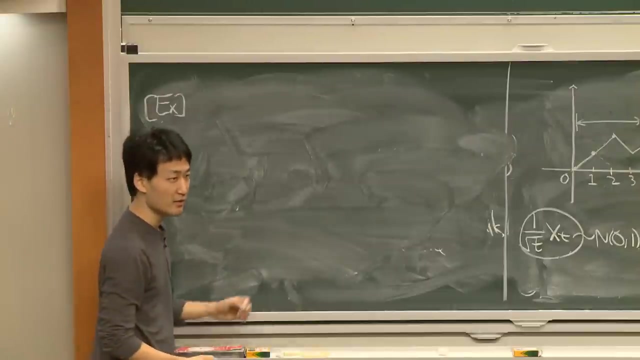 And simple random walk is the fundamental stochastic process. So let's try to see one interesting problem about simple random walk. So example: You play a game. It's like a coin toss. It's a coin toss game I play with, let's say, Peter. 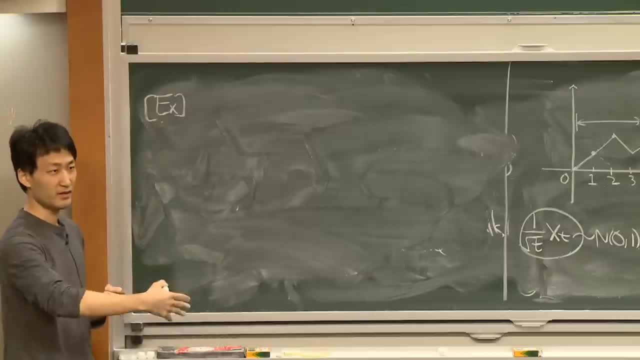 So I bet $1 at each turn, And then Peter tosses a coin, a fair coin. It's either head or tail. If it's head, he wins, He wins the $1.. If it's tail, I win. I win $1.. 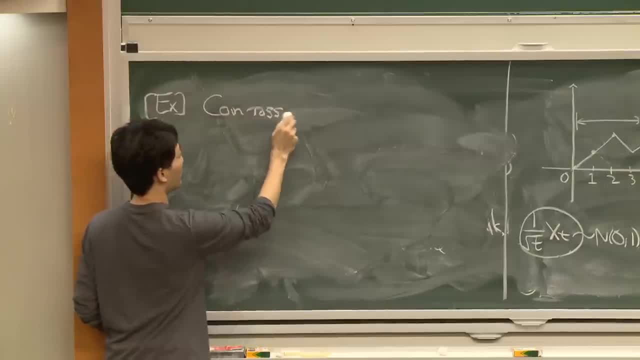 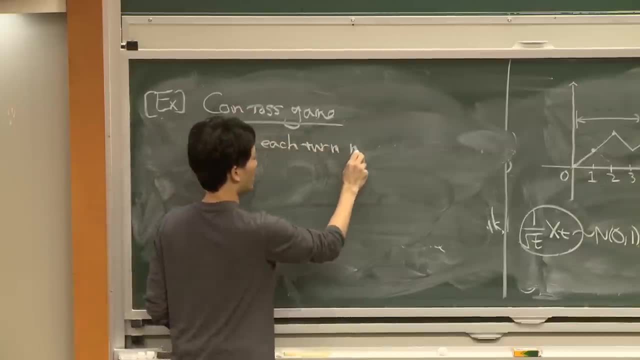 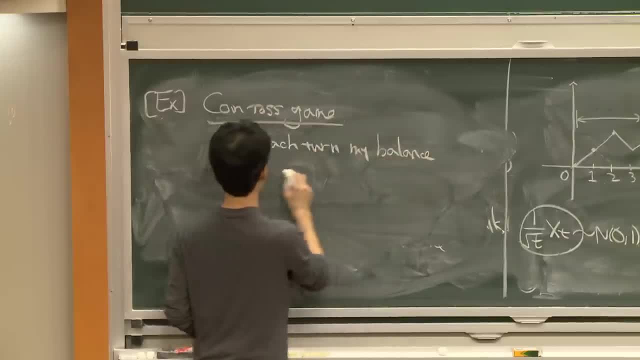 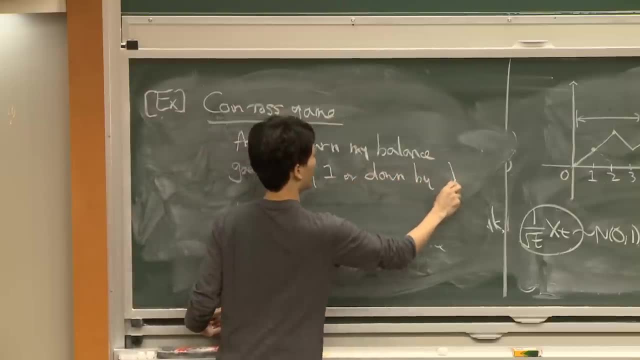 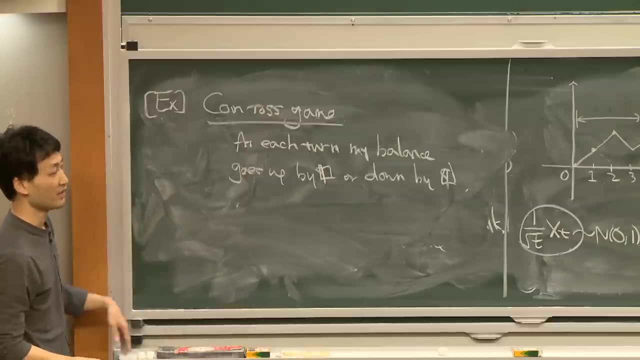 My balance goes up by 1 or down by $1. And now let's say I started from $0 balance, even though that's not possible, Then my balance will exactly follow the simple random walk. assuming that the coin is fairly so, it's a fair coin. 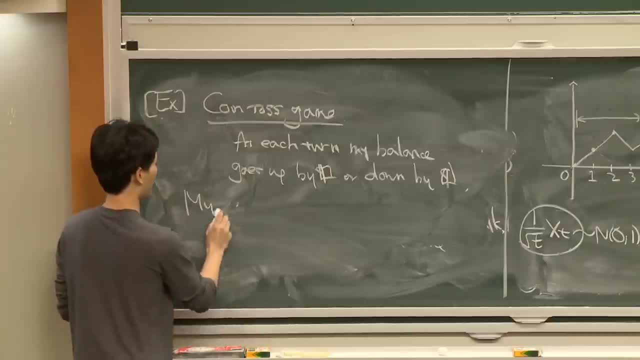 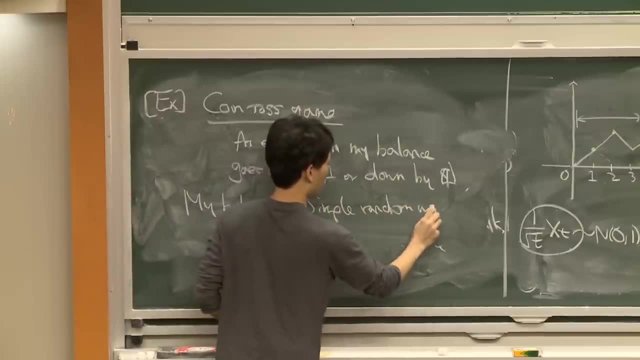 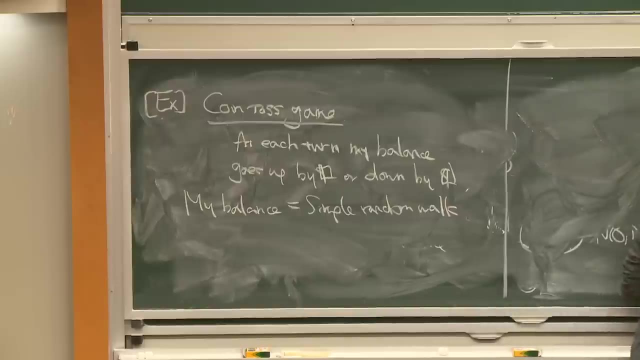 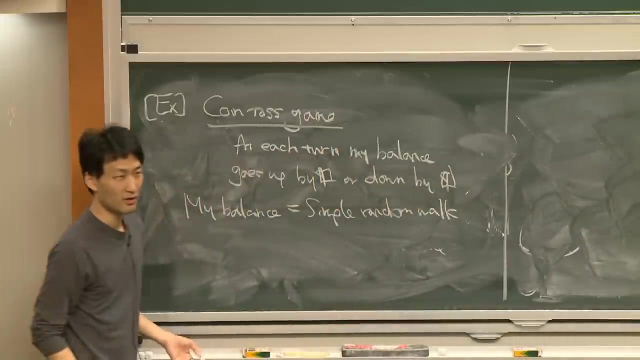 50-50 chance. Then my balance is a simple random walk. And then I say the following: You know what I'm going to play? I want to make money, So I'm going to play until I win $100 or I lose $100. 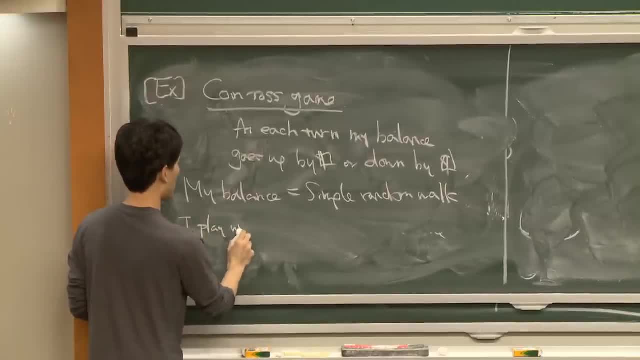 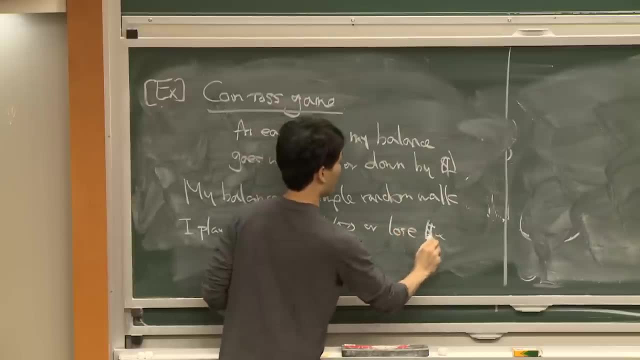 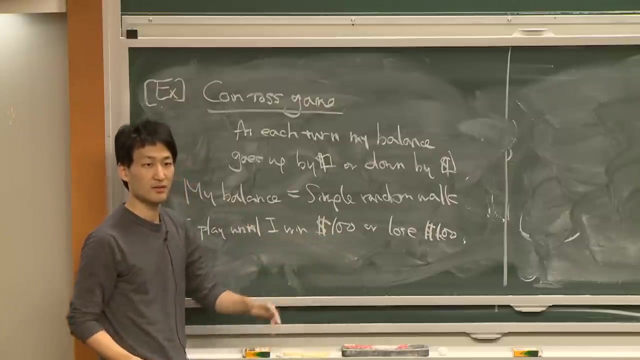 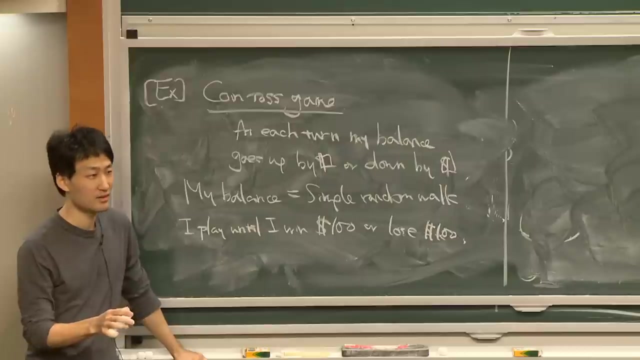 So let's say I play. I'm going to play until I win $100 or I lose $100. What is the probability that I will stop after winning $100? 1 1⁄2. Because Yes, So it happens with 1 1⁄2.. 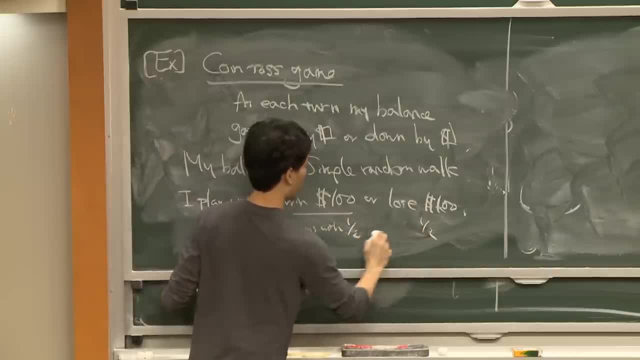 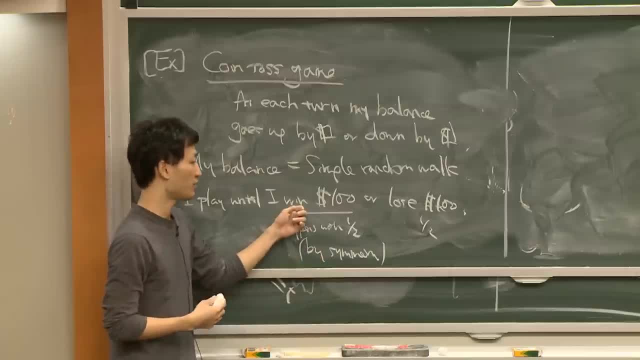 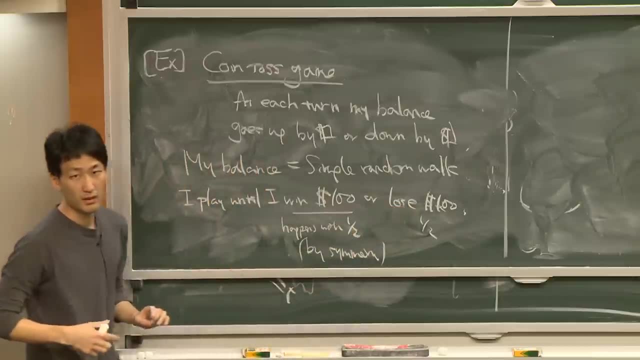 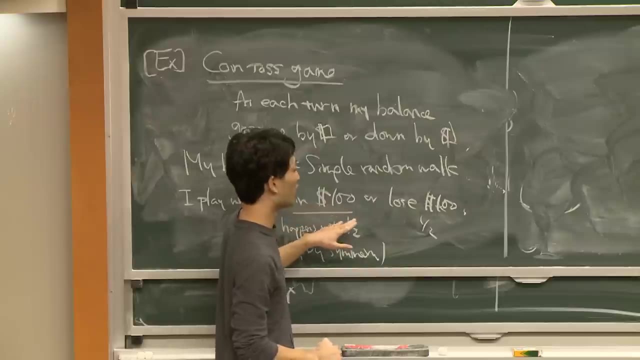 Because every chain of coin toss which gives a winning sequence, when you flip it, it will give a losing sequence. So you have a one-to-one correspondence between those two things. That was good. Now, if I change it, what if I say I win $100 or I lose $50?? 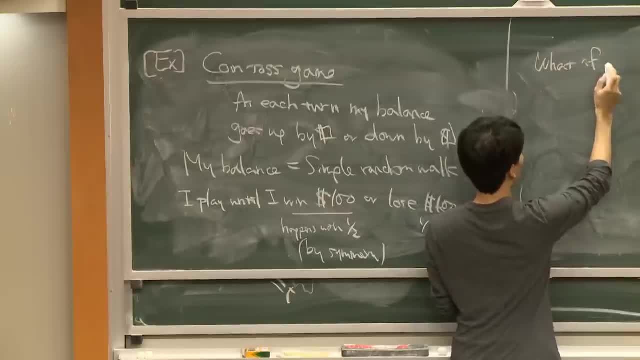 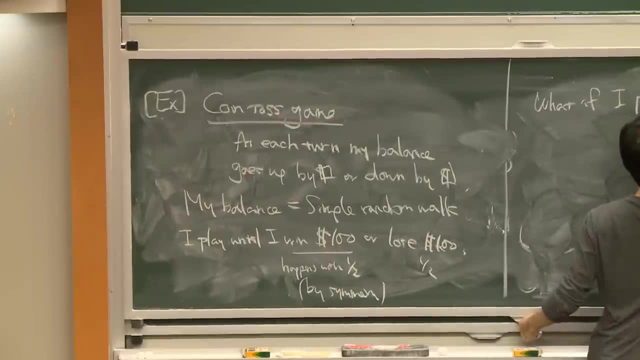 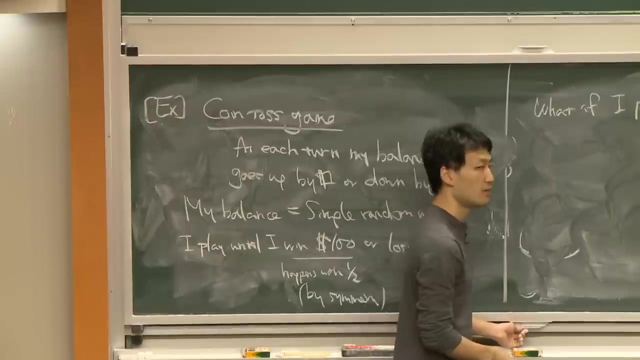 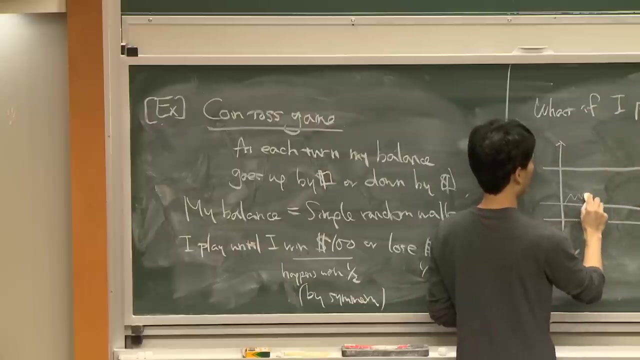 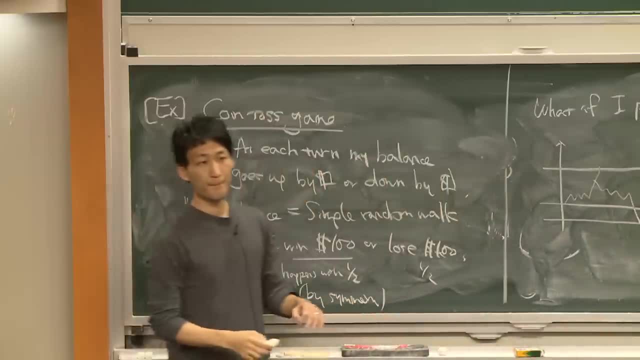 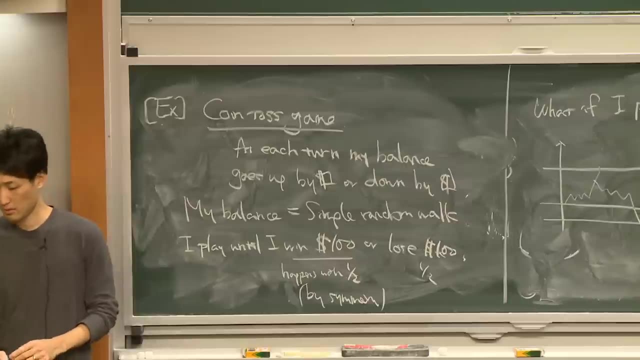 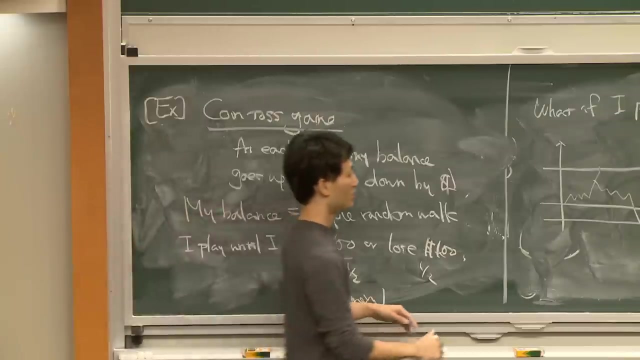 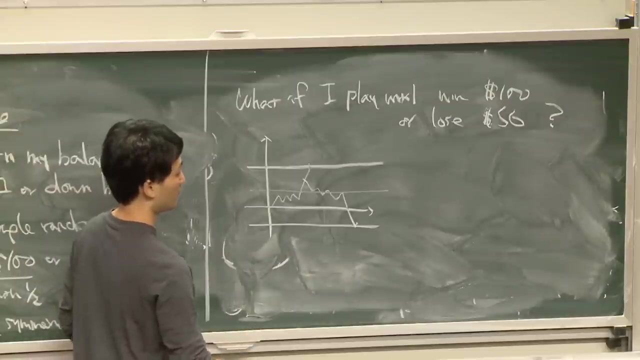 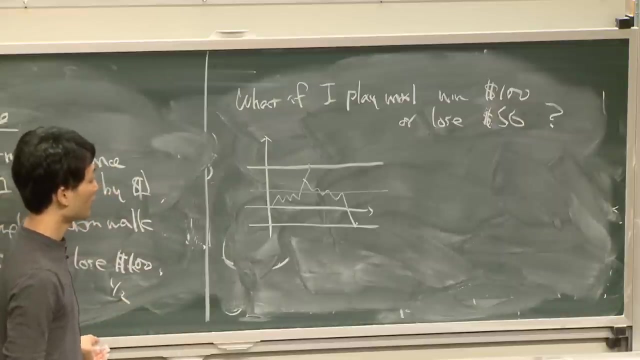 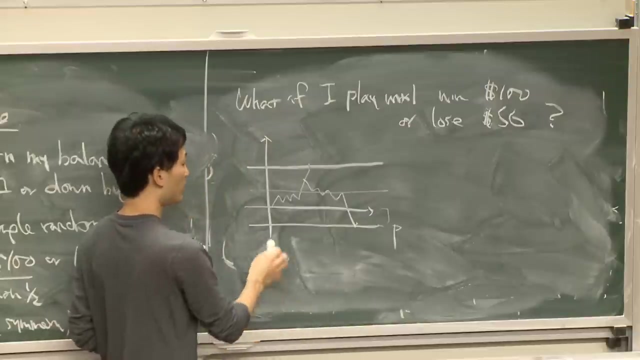 or it hits this line And then I stop. What is the probability that I will stop? stop after winning $100 one-third. can you see why? one-third? okay, so you're saying. you're saying So hitting this probability is P And the probability 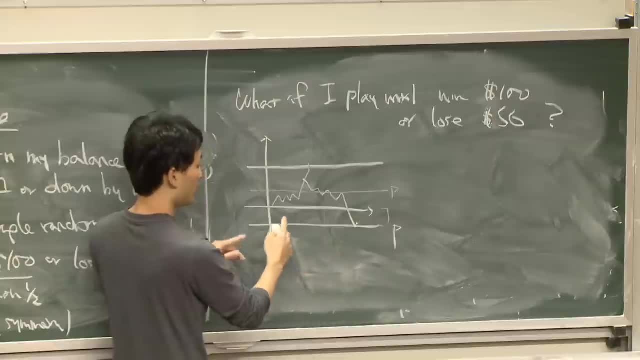 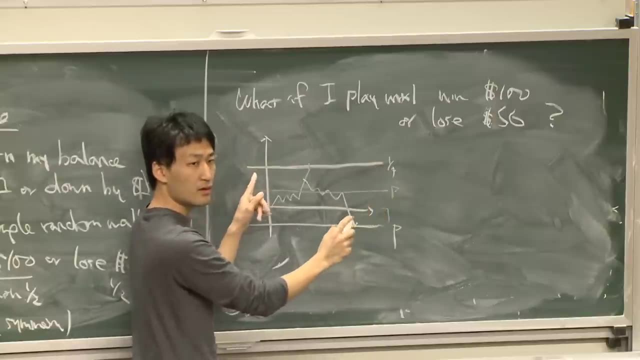 that you hit this first is P. This is 1 half, 1 half. What you're saying from here is the same, So it should be 1 fourth here: 1 over 2 times 1 over 2.. And you had a good intuition. 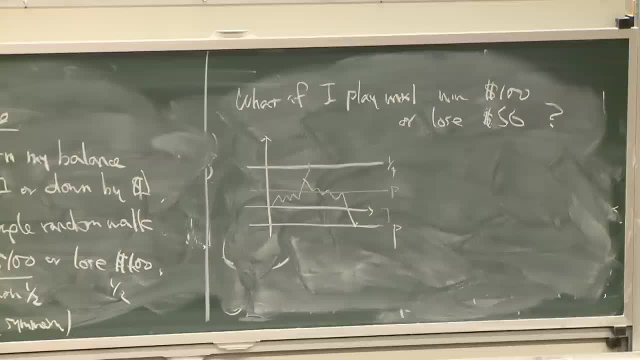 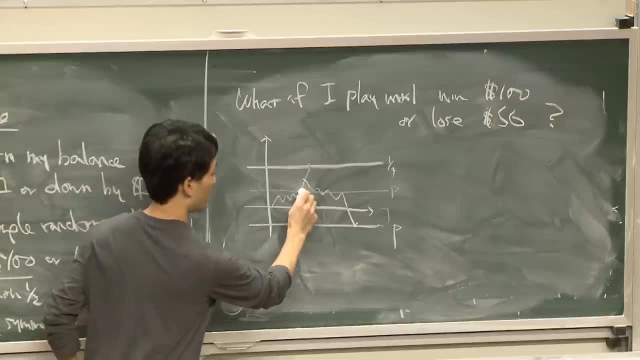 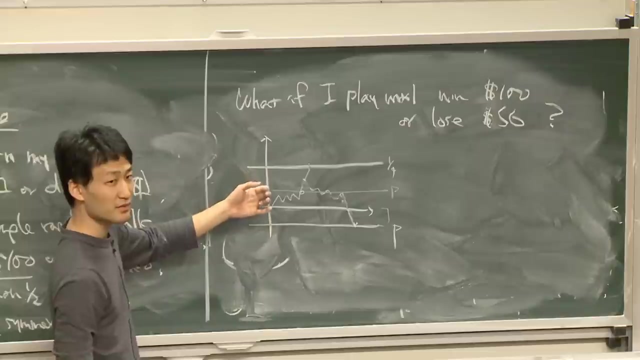 It is 1 over 3, actually I was wondering if, instead of all 2, you could add intersect 50. And then, once you hit it, it's like the same afterwards. I'm not sure if there's a way to make an argument out of it. 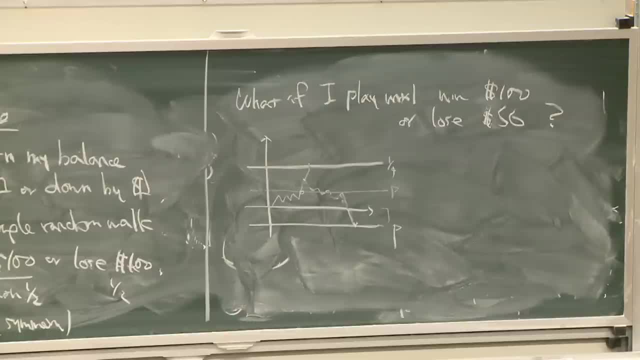 I really don't know. There might be or there might not be, I'm not sure. I was thinking of a different way. But yeah, there might be a way to make an argument out of it. I just don't see it right now. 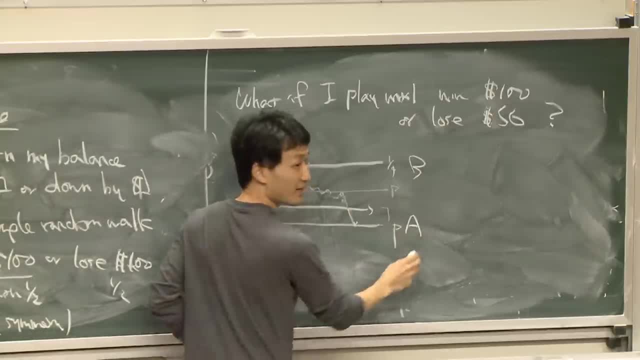 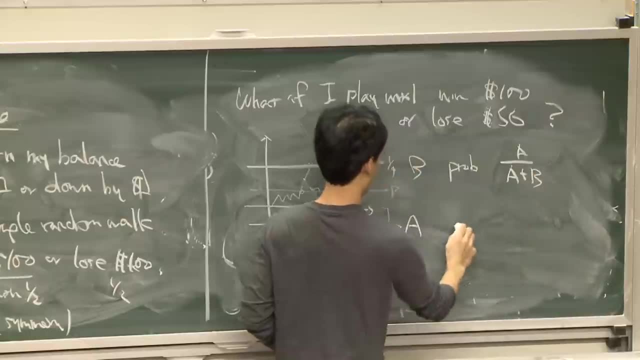 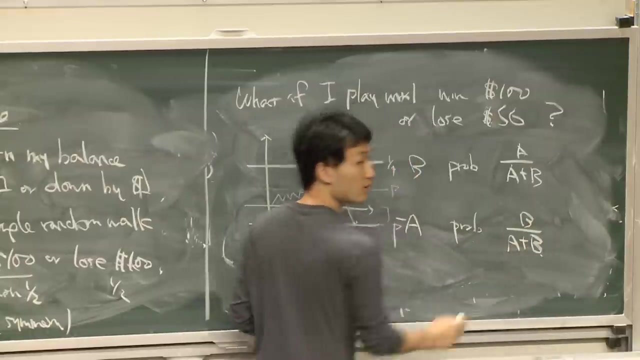 So in general, if you put a line B and a line A, then probability of hitting B first is A over A plus B, And probability of hitting this line minus A, It's B over A plus B. So in this case, if it's 150, it's 100 over 150. 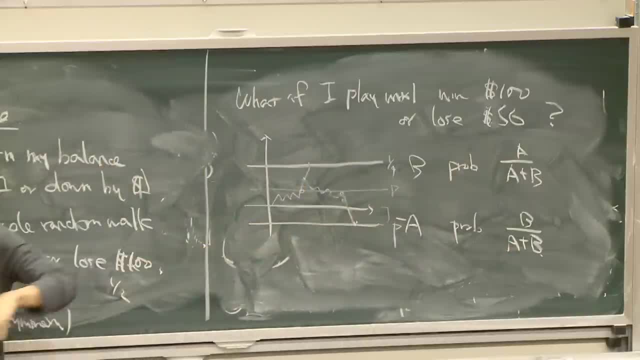 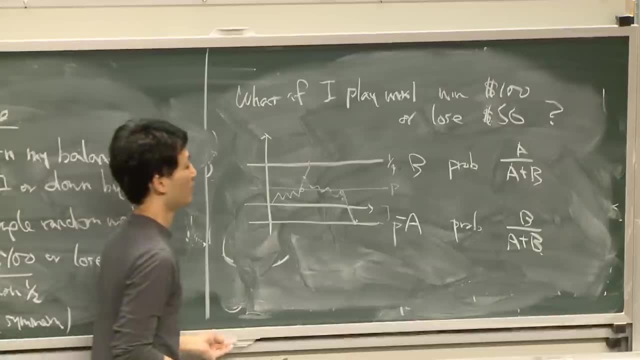 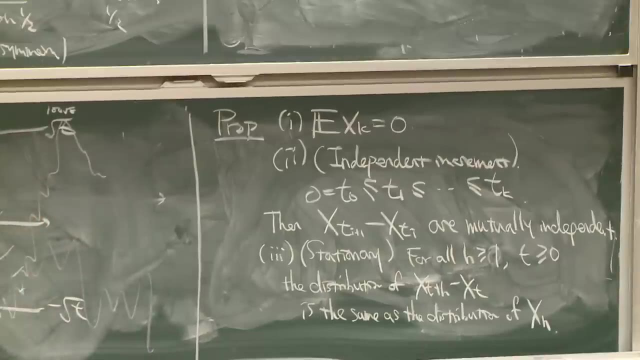 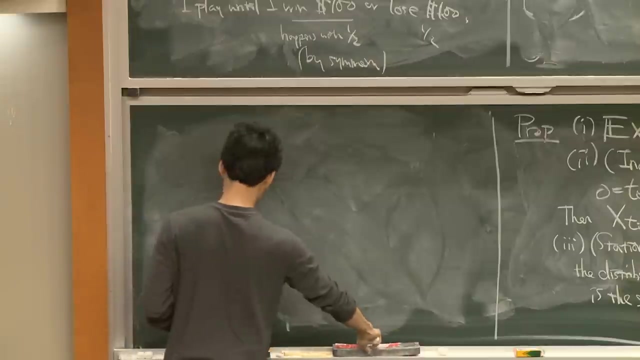 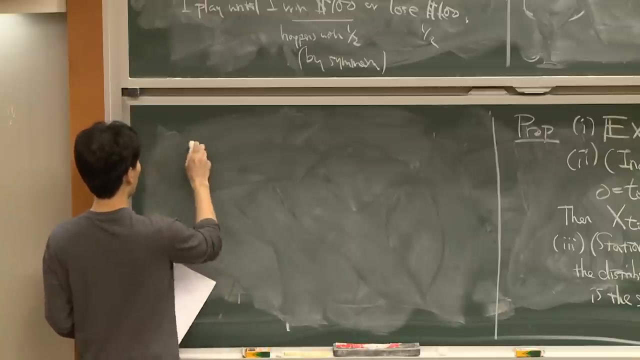 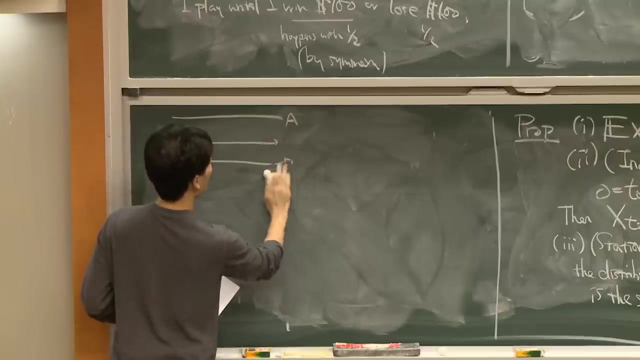 That's 2 thirds And that's 1 third. This can be proved. It's actually not that difficult to prove it. I mean it's hard to find the right way to look at it. So fix your A, a, B and A. 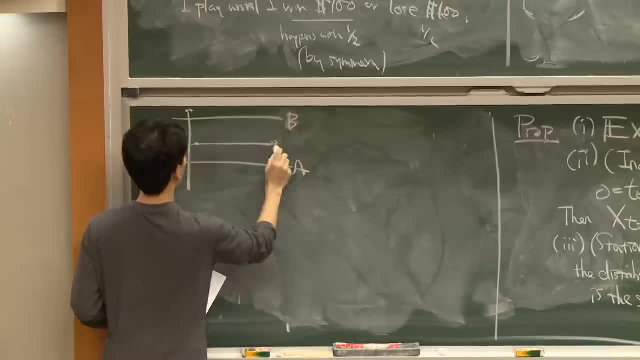 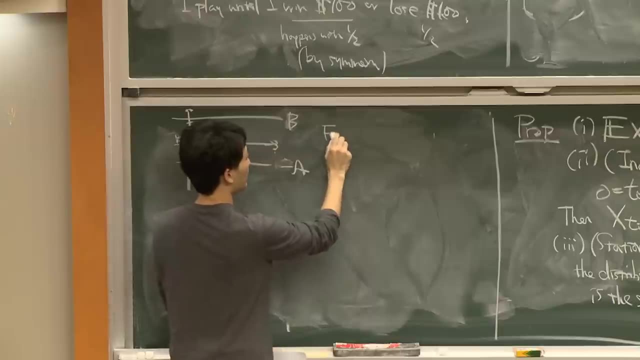 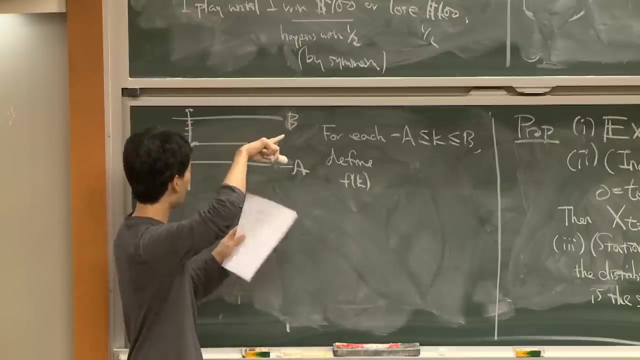 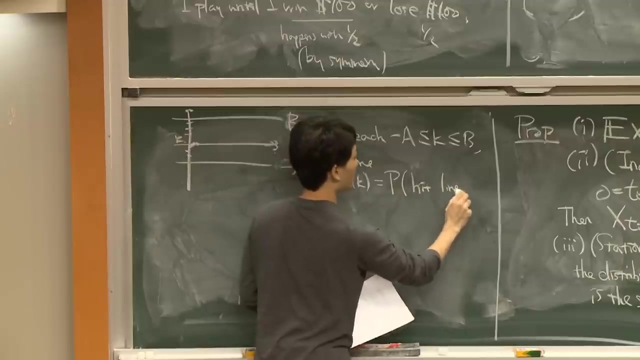 And for each k between A minus A and B, define f of k as the probability that you will hit this line first As the probability that you hit this line first. And for each k between A minus A and B, you hit the line B first when you start at k. 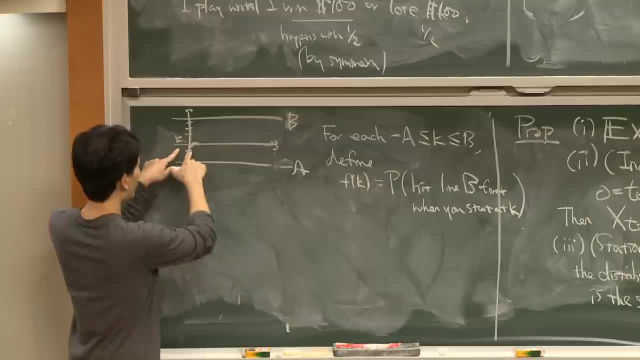 So it kind of points out what you're saying. Now, instead of looking at one fixed starting point, we're going to change our starting points and look at all possible ways. So when you start at k, I will define f of k as the probability that you hit this line first. 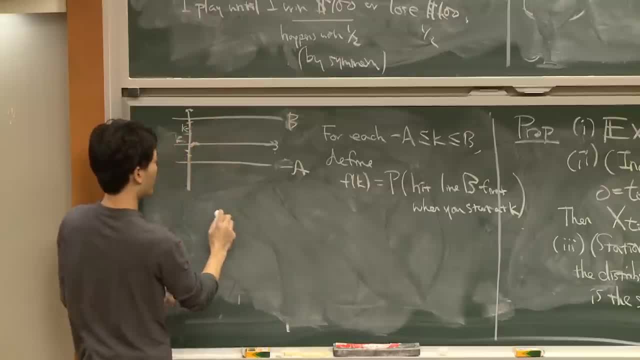 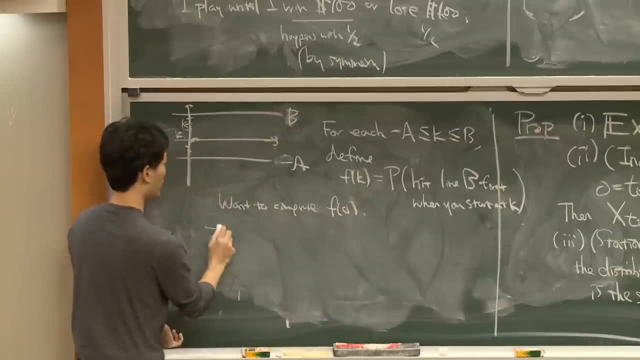 before hitting that line: OK, What we're interested in is want to compute f0?. What we know is: f of B is equal to 1.. f of minus A is equal to 0.. No, And then we'll formula. 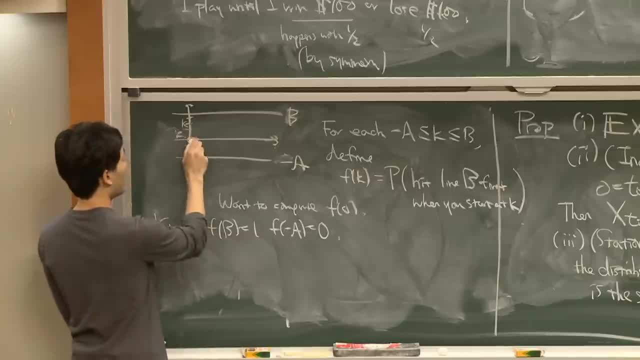 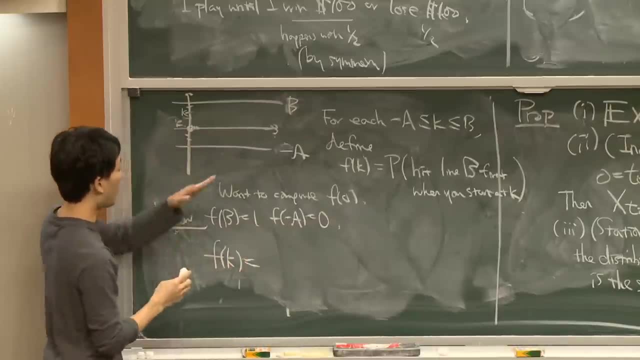 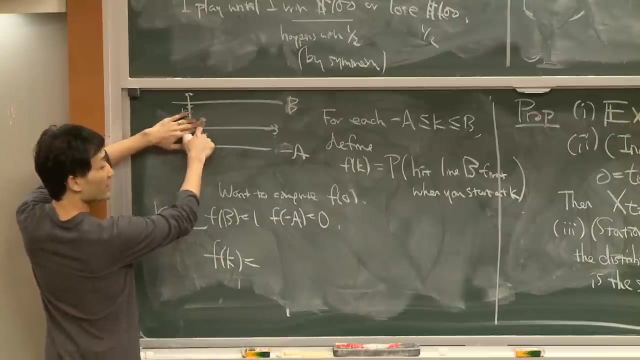 Actually, there is one recursive formula. that matters to us is if you start at fk. But if you start at fk, you either go up or go down. You go up with probability one half, You go down with probability one half, And now it starts again because of this stationary property. 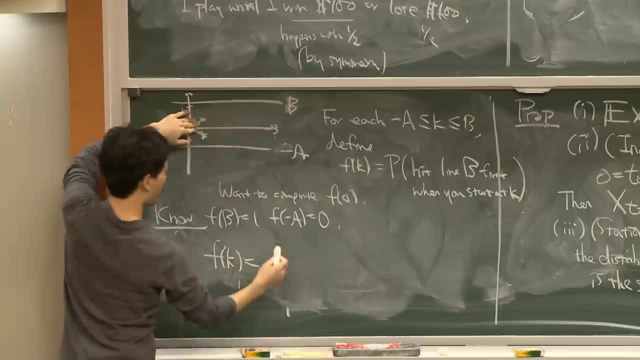 So, starting from here, the probability that you hit B first is exactly f of k plus one. So if you go up, the probability that you hit B first will be one half first is f of k plus 1.. If you go down, it's f of k minus 1.. 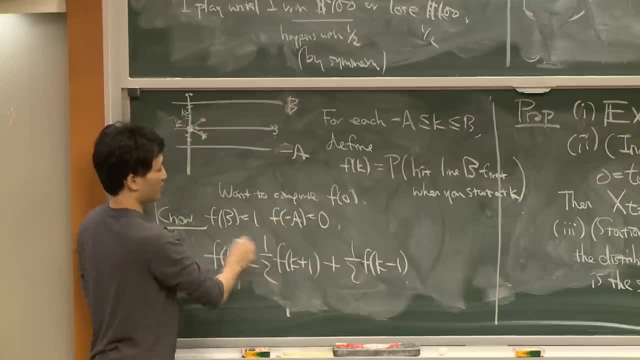 And then that gives you a recursive formula with two boundary values. If you look at it, you can solve it. When you solve it, you'll get that answer. So I won't go into detail, but what I wanted to show is that simple, random walk is really. 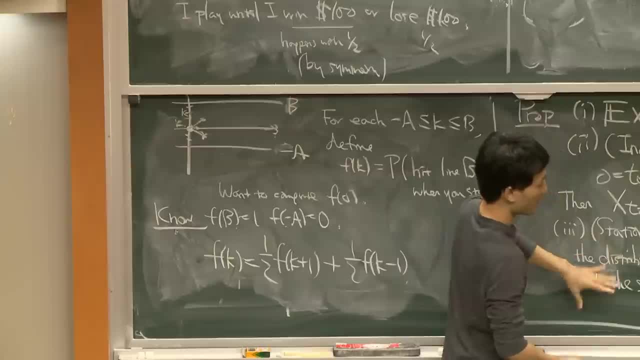 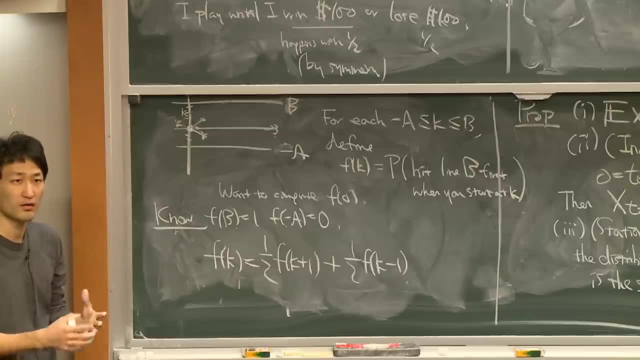 this property, these two properties have these properties and even more powerful properties. So it's really easy to control And at the same time it's quite universal. It can model something. It's not a very weak model, It's rather restricted, but it's a really good model. 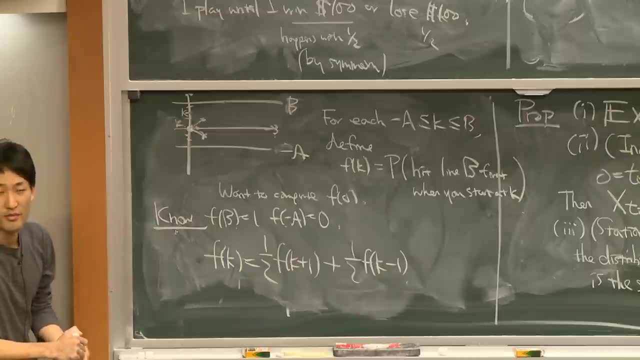 for a mathematician. From the practical point of view you'll have to twist some things slightly and so on. But I mean, In many cases you can approximate it by simple random walk And as you can see the computations, you can do computations with simple random walk by hand. 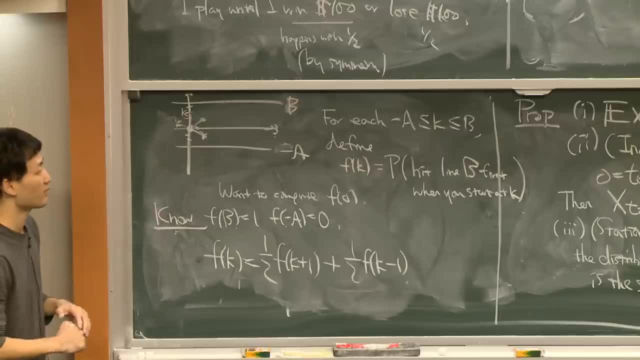 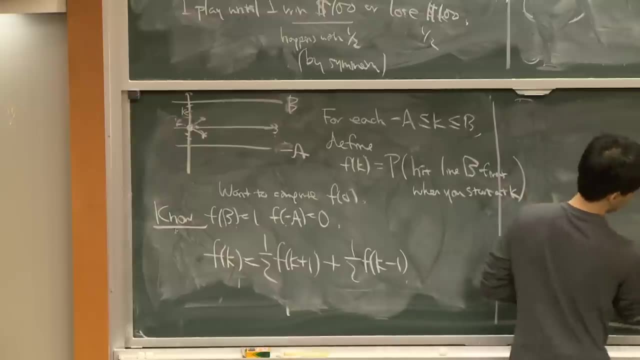 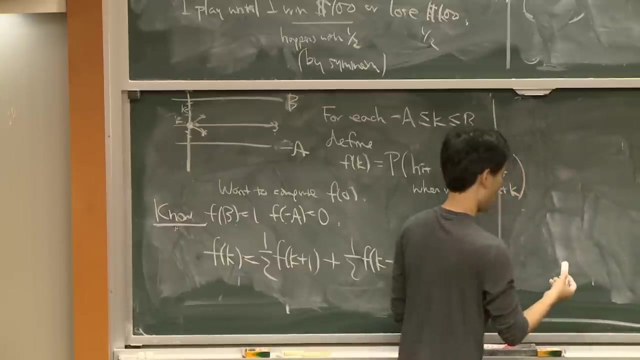 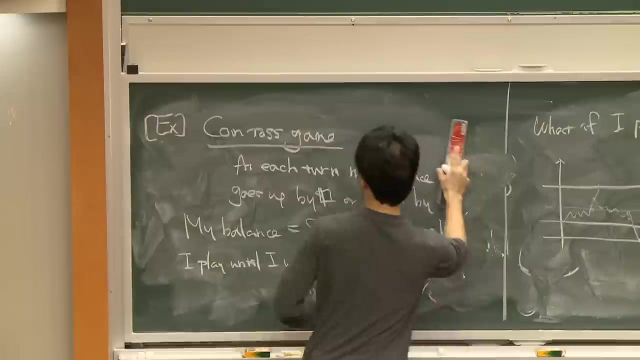 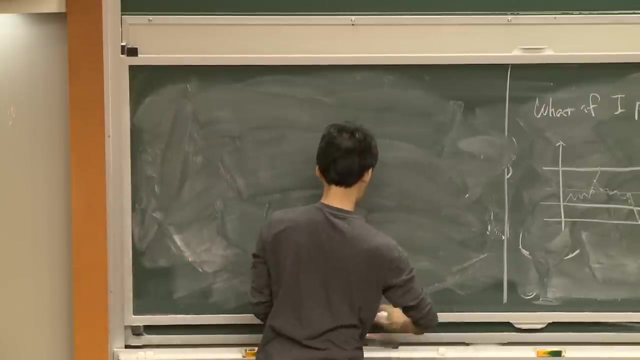 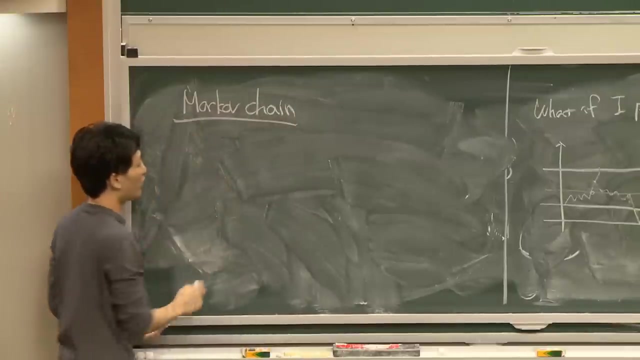 That was it. I talked about the most important example of stochastic process. Now let's talk about more stochastic processes. The second one is called the Markov chain. Let me erase that part. actually, The Markov chain, unlike the simple random walk, 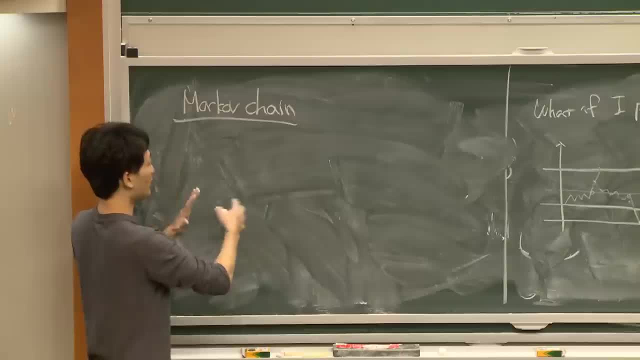 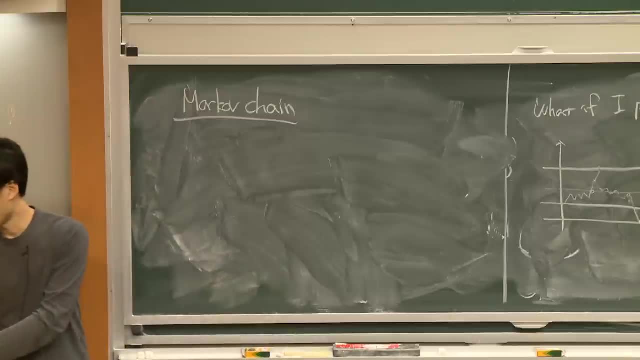 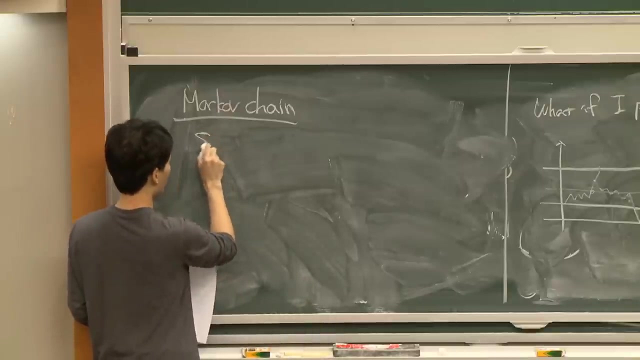 is not a single stochastic process. It's not a single stochastic process. It's a collection. It's a stochastic process. It's called a Markov chain if it has some property. And what we want to capture in Markov chain is the following statement: 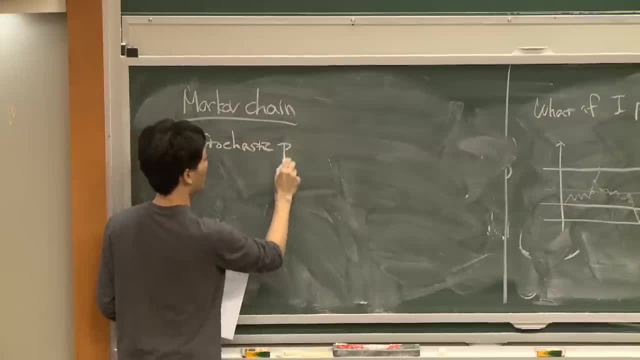 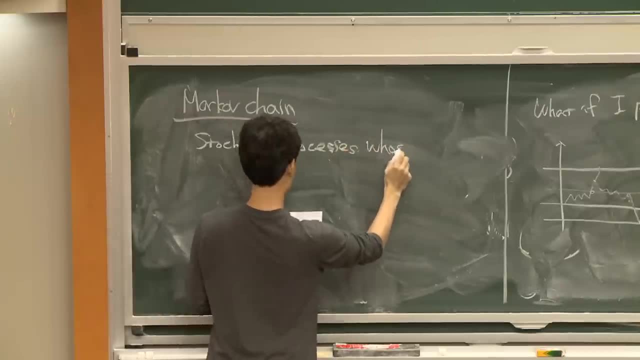 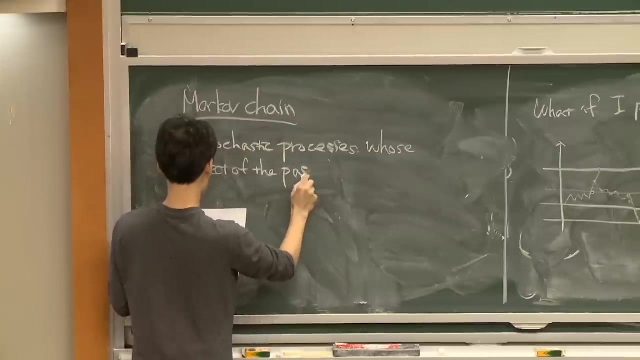 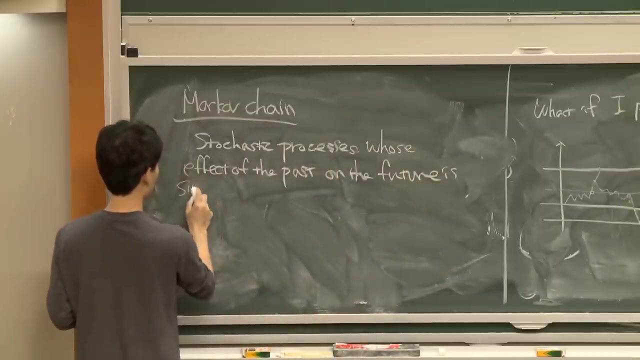 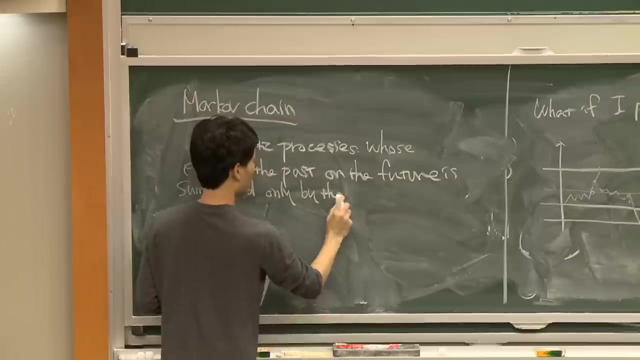 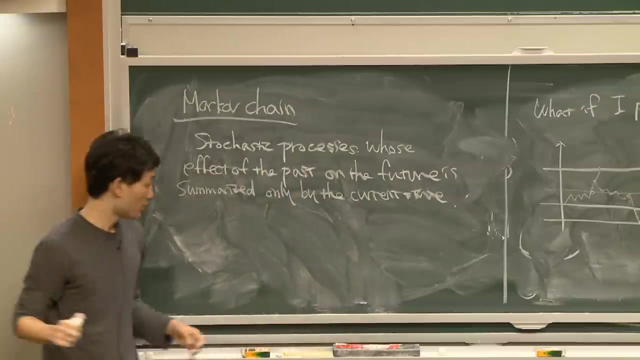 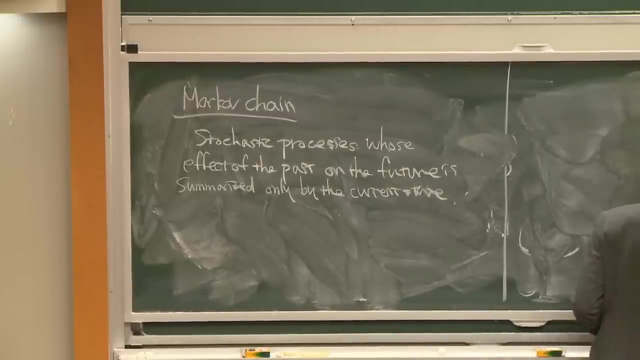 These are a collection of stochastic processes having the property that whose effect of the past On the future is summarized only by the current state. That's quite a vague statement. What we're trying to capture here is: let's look at some generic stochastic process at time t. 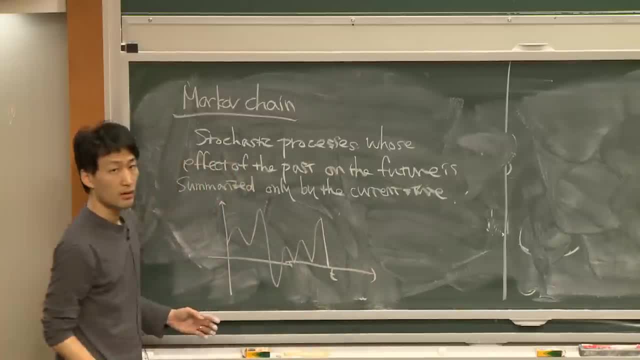 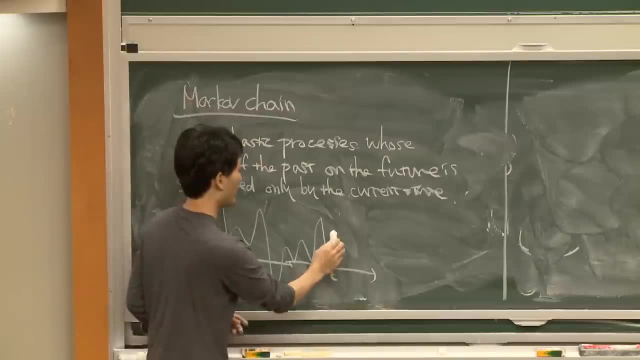 Now look at some generic stochastic process. at time t, You know all the history up to time t. You want to say something about the future? Then if it's a Markov chain, what it's saying is: you don't even have to know all about it. 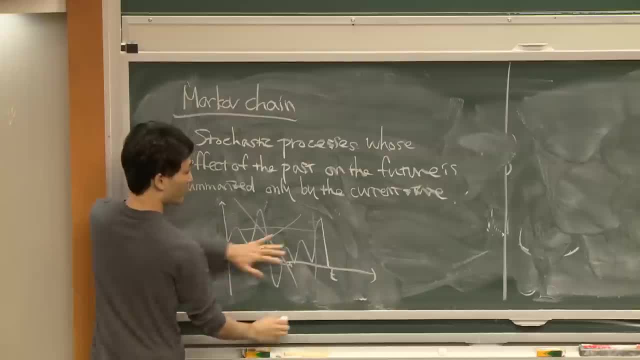 Like. this part is really irrelevant. What matters is the value at this last point, The value at this last point last time. If it's a Markov chain, you don't have to know all this history. All you have to know is this single value. 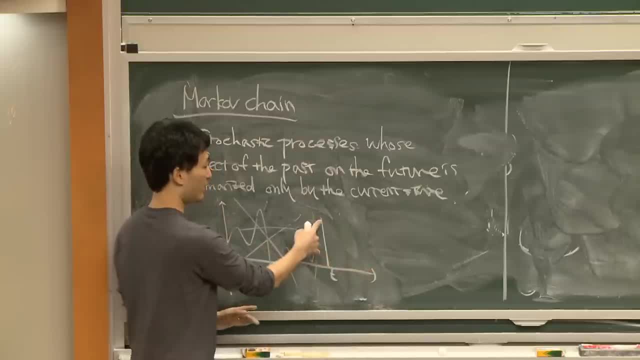 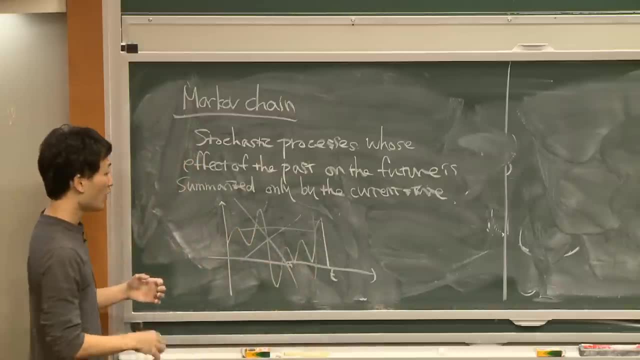 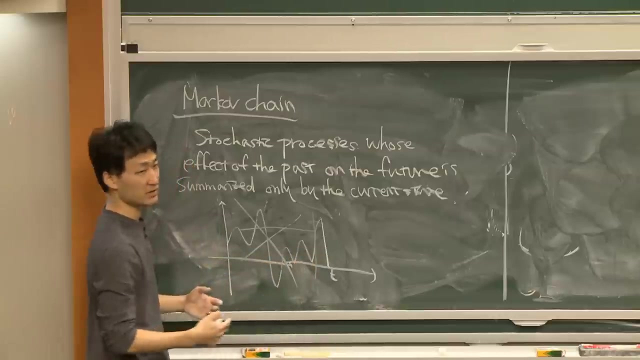 And all the effect of the past and the future is contained in this value. No, nothing else matters. Of course, this is a very special type of stochastic process. Most of the stochastic processes, the future will depend on the whole history, And in that case it's more difficult to analyze. 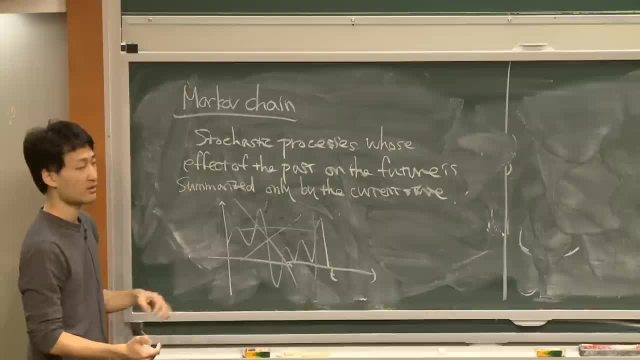 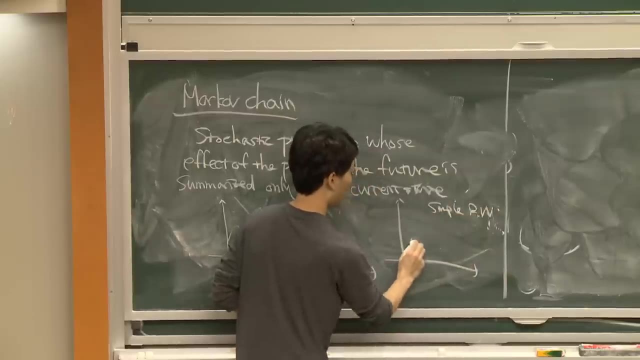 But these are very special Because these ones are more manageable And still lots of interesting things turn out to be Markov chains. So if you look at simple random walk, it is a Markov chain. Simple random walk. Let's say you went like that. 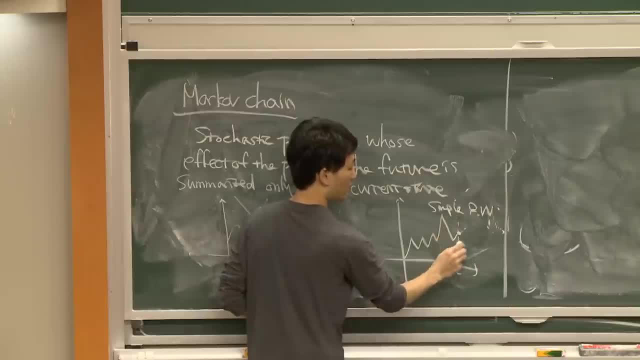 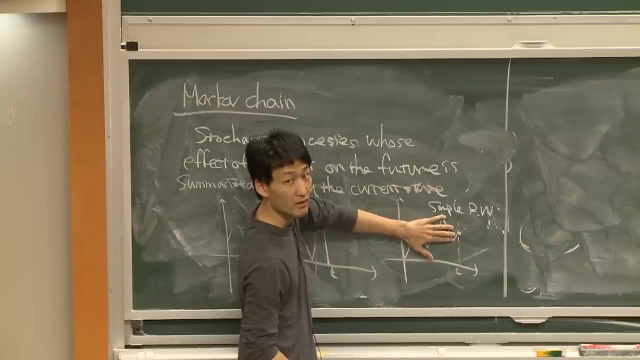 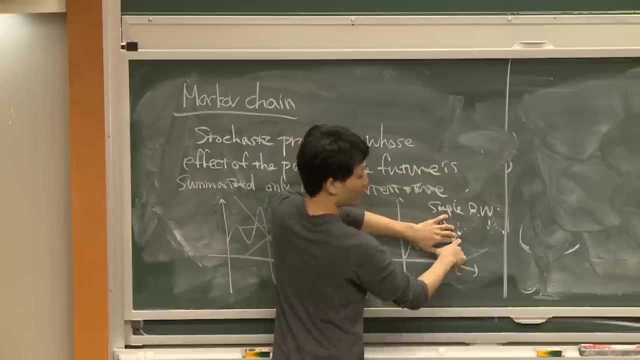 Then what happens after time? t really just depends on how high this point is at. What happened before doesn't matter at all, Because we're just having new coin tosses every time, But this value can affect the future, Because that's where you're going to start your process. 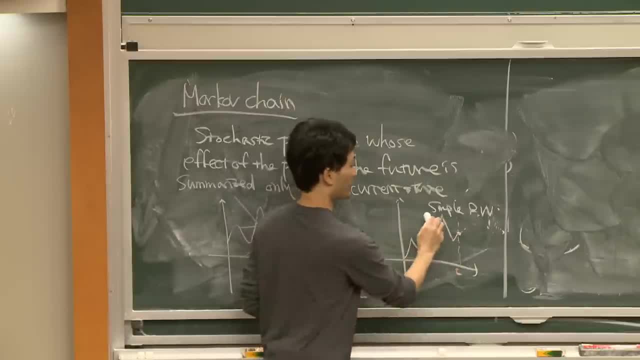 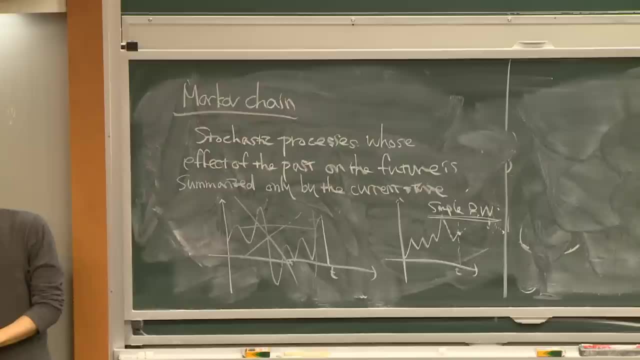 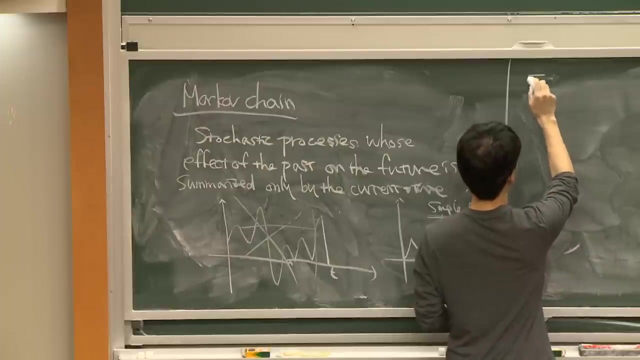 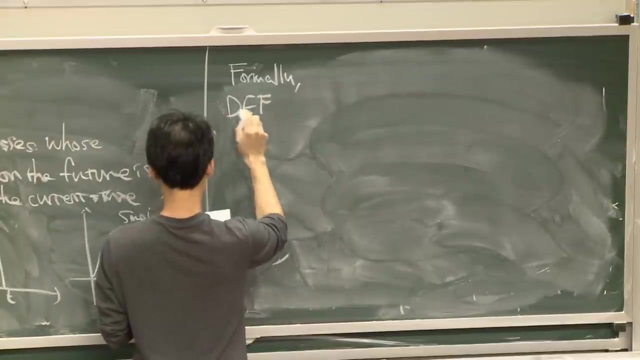 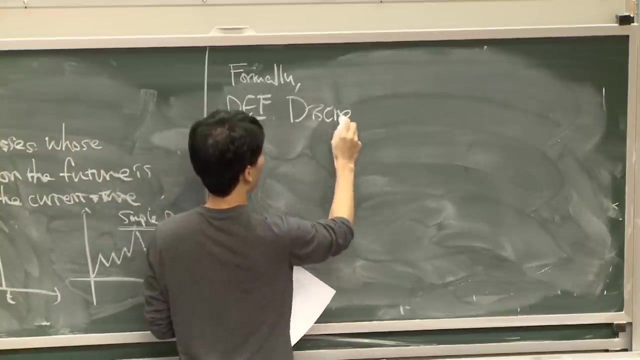 That's where you're starting your process. So that is a Markov chain. This part is irrelevant, Only the value matters. So let me define it a little bit more formally, More formally. So let's figure out what it means when I say: 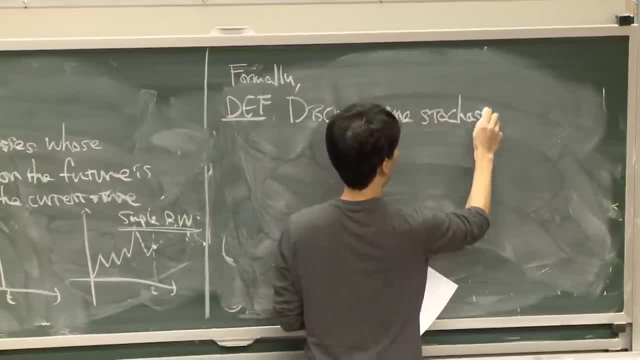 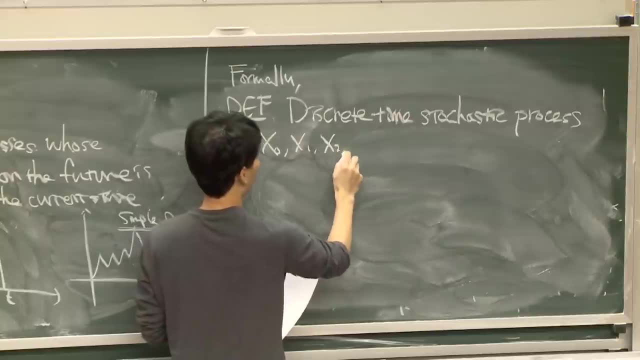 a discrete time. stochastic processing is a Markov chain. Of course we're going to call it what we call trem, partial time t. But while you're working with the demand, this can depend on your Autom проф variety sausage They can vary. 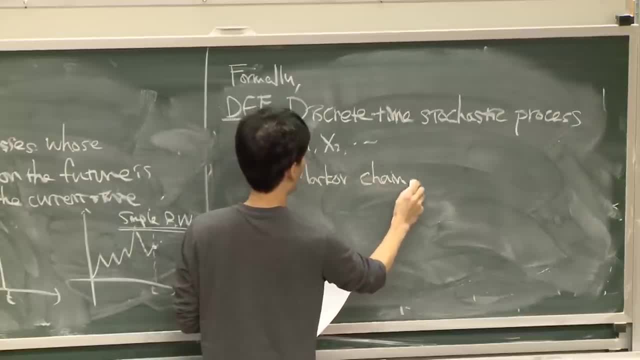 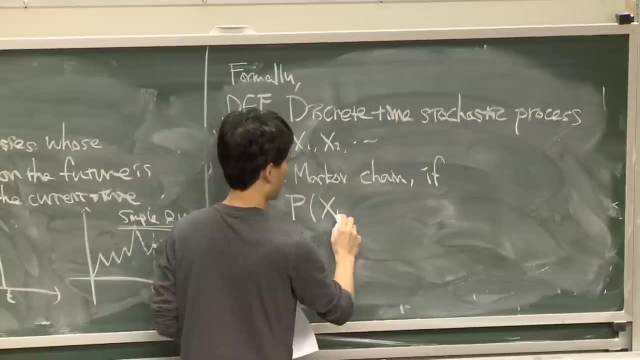 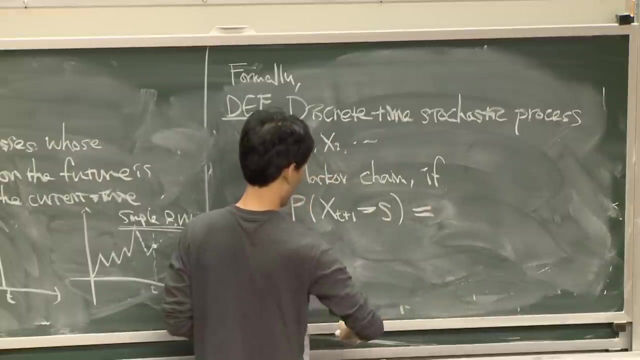 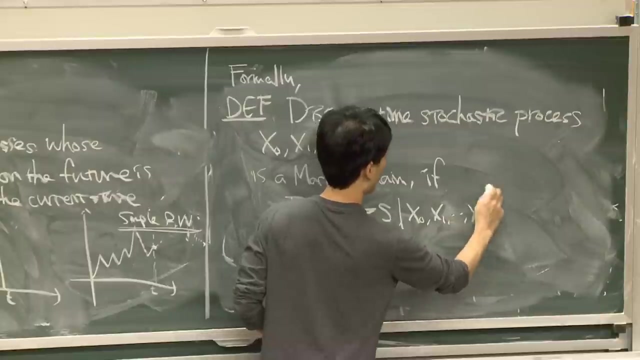 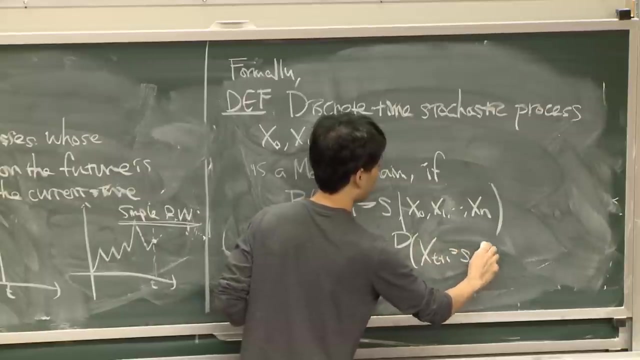 if the probability that x, at some time, t plus 1 is equal to something, some value, given the whole history up to time, n, is equal to the probability that x, t plus 1 is equal to that value, given the value of x of n. 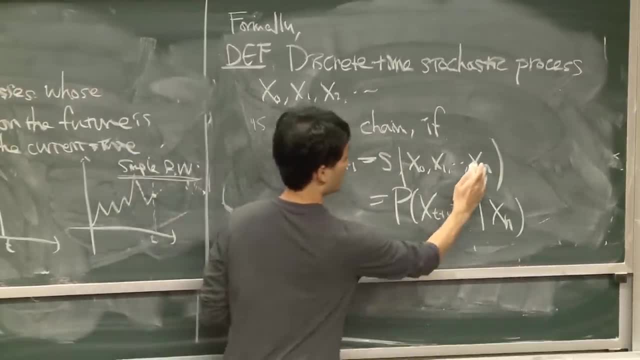 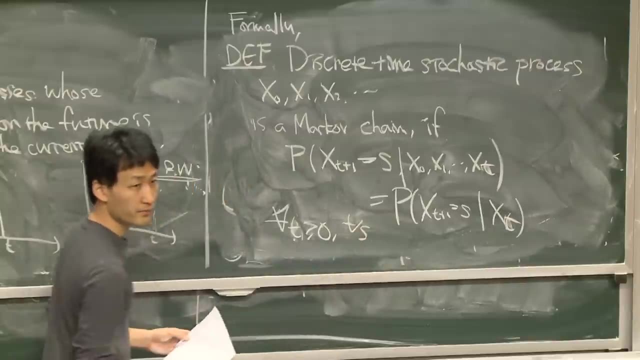 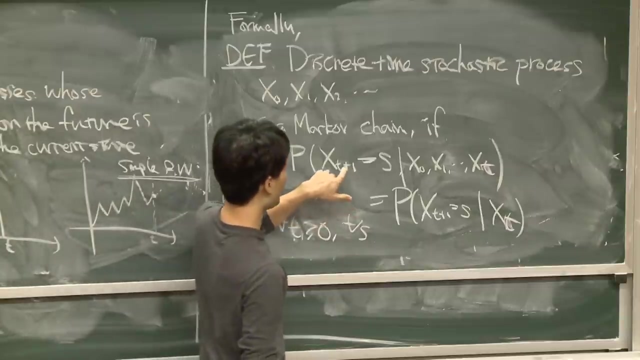 for all n greater than or equal to t greater than or equal to 0, and all s. This is a mathematical way of writing down the value at x, t plus 1. given all the values up to time t, t is the same as the value at time t plus 1,. 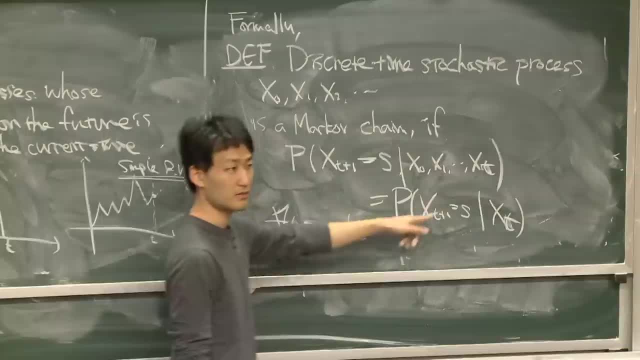 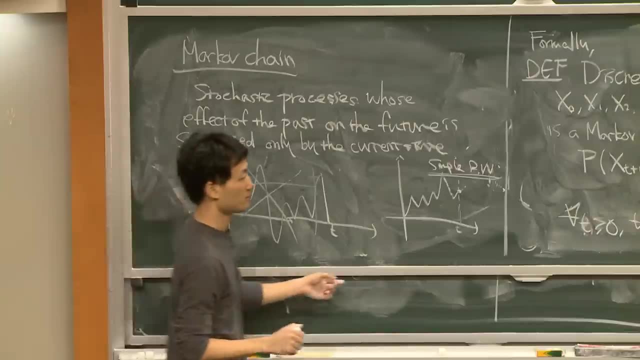 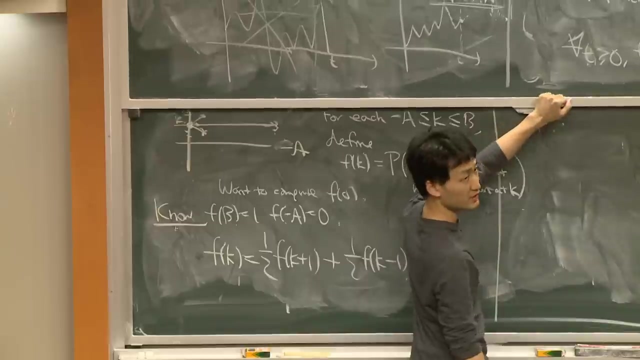 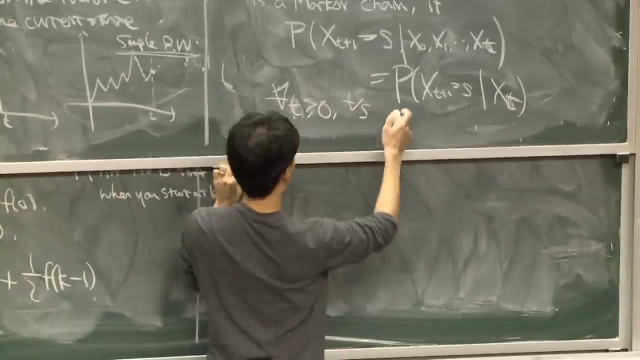 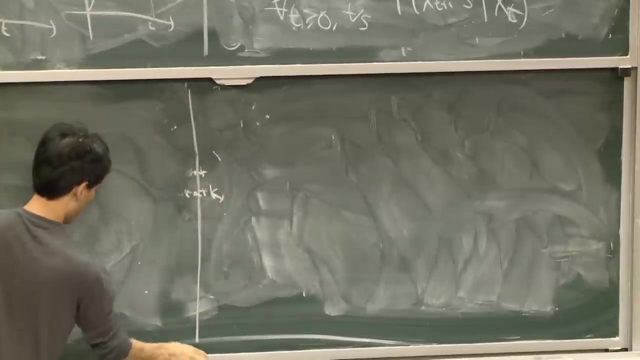 the probability of it, given only the last value. And the reason simple random walk is a Markov chain is because both of them are just 1 half If it's 4.. Let me write it down Why, For example, random walk probability. 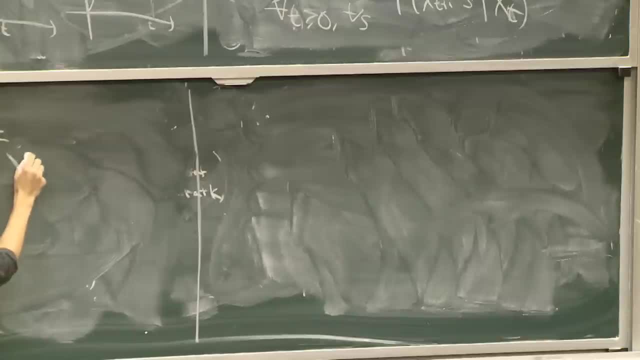 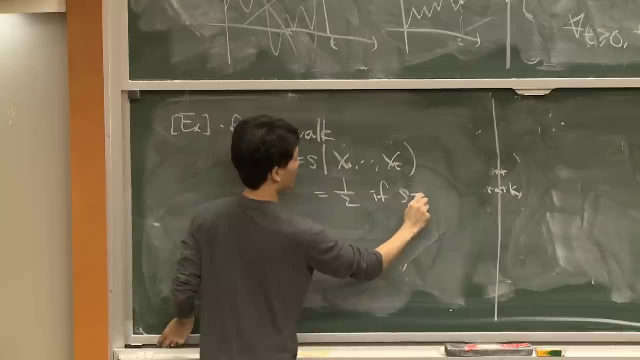 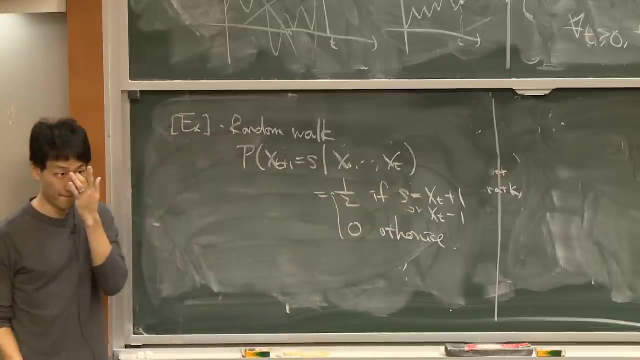 that x t plus 1 plus s, given t is equal to 1 half. If s is equal to x t plus 1, r, x t minus 1, and 0 otherwise. So it really depends only on the last value: x t. 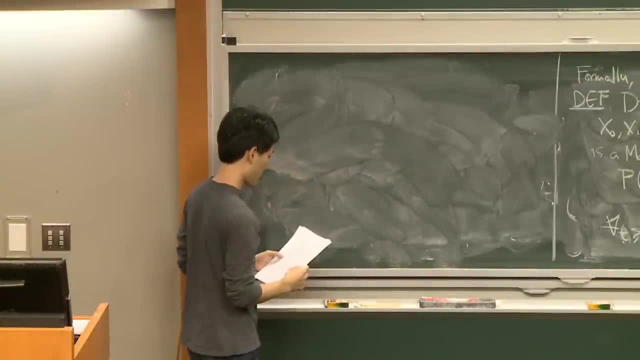 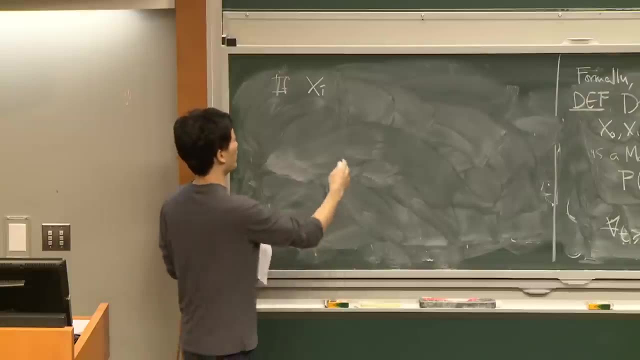 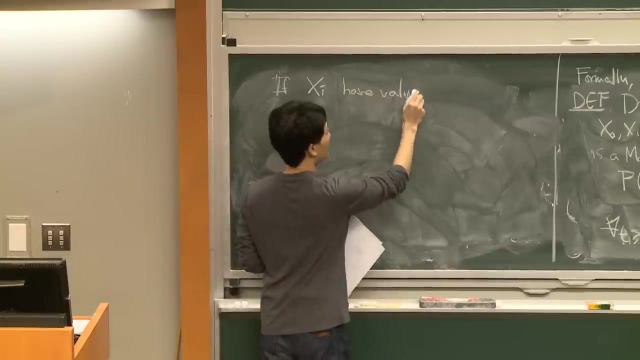 Any questions? All right. So consider the case when all xi's- you're looking at a stochastic process, the Markov chain- and all xi, if xi have values in some set- s, r, s and t, which is finite, a finite thing. 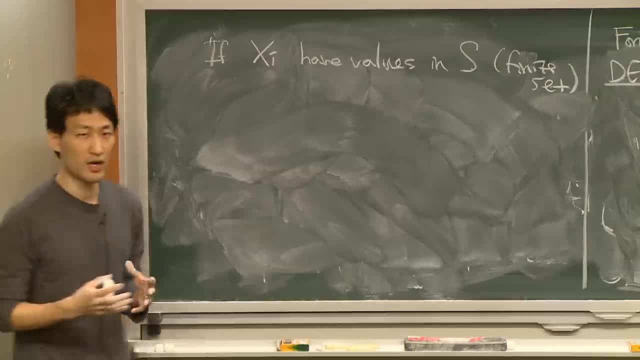 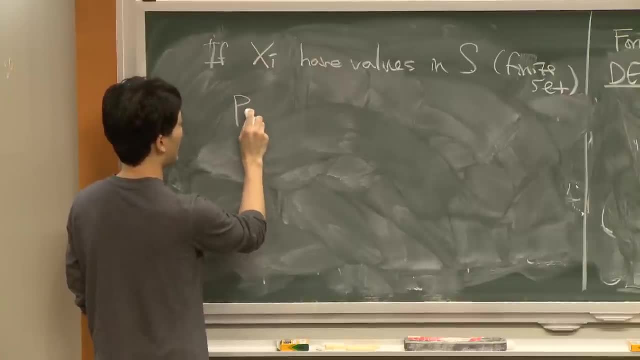 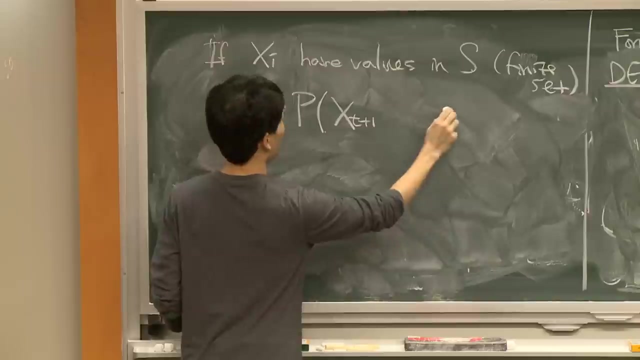 In that case it's really easy to describe Markov chains. Now denote the probability i- j as the probability that if, at time t, you are at i, the probability that you're going to be at j. Okay, So I'm going to use it. 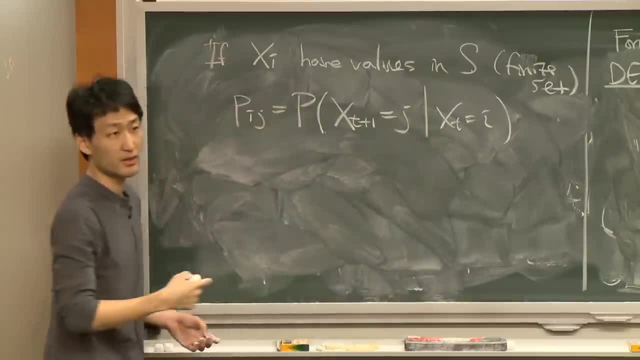 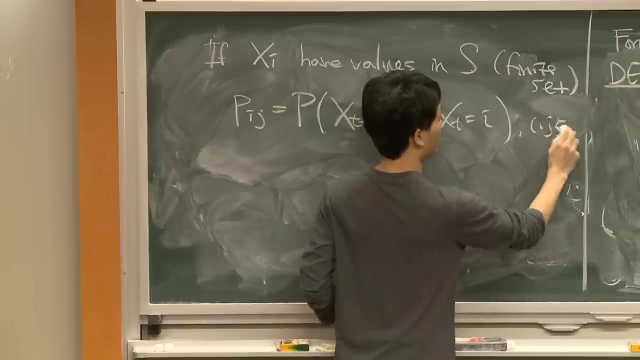 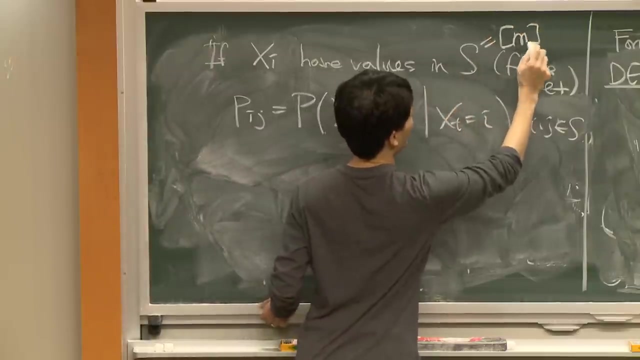 All right, So I'm going to use it. All right, jump to j at time. t plus 1 for all pair of points i j. I mean it's a finite set, so I might just as well call it the integer set from 1 to m. 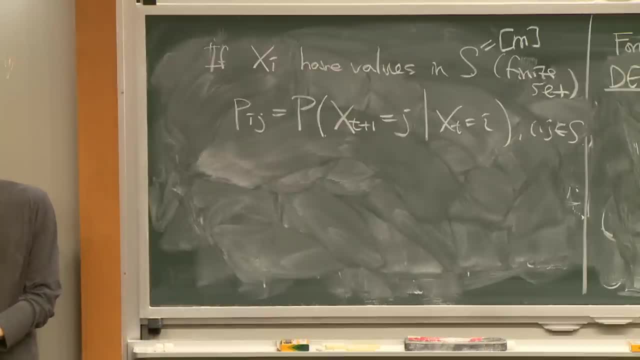 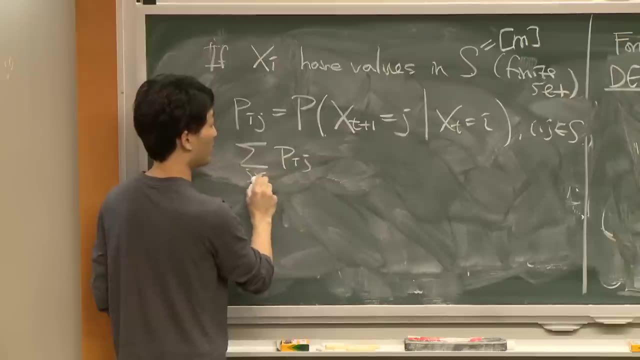 just to make the notation easier, Then to: first of all, if you sum over all j in S? pij, that is equal to 1. Because if you start at i, you'll have to jump to somewhere in your next step. 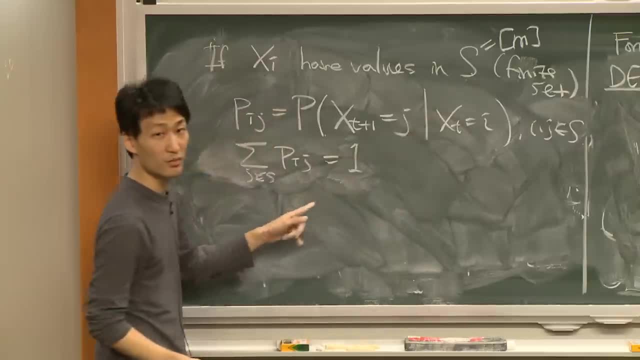 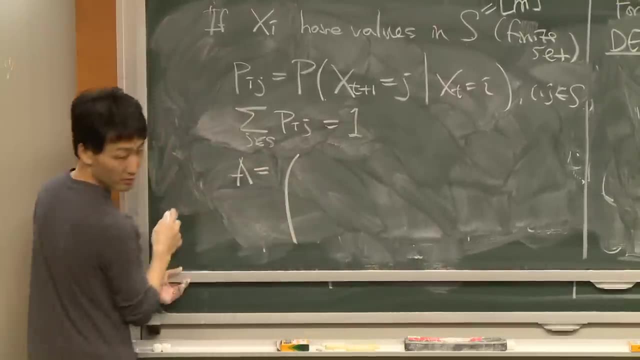 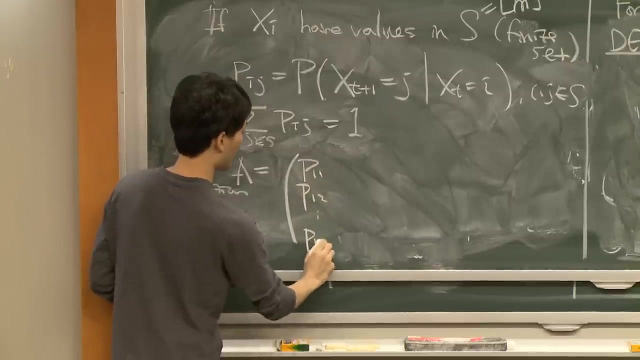 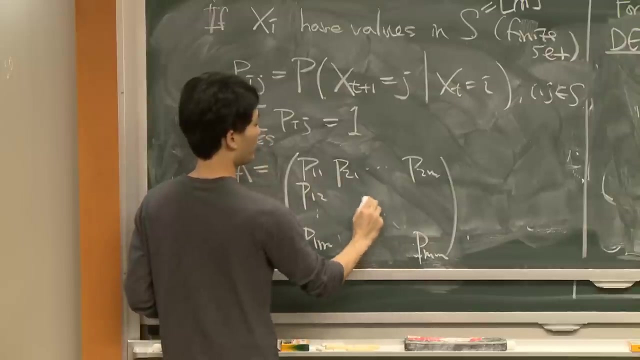 So if you sum over all possible states you can have, you have to sum up to 1.. And really a very interesting thing is this matrix called the transition and probability matrix, defined as p. this We put pij at i through o in j's column. 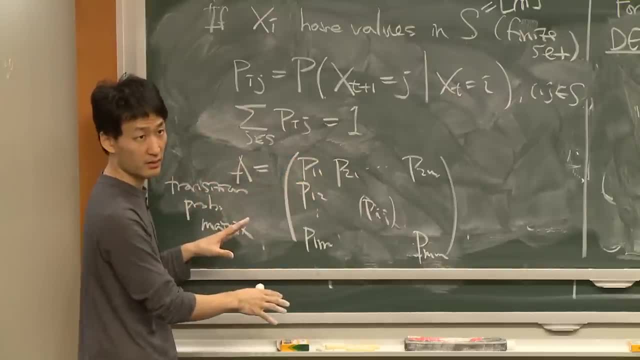 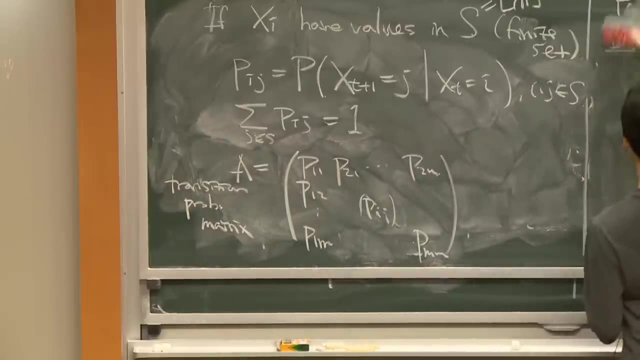 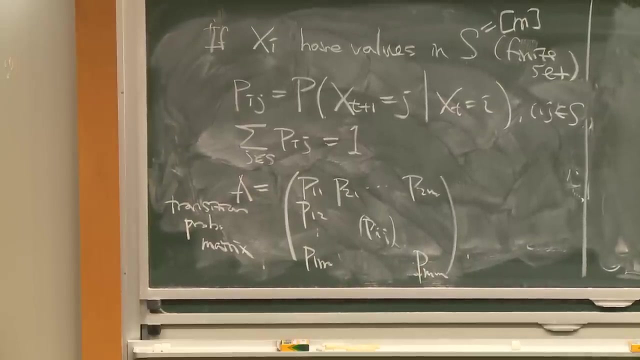 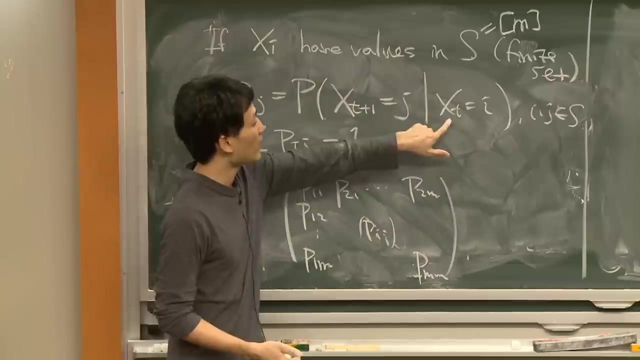 And really this tells you everything about the Markov chain. Everything About About the stochastic process is contained in this matrix. That's because a future state only depends on the current state. So if you know what happens at time t, where it's at time t, 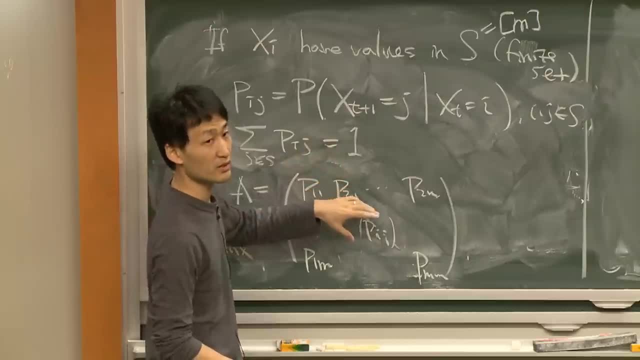 look at the matrix. You can decode all the information you want. What is the probability that it will be at? let's say it's at 0 right now. what's the probability that it will jump to 1 at the next time? 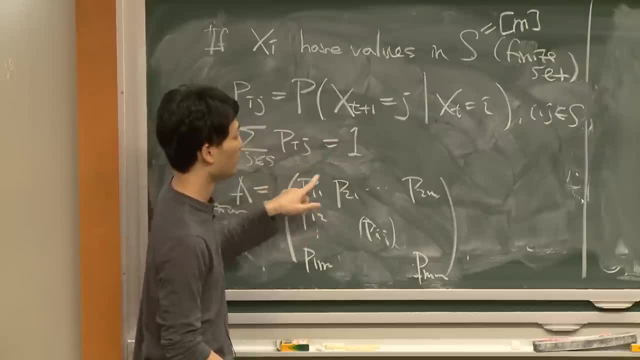 Just look at 0 comma 1 here. There's no 0, 1 here, So it's 1 and 2.. Just look at 1 and 2.. 1 and 2.. i and j, which I made a mistake. 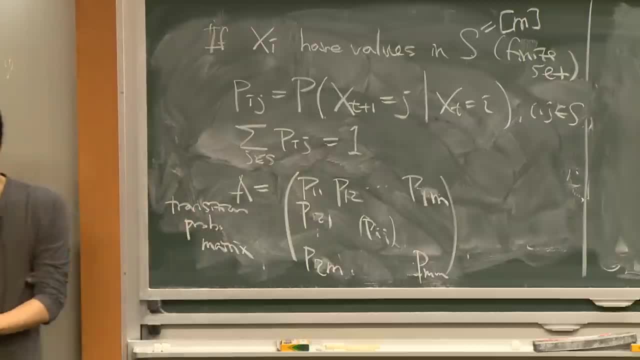 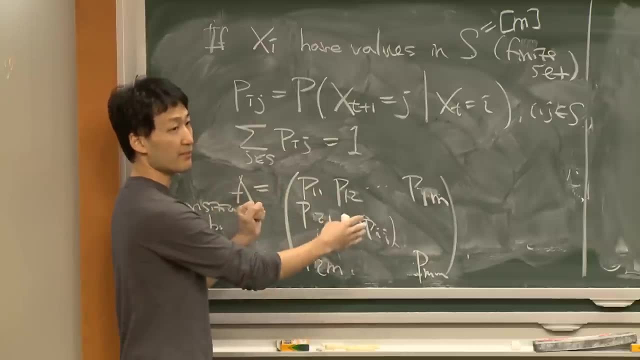 That should be the right one. Not only that, that's the one step. So what happens in 1, it describes what happens in a single step, the probability that you jump from i to j. But using that you can also model. 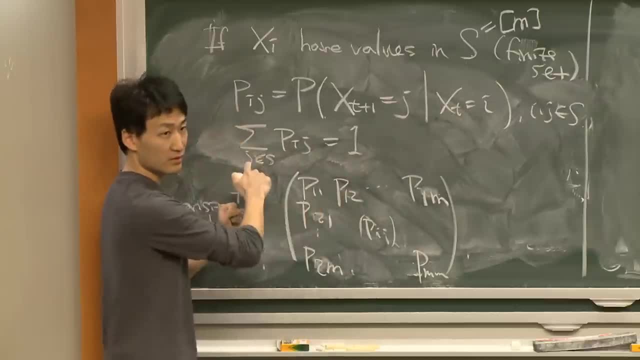 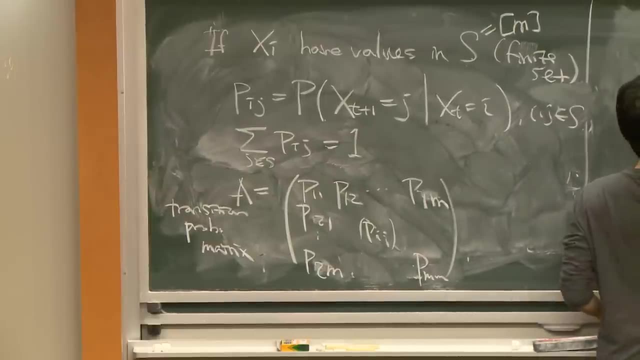 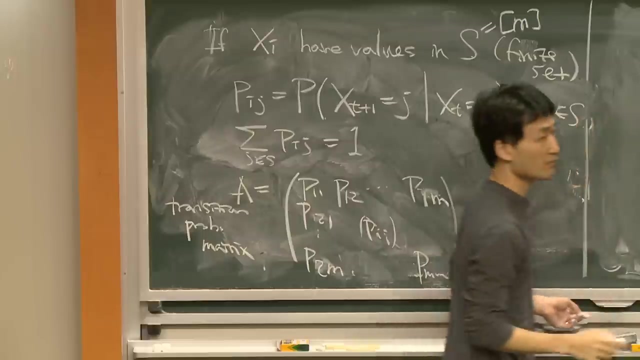 what's the probability? that you jump from i to j in two steps. So let's define q sub ij as probability that x at time t plus 2 is equal to j. given that x at time t is equal to i, Then the matrix defines: 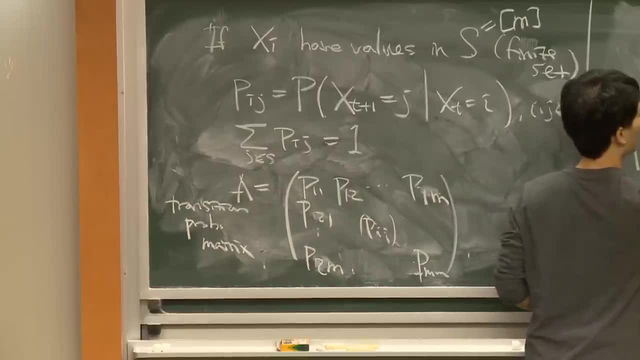 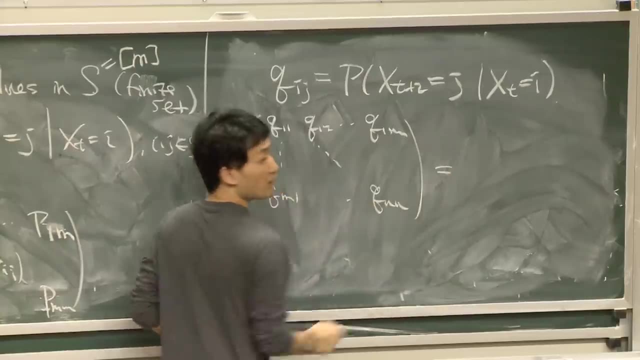 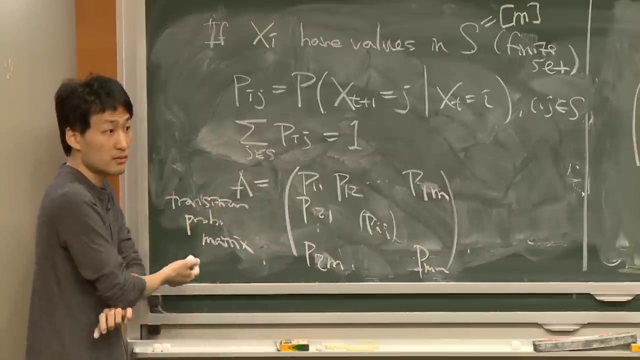 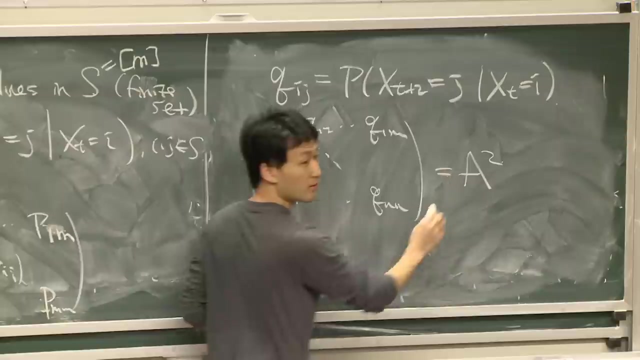 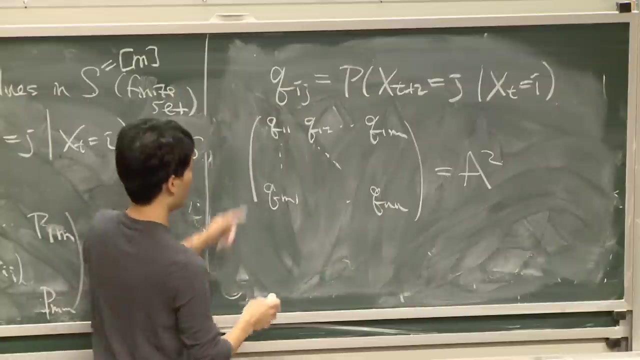 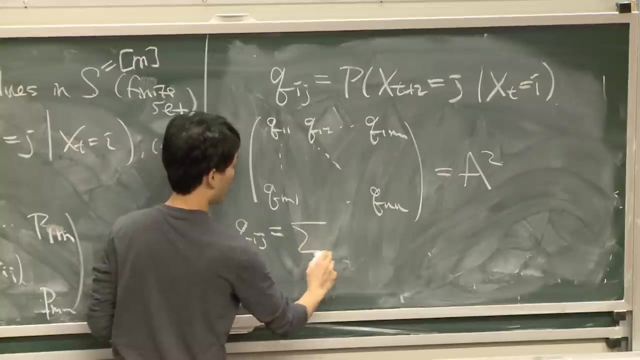 The matrix defined in this way. can you describe it in terms of the matrix, A Multiplication? Very good, It's A square. Why is it So? let me write this down in a different way: q, ij is you sum over all intermediate values. 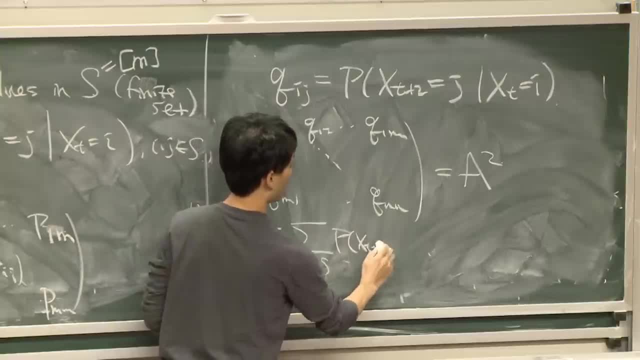 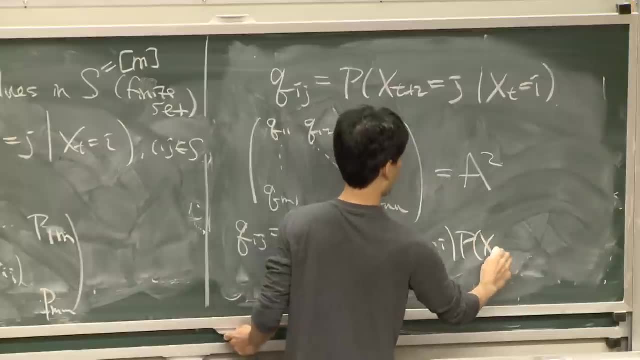 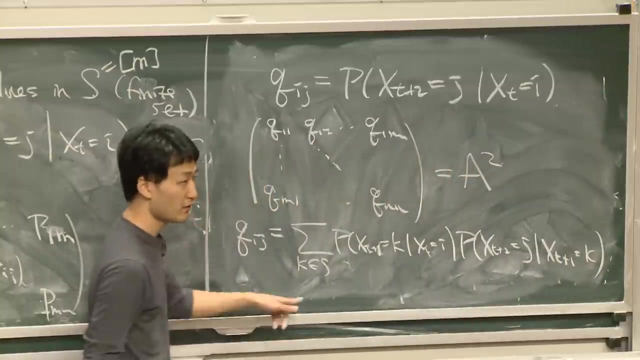 the probability that you jump from i to k first and then the probability that you jump from k to j, And if you look at what this means, it's exactly. each entry here is described by a dot, product of two, a column in a row. 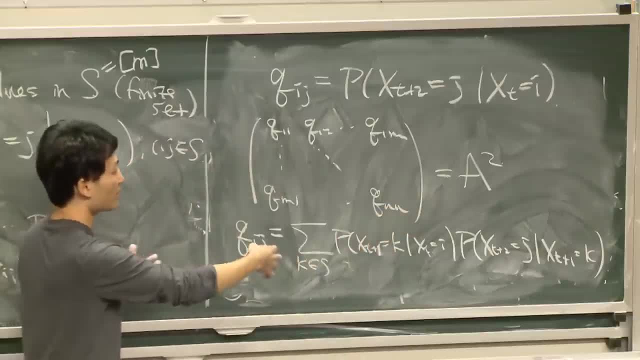 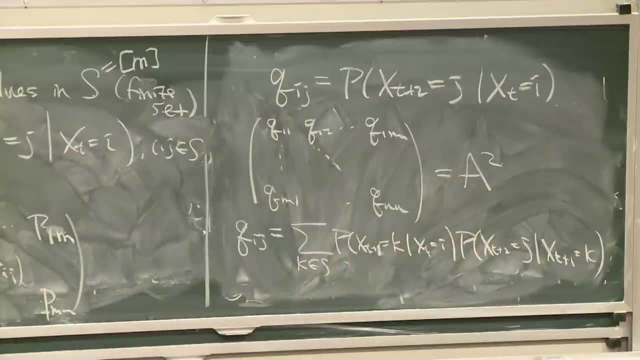 And that's exactly the equation. And if you want to look at the three step, four step, all you have to do is just multiply it again and again and again. Really, this matrix contains all the information you want if you have a Markov chain and it's finite. 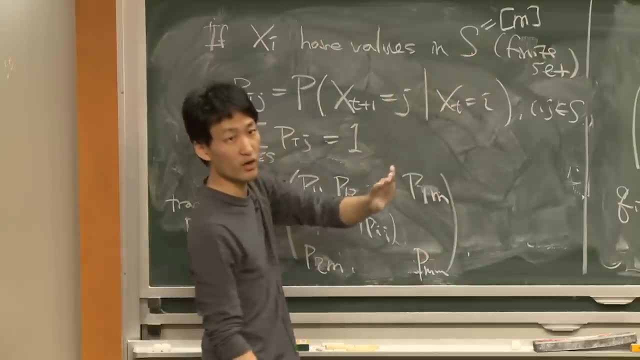 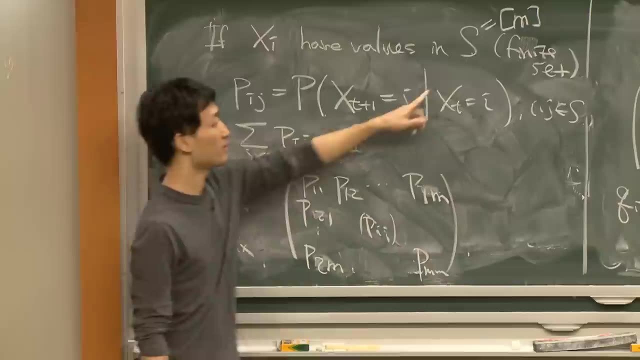 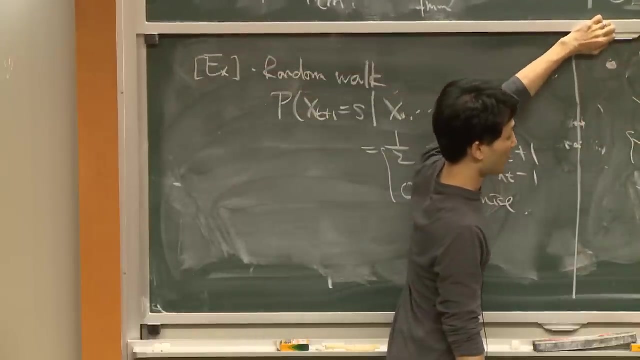 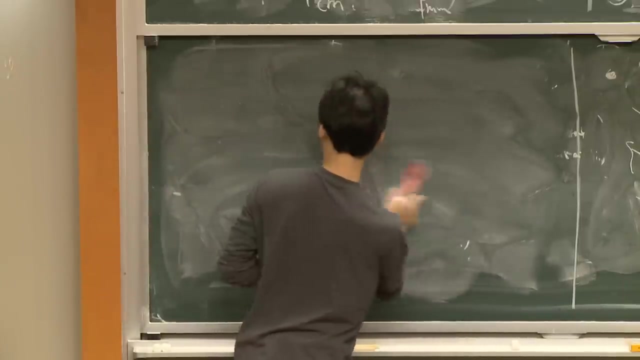 That's very important. For random walk, Simple random walk. I told you that it is a Markov chain, But it does not have a transition probability matrix because the state space is not finite. So be careful. However finite Markov chains, really there is one matrix. 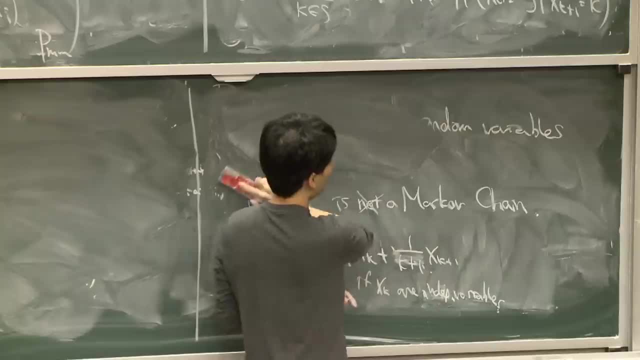 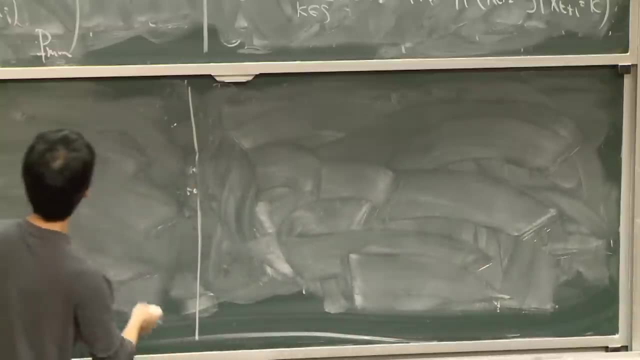 that describes everything. I mean, I said it like it's something very interesting, But if you think about it it's not. If you think about it, you just wrote down all the probabilities, So it should describe everything And that's it. 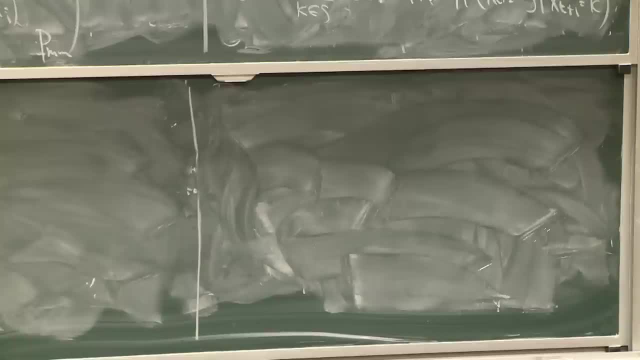 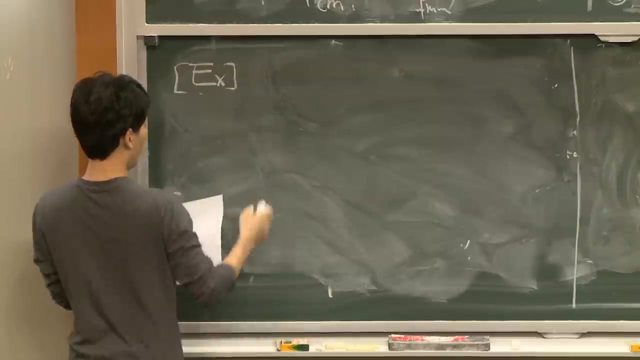 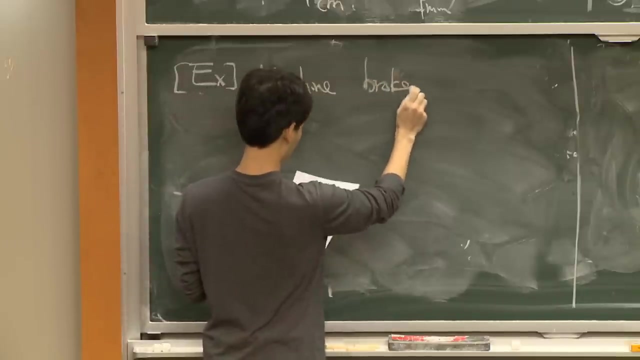 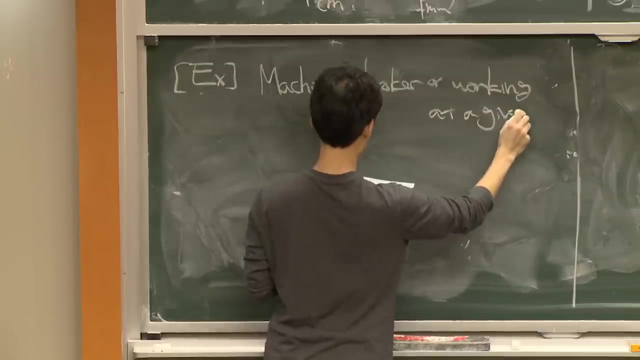 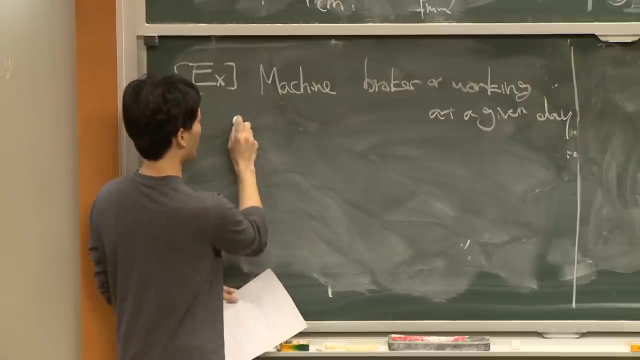 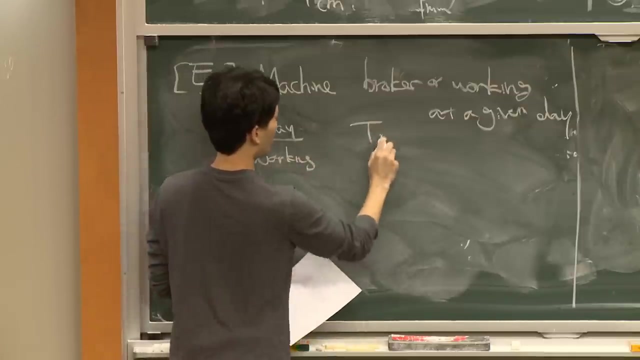 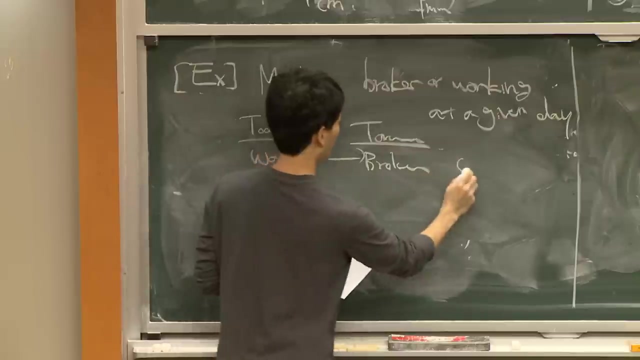 OK, so now so an example. you have a machine And it's broken or working at a given day. That's a silly example. So if it's working today, working tomorrow, broken with probability 0.01,, working with probability 0.99.. 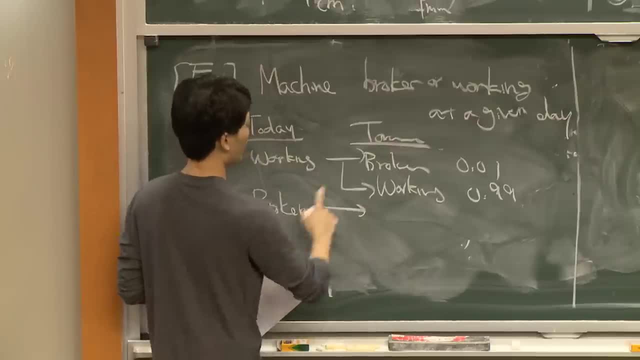 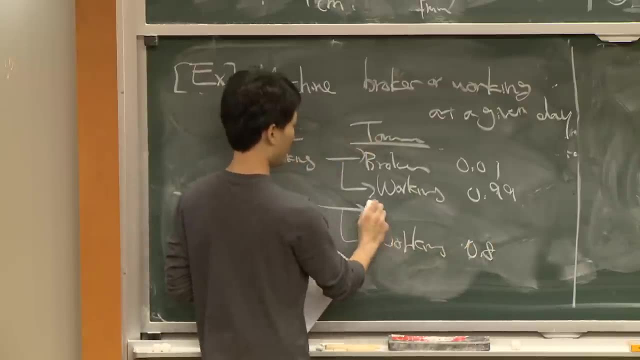 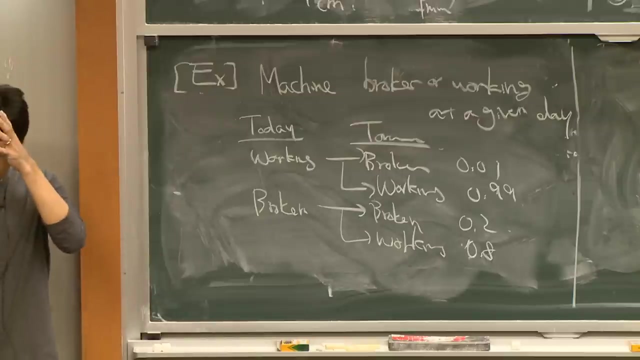 If it's broken, the probability that it's repaired on the next day is 0.8.. And if it's broken, it's 0.2.. Suppose you have something like this. OK, This is an example of a Markov chain. 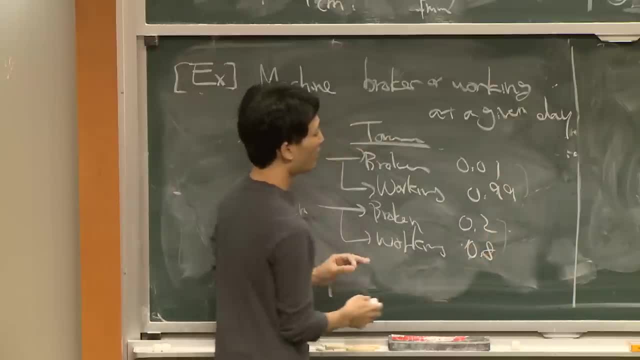 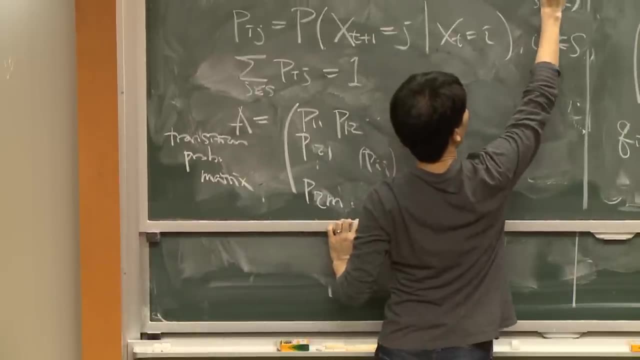 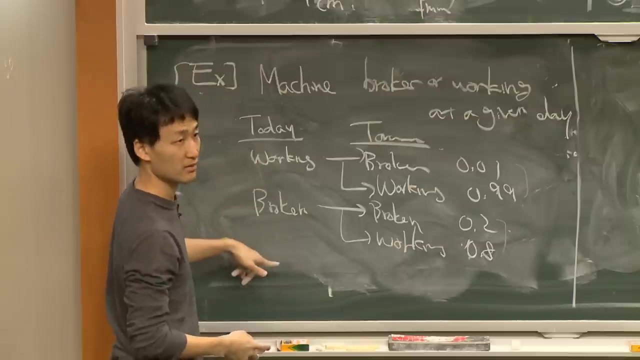 used in engineering applications. So many cases the reason I call s is also called. in this case, s is also called a state space actually, And the reason is because many cases what you're modeling is these kind of states of some system, like broken or working. 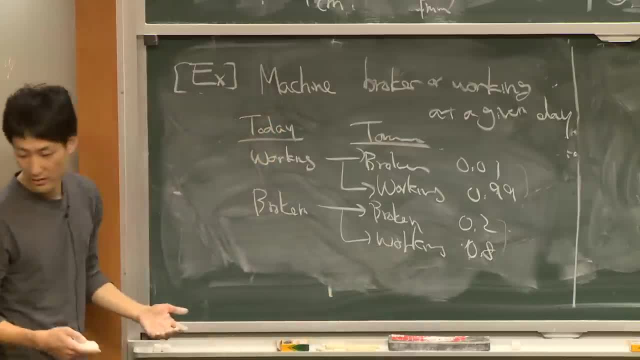 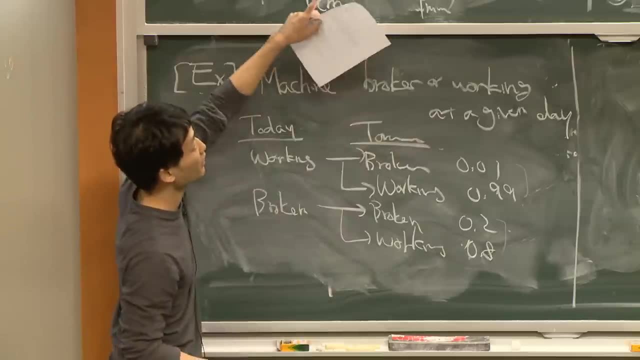 raining, rainy, sunny, cloudy- OK, OK, OK, It's cloudy, it's weather, And all these things that you model represent states a lot of time, So you call it state set as well. So that's an example. 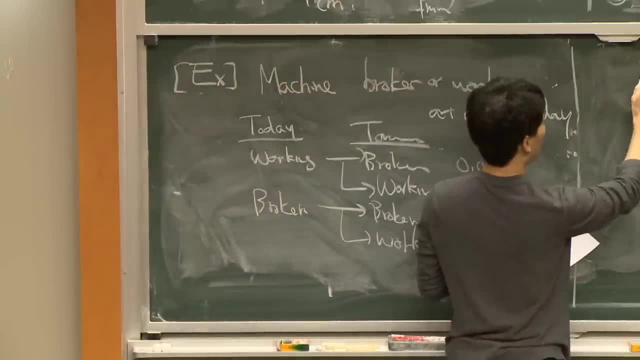 And let's see what happens for this matrix. So you have two states: working and broken. So if it's working, working to working is 0.99.. Working to broken is 0.01.. Broken to working is 0.8.. 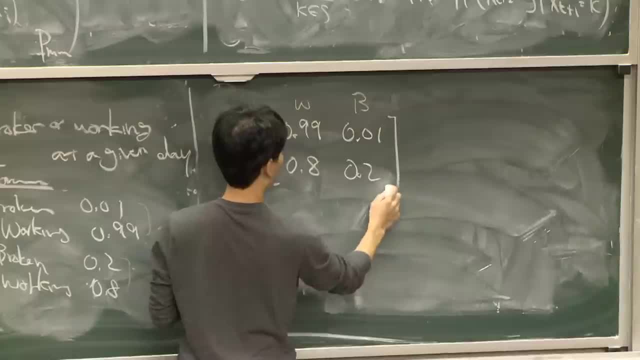 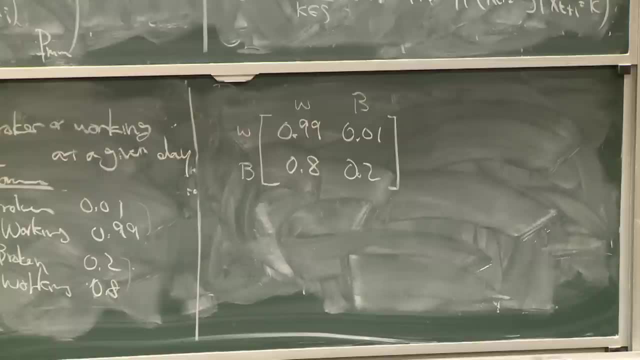 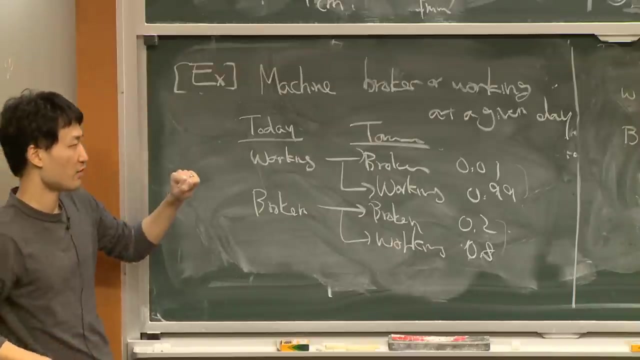 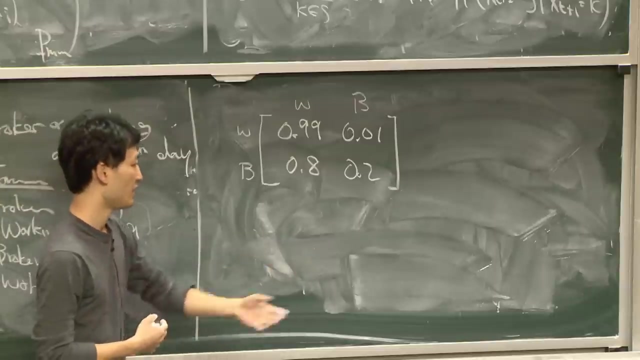 Broken to broken is 0.2.. OK, So that's what we learned so far. And the question: what happens if you start from some state- Let's say it was working today- And you go a very, very long time, like a year or 10 years? 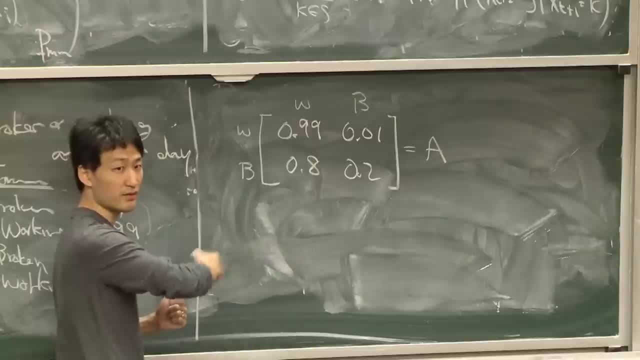 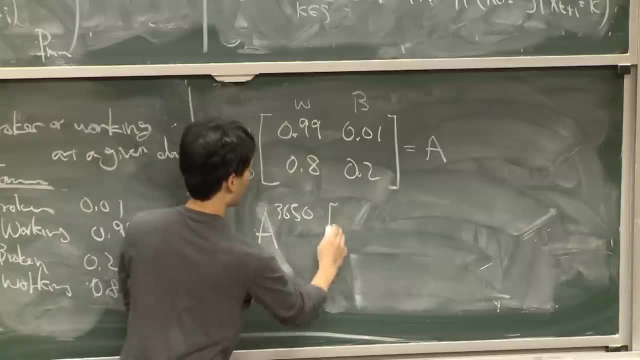 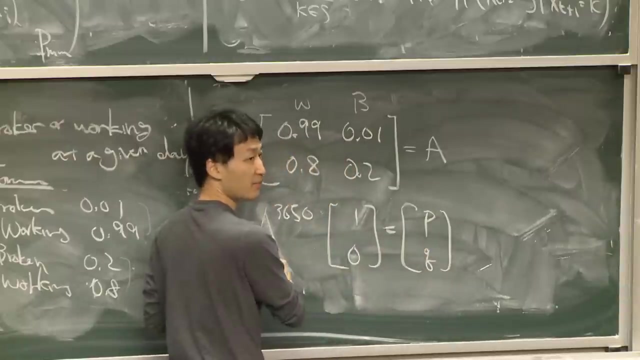 OK, Then the distribution after 10 years on that day is 8 to the 3,650.. That will be that times 1, 0 will be the probability pq. p will be the probability that it's working at that time. 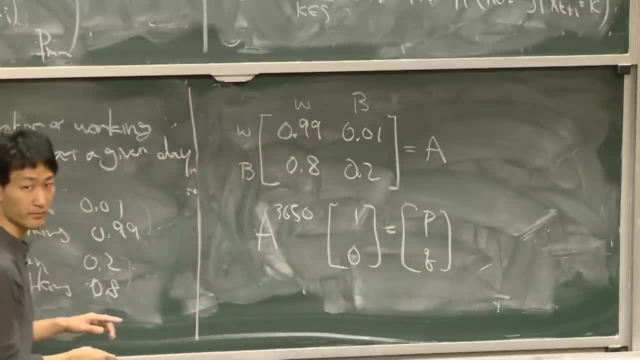 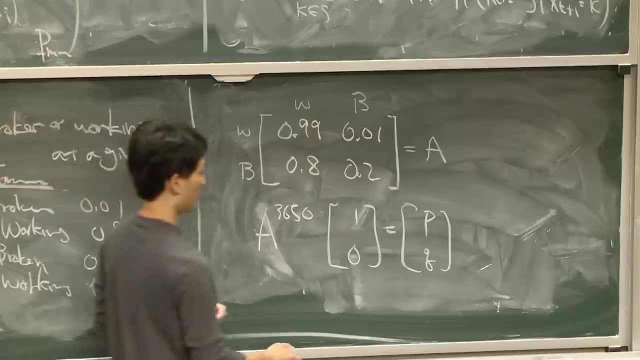 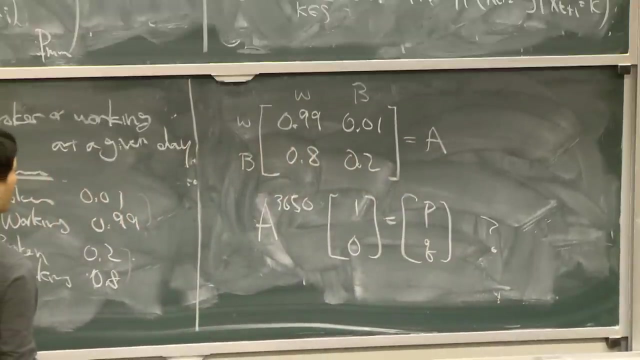 q will be the probability that it's broken. at that time, What will p and q be? What will p and q be? That's the question that we're trying to ask now. We didn't learn so far how to do this, But let's think about it. 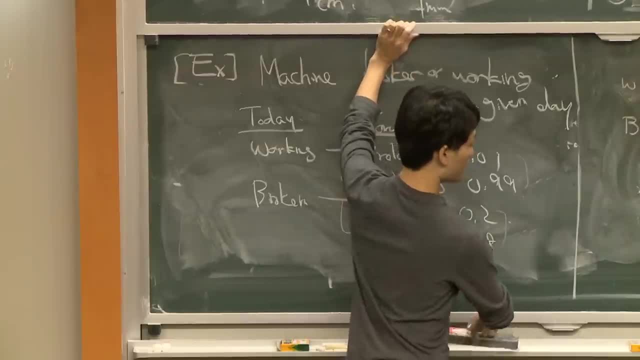 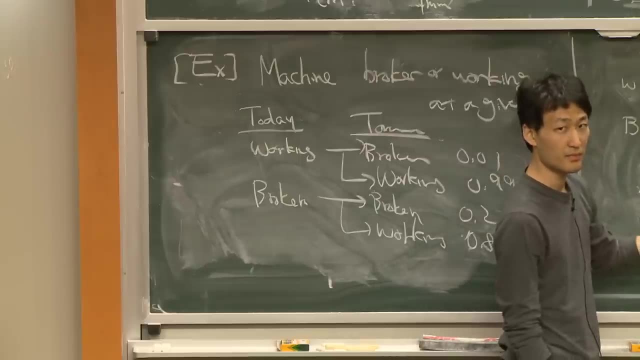 Just, I'm going to cheat a little bit And just say you know what I think: if, over a long period of time, Yes, Yes, Yes, Yes, The probability distribution on day 3,650 and that on day 3,651 shouldn't be that different. 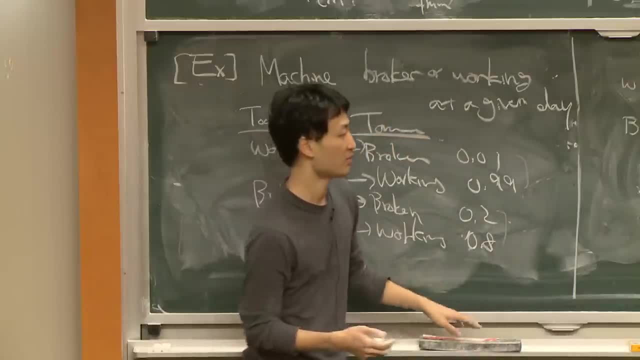 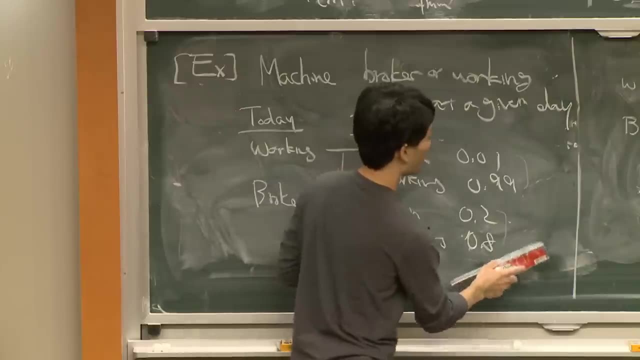 They should be about the same. Let's make that assumption. I don't know if it's true or not. Well, I know it's true, but that's what I'm telling you. Under that assumption, now you can solve what p and q are. 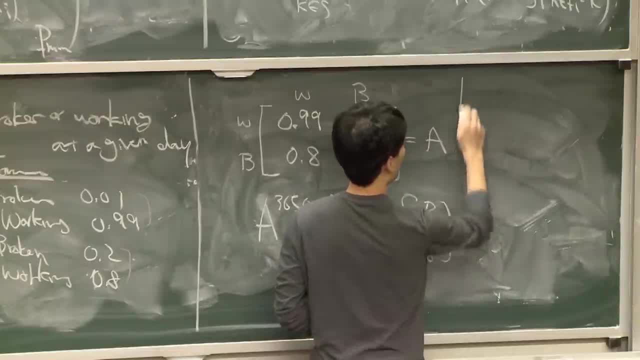 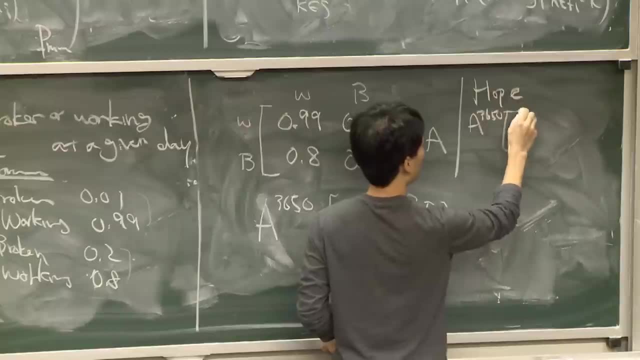 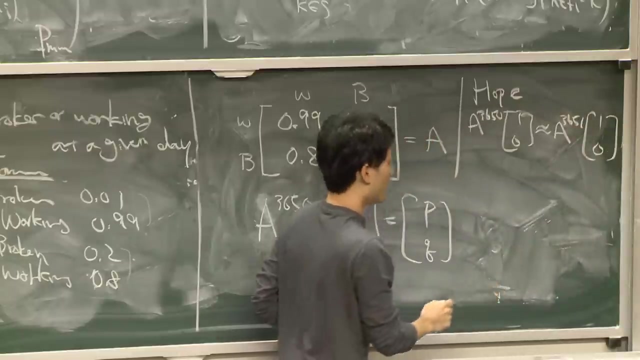 So and approximately- I hope I hope pq. so a 3,650, 1, 0, is approximately the same as h of 3,651, 1, 0. That means, if this is pq, pq is about the same as a times pq. 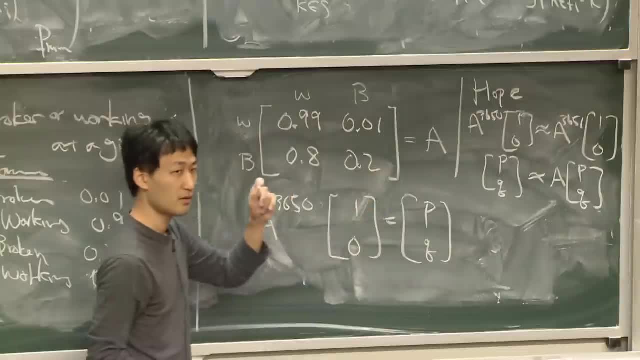 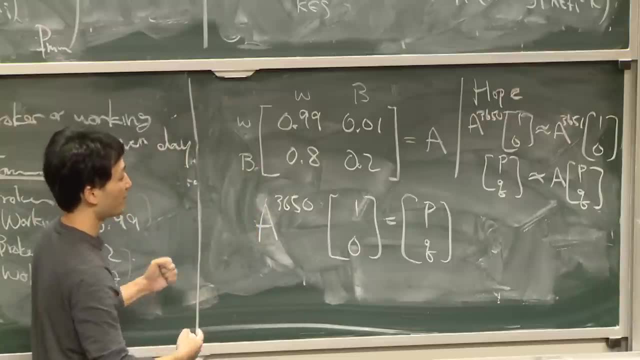 Anybody remember what this is? Yes, So pq will be the eigenvector of this matrix Over a long period of time. the probability distribution that you will observe will be the eigenvalue eigenvector. And what's the eigenvalue? 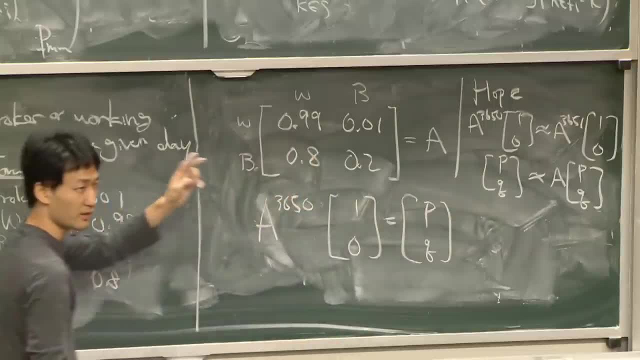 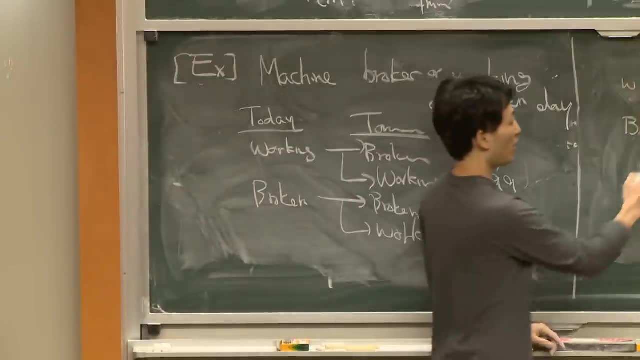 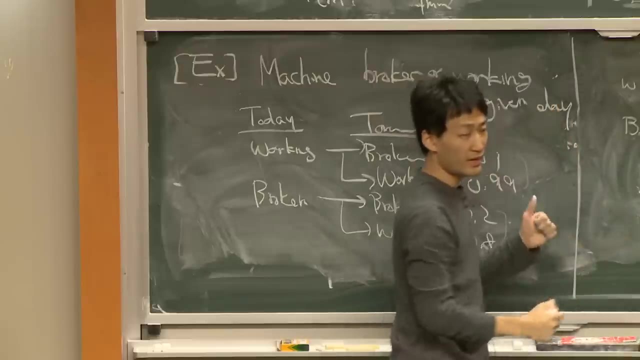 1. At least in this case it looks like it's 1.. OK, Now I'll make one more connection. Do you remember Perron-Frobenius theorem? This is a matrix. All entries are positive, So there is a largest eigenvalue, which is positive and real. 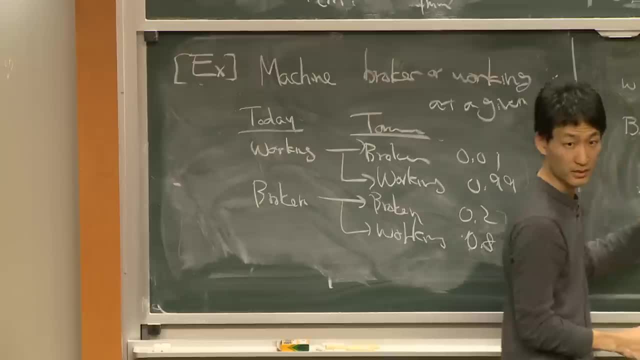 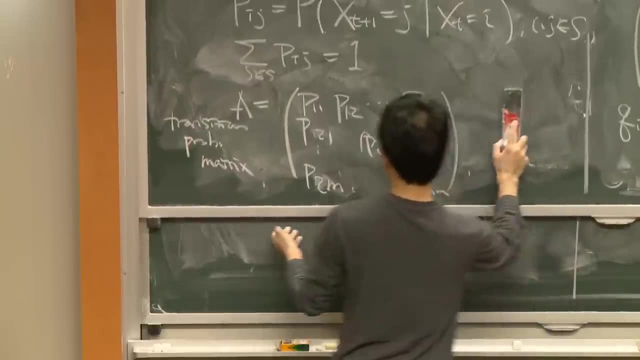 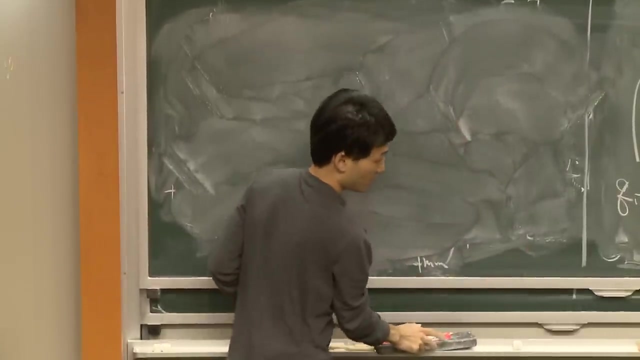 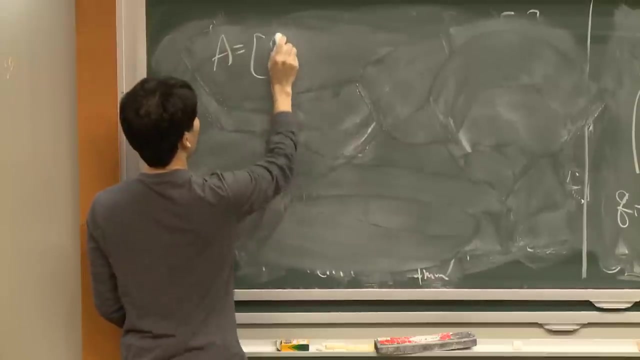 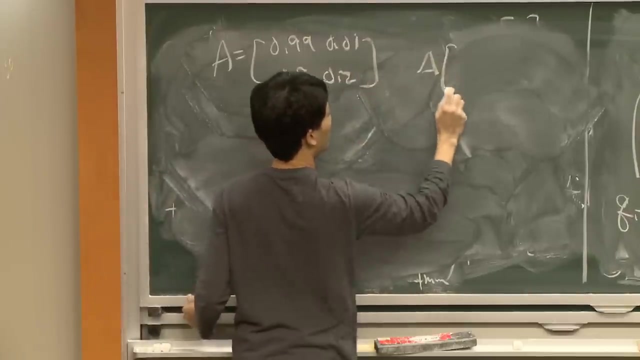 And there is an all-positive eigenvector corresponding to it. What I'm trying to say is: that's going to be your pq, But let me not jump to the conclusion yet. And then what we know is: this is a. And one more thing we know is: from pi, and then from pi, and then from pi, it's going to be a. 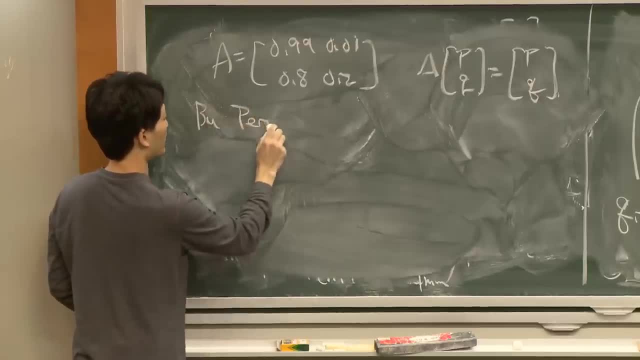 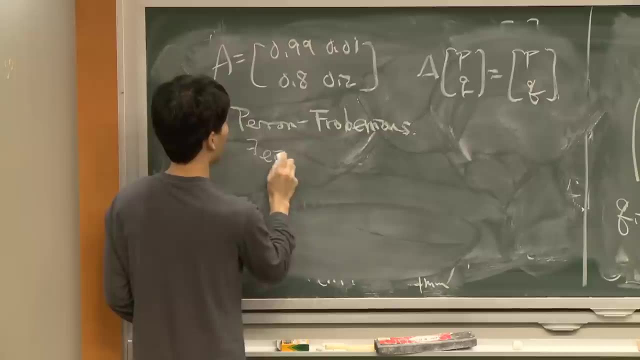 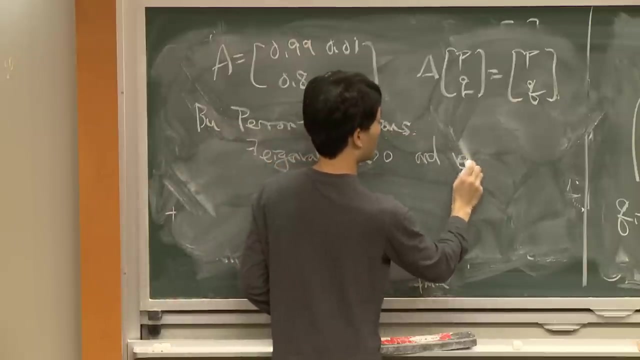 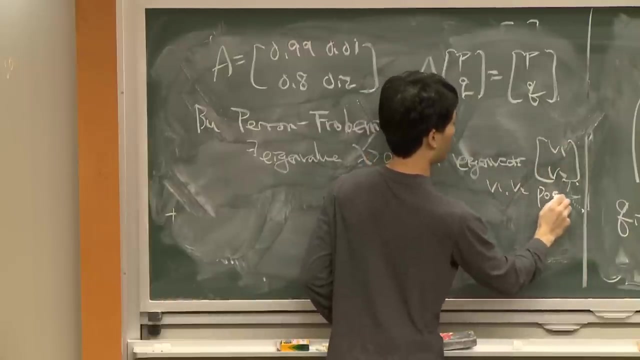 So is from by Perun Rubinius. there exists an eigenvalue- largest one, lambda- greater than 0, and eigenvector v1, v2, where v1, v2 are positive. Moreover, lambda was at multiplicity 1.. 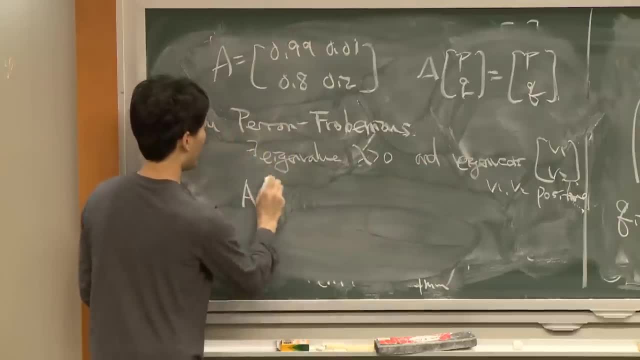 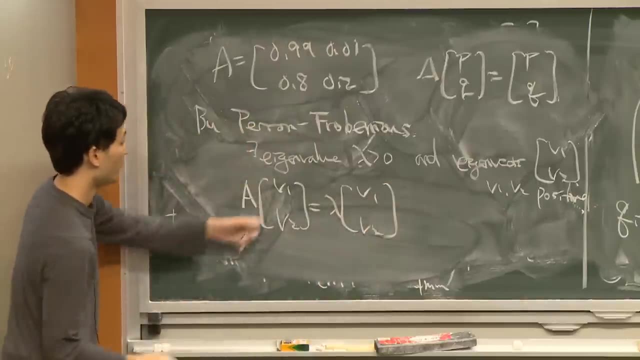 I'll get back to it later. So let's write this down: a times v1, v2 is equal to lambda times v1, v2.. a times v1, v2, we can write it down It's 0.99v1 plus 0.01v2.. 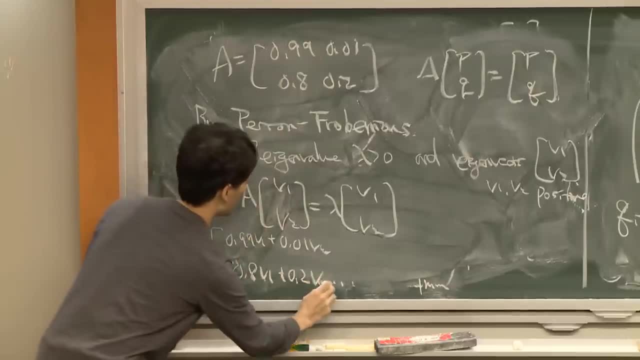 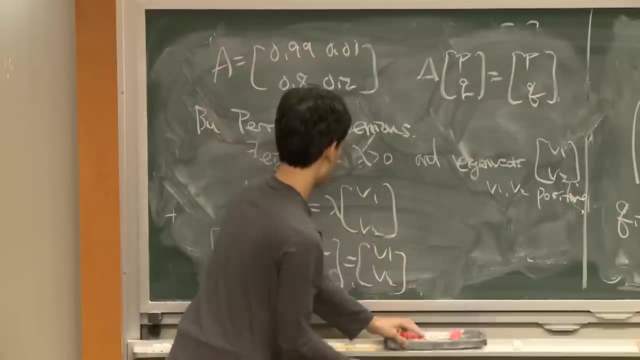 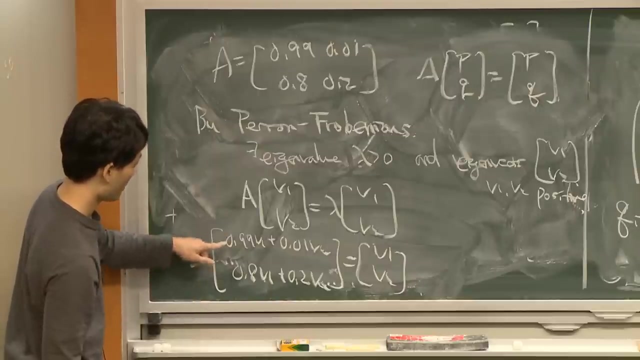 And that's 0.8v1 plus 0.2v2, which is equal to v1, v2.. OK, you can solve v1 and v2.. But before doing that, p sorry about that. This is flipped. 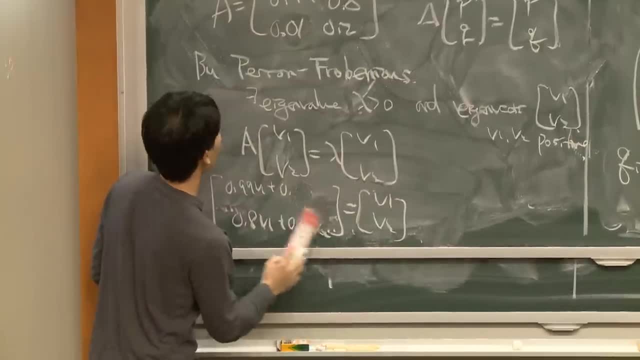 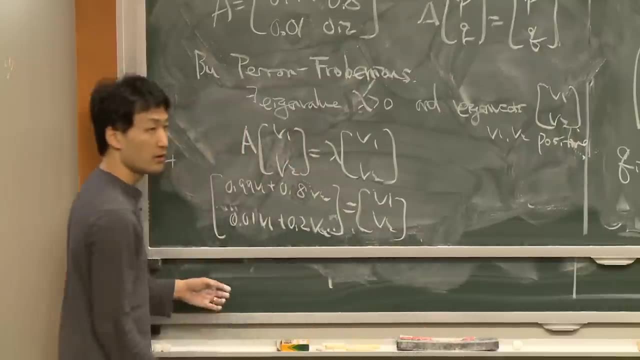 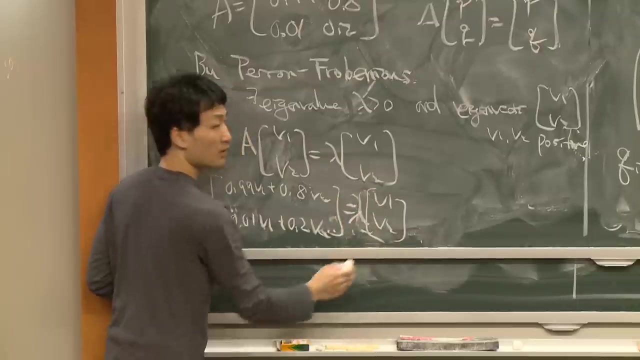 Yeah, sorry about that. It should have been flipped in the beginning. What's that? OK? So sum these two values and you get lambda times v1, v2.. On the left, what you get is v1 plus v2.. 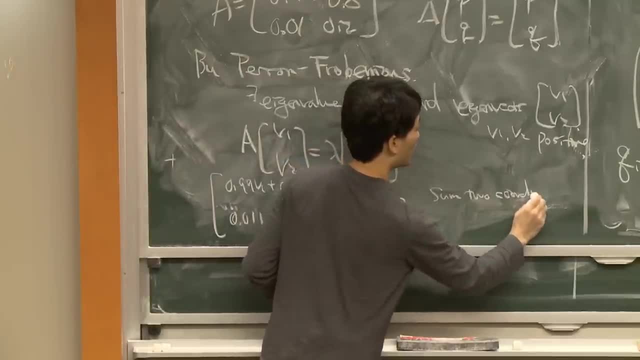 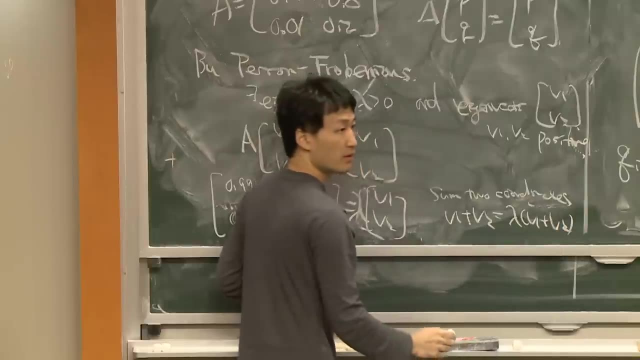 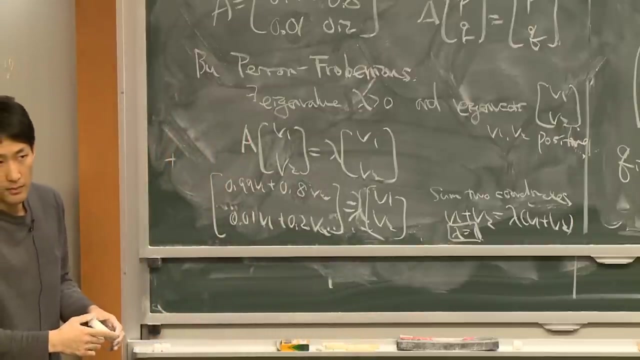 So sum two coordinates: On the left you get v1 plus v2.. On the right you get lambda times v1 plus v2.. That means your lambda is equal to 1.. OK, So that eigenvalue guaranteed by Perron-Probenius theorem. 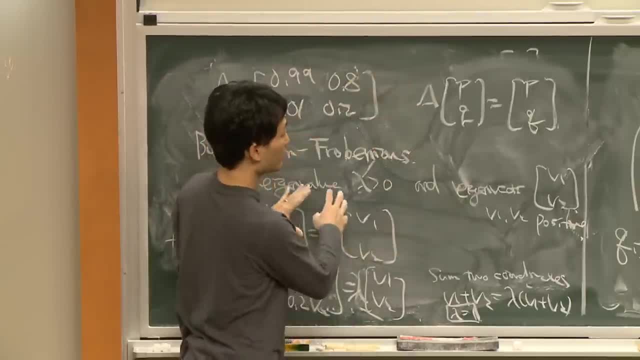 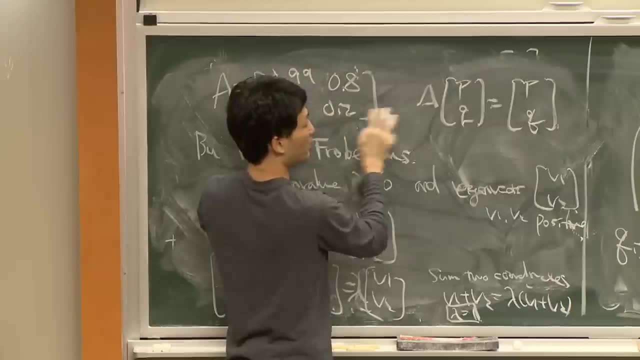 is 1.. Eigenvalue is 1.. So this, what you'll find here, will be the eigenvector corresponding to the largest eigenvalue. Eigenvalue Eigenvector will be the one corresponding to the largest eigenvalue, which is equal to 1.. 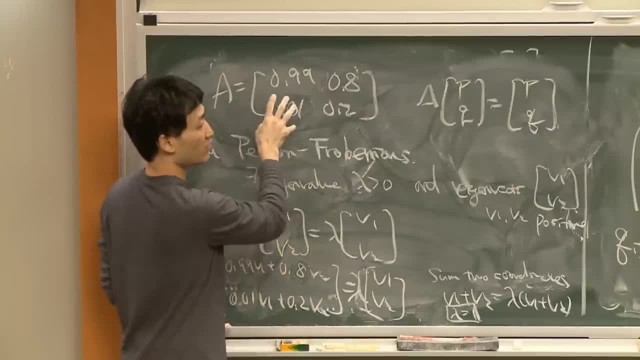 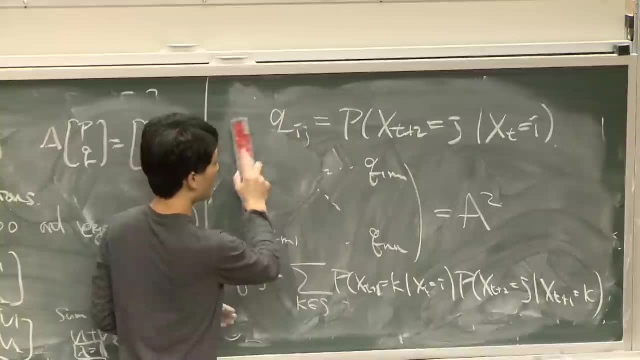 And that's something very general. It's not just a general, It's just about this matrix and this special example. In general, if you have a transition matrix, if you're given a Markov chain and given a transition matrix, Perron-Probenius theorem guarantees. 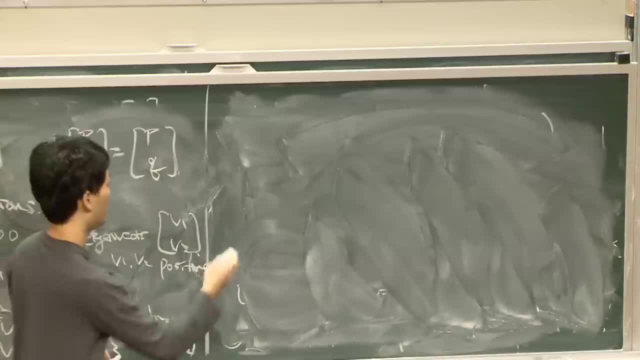 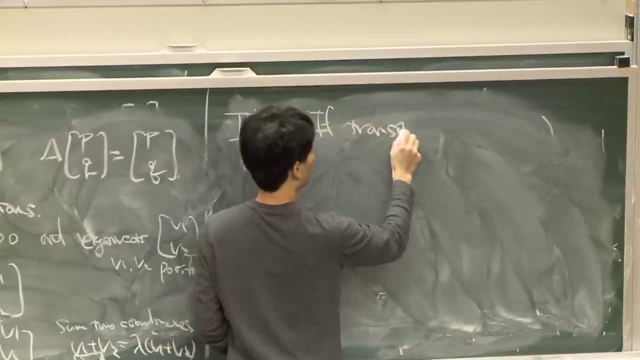 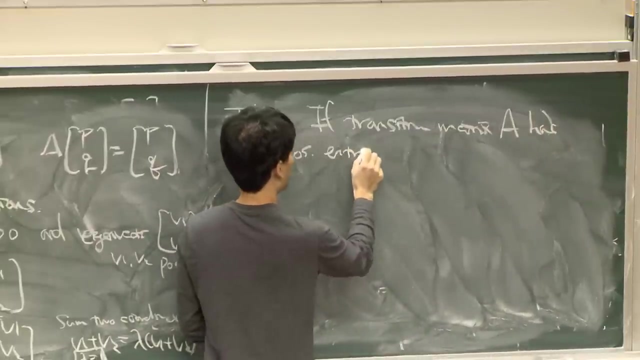 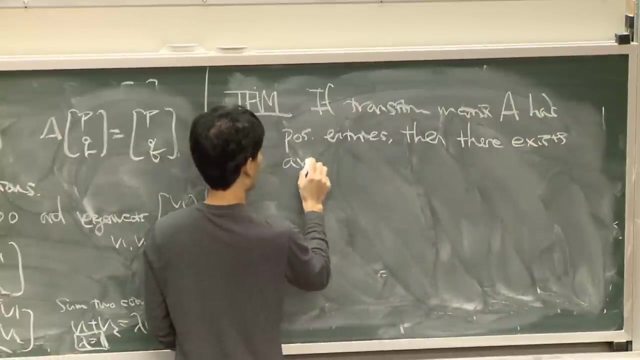 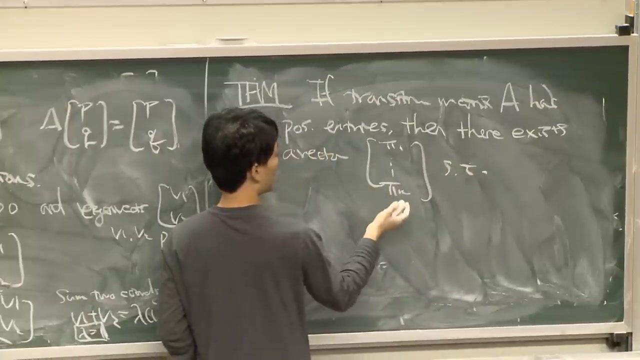 that there exists a vector as long as all the entries are positive. So in general, if transition matrix of a Markov chain has positive entries, Then there exists a vector, pi 1 up to pi m, such that a v is equal to v. 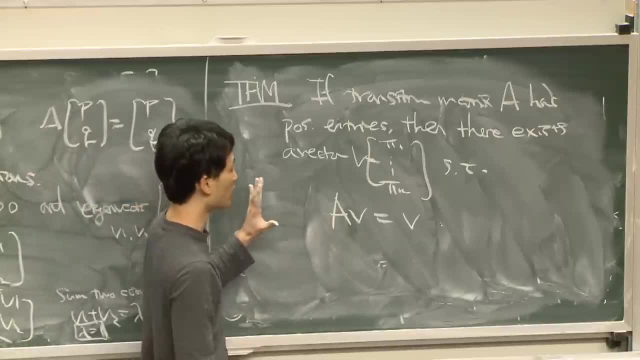 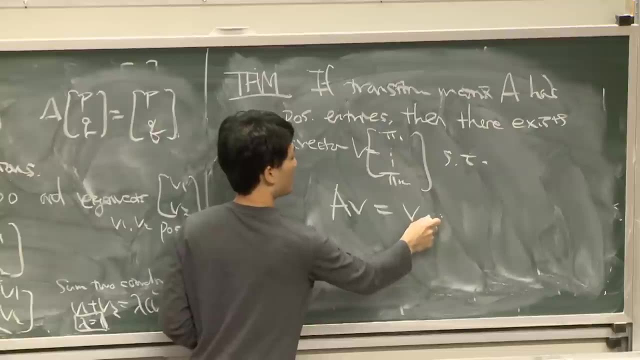 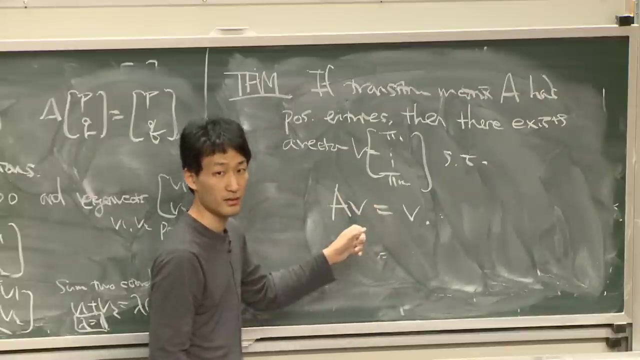 And that will be the long-term behavior as explained Over a long term. if it converges to some state, it has to satisfy that And by Perron-Probenius theorem we know that there is a vector satisfying it. So if it converges, it will converge to that. 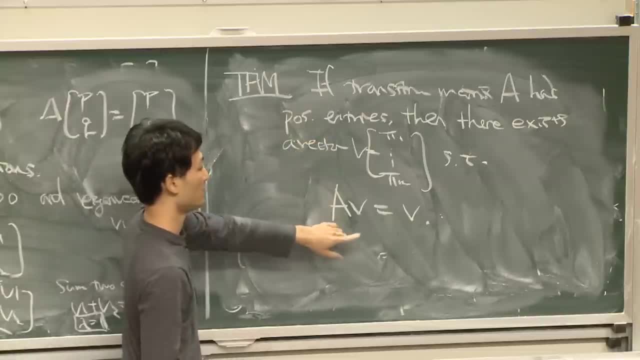 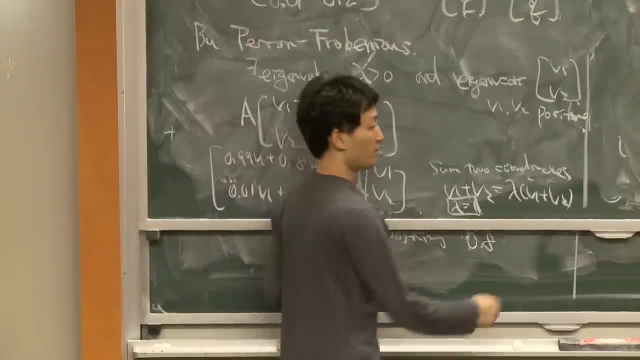 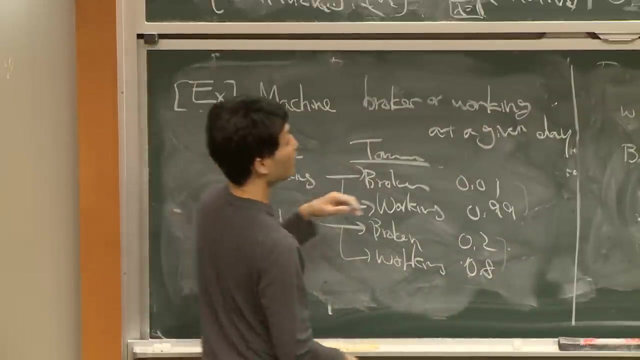 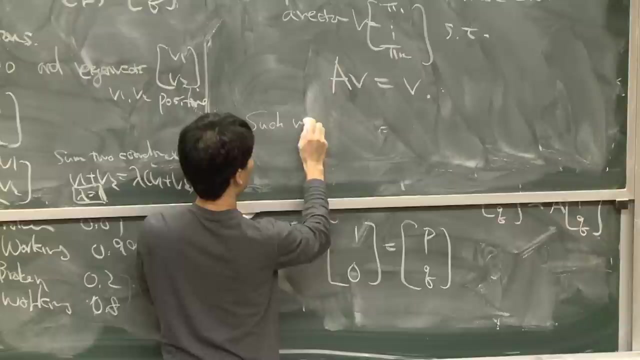 And what it's saying is: if all the entries are positive, then it converges And there is such a state. We know the long-term behavior of the system. OK, So this is called a stationary distribution. such vector v is called. 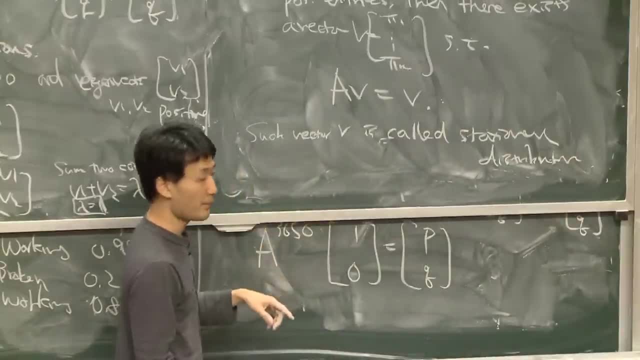 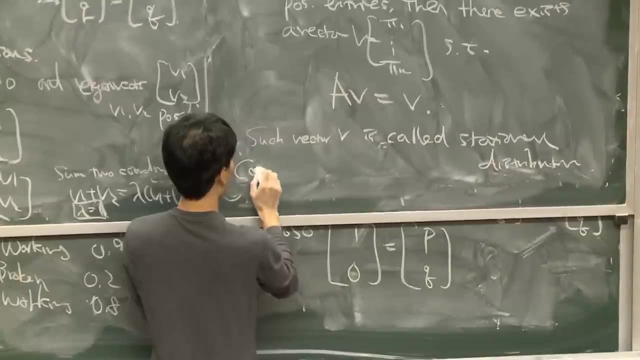 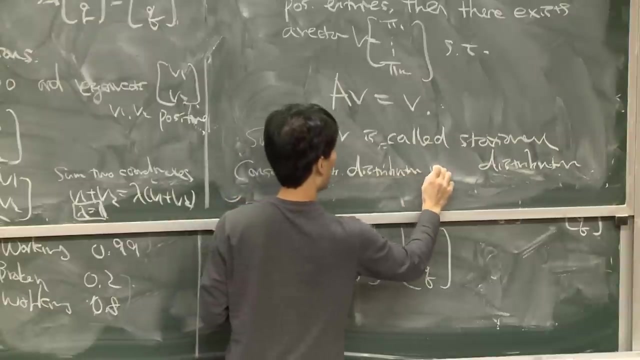 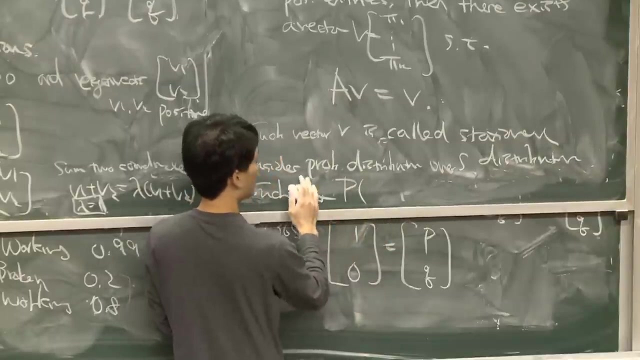 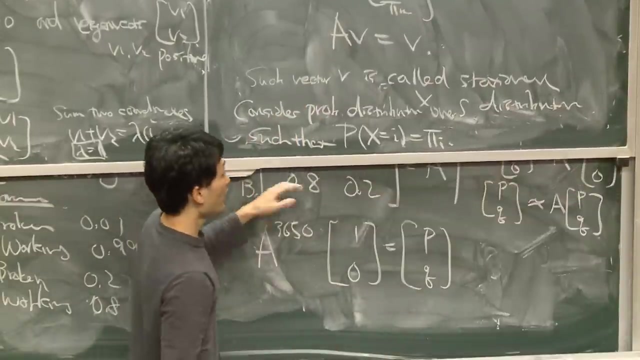 OK, it's not really right to say that a vector is stationary distribution, But if I give this distribution to the state space, what I mean is consider Probability distribution over s such that probability is, with the random variable, x, x is equal to i is equal to pi i. 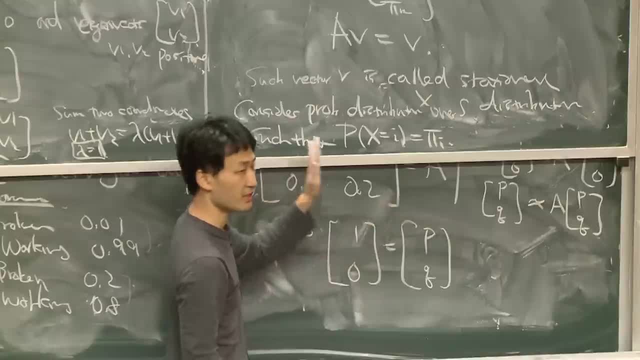 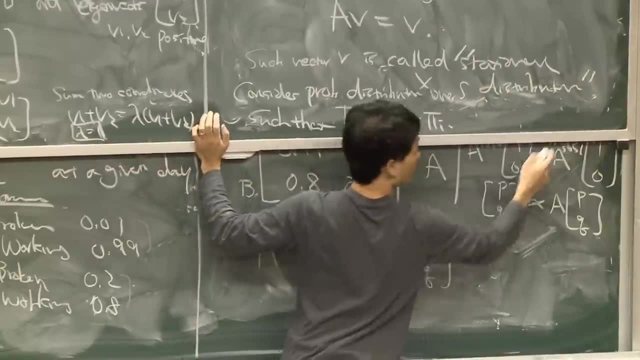 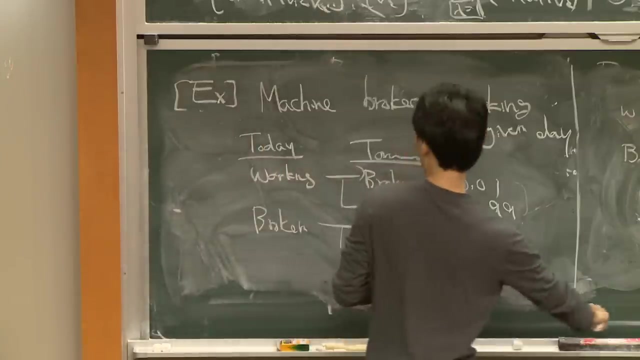 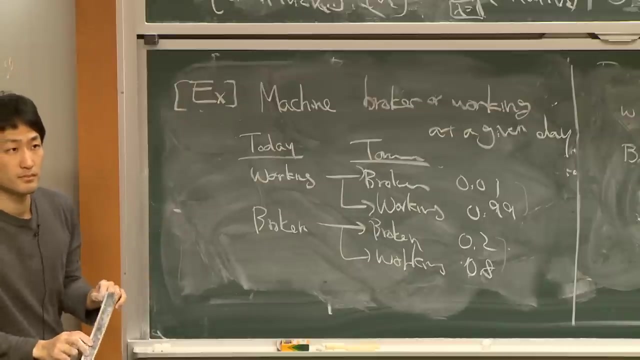 If you start from this distribution, in the next step you'll have the exact same distribution. That's what I'm trying to say here. That's called a stationary distribution. OK, Any questions? And So both of them have the same number of eigenvectors. 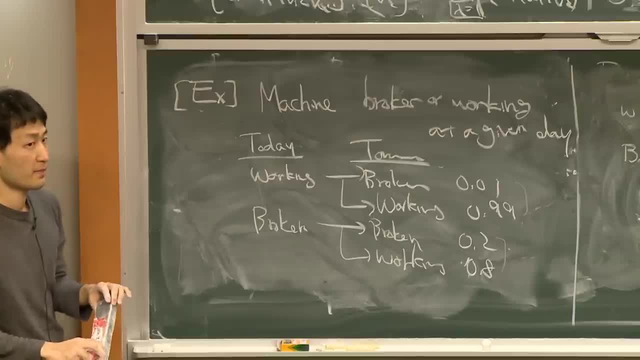 And there are more eigenvectors? Yes, very good question, But yeah, Yeah, but Perron-Probenius theorem says there is exactly one eigenvector corresponding to the largest eigenvector, The eigenvalue, And that turns out to be 1.. 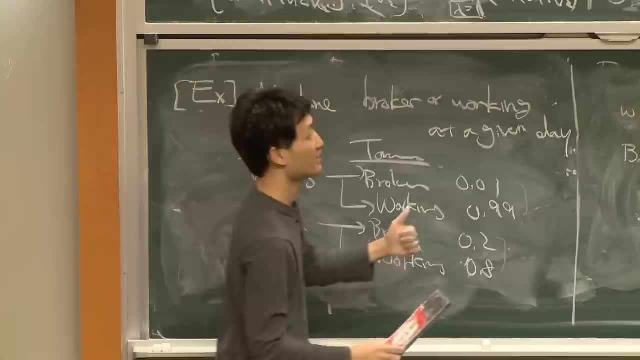 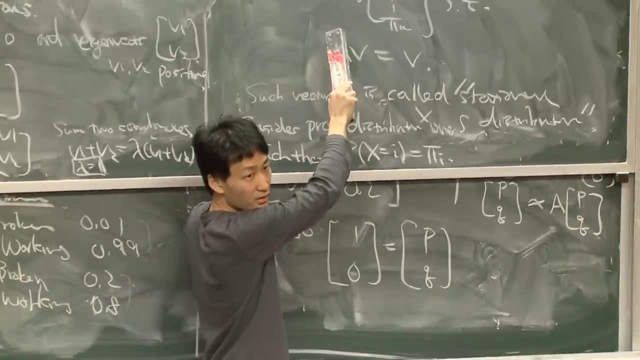 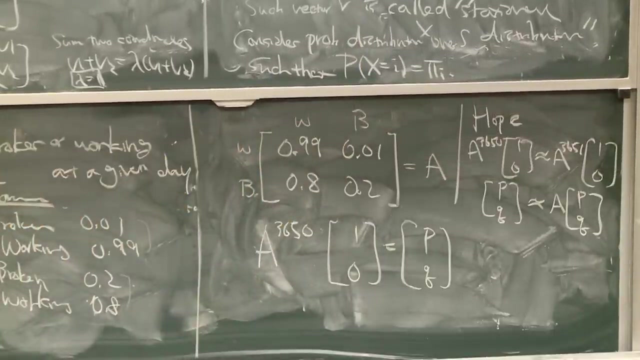 The largest eigenvalue turns out to be 1.. So there will be a unique stationary distribution if all the entries are positive, And then all of the eigenvalues of the graph will be the same. This one, Oh, that's a good one. 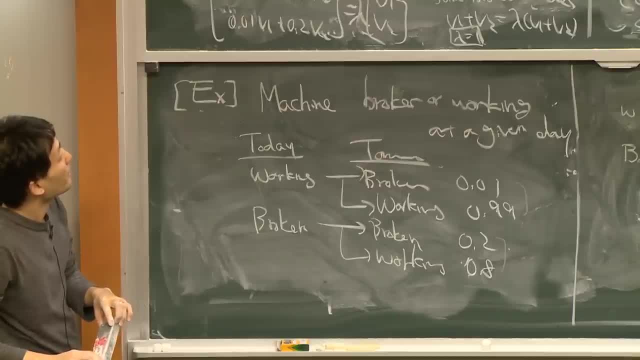 That implies: So this one, Oh this one, The eigenvectors are positive, And the eigenvectors are positive. So the eigenvectors are positive, And if all the pointers, if all the pointers are positive, then the eigenvectors are positive. 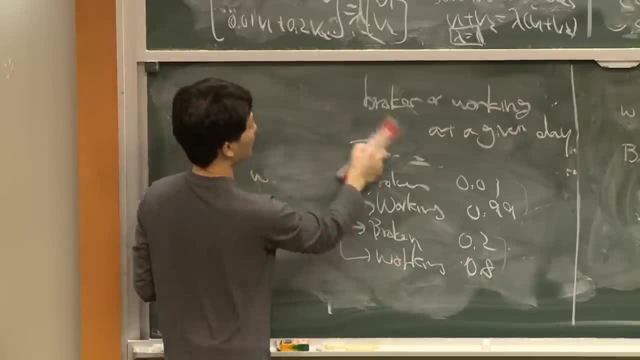 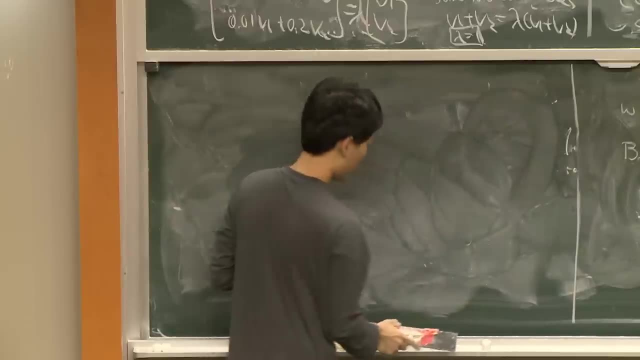 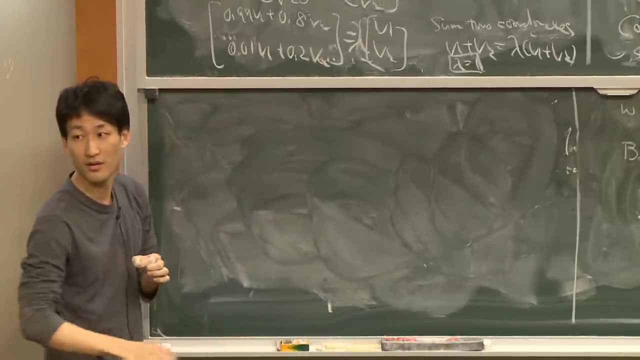 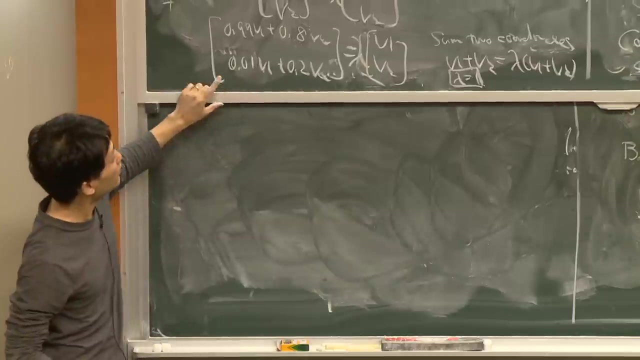 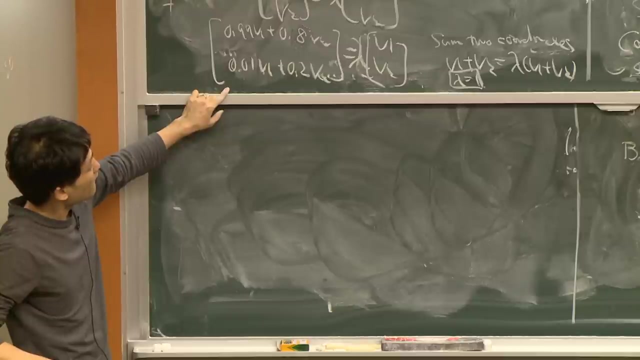 Good, OK, OK, Okay, can anybody help me? This part looks questionable. So when you take products of the transition probability matrix, those eigenvalues, they're smaller than one scale after repeated multiplication to zero. So yeah, In the limit they're zero. 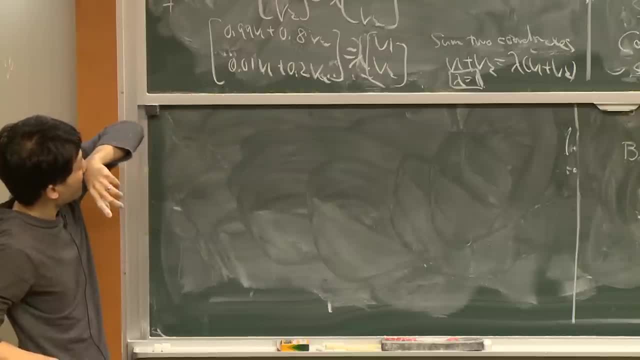 But until you get to the limit you still have them. But essentially that kind of behavior is transitionary behavior, that dissipates, But the behavior, of course, stationary distribution persists. But, as you mentioned, this argument seems to be giving that all lambda has to be 1, right. 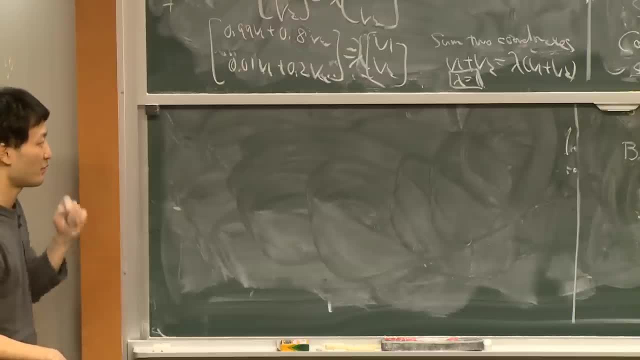 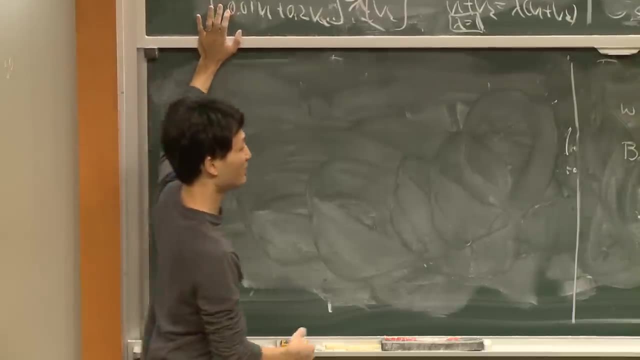 Is that your point? You're right. I don't see what the problem is, right? No, I'll think about it later. I don't want to waste my time on trying to find what's wrong, But the conclusion is right. 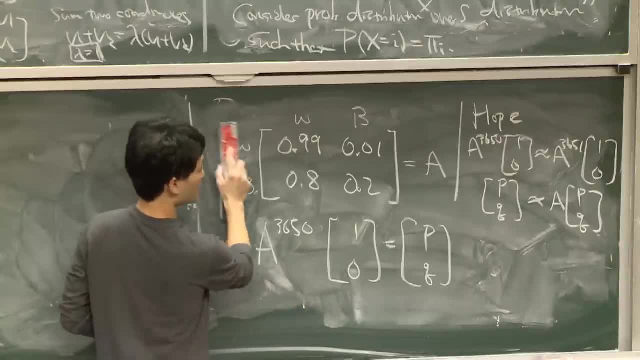 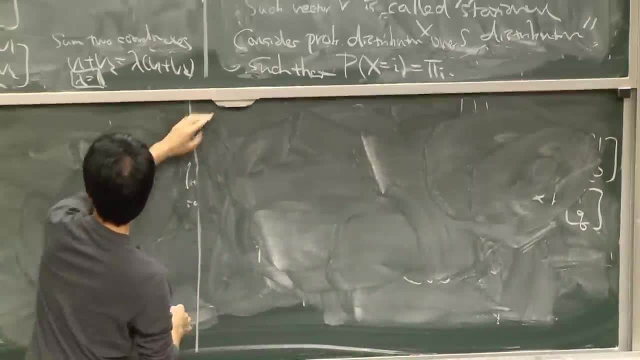 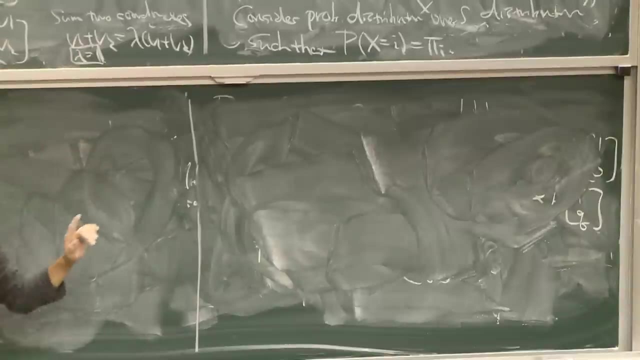 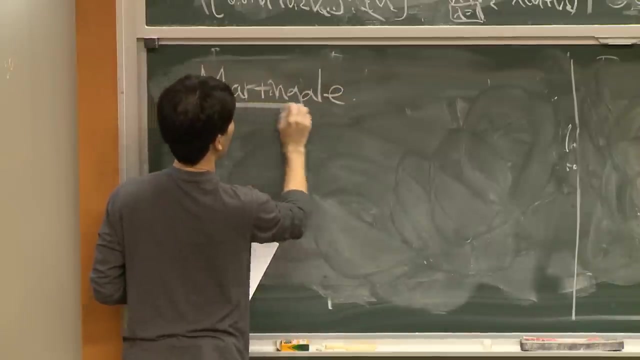 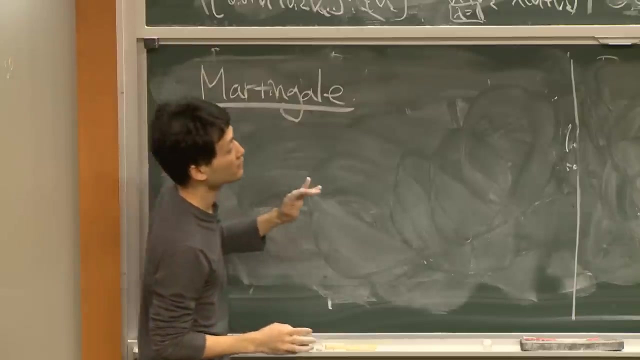 There will be a unique one, and so on. Let me make a note here, OK, So let me move on to the final topic. It's called martingale, And this is another collection of stochastic processes, And what we're trying to model here is 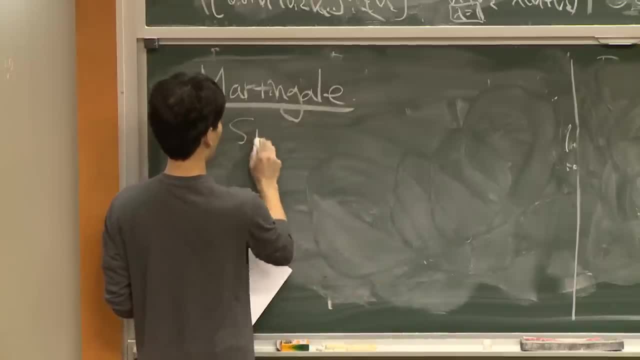 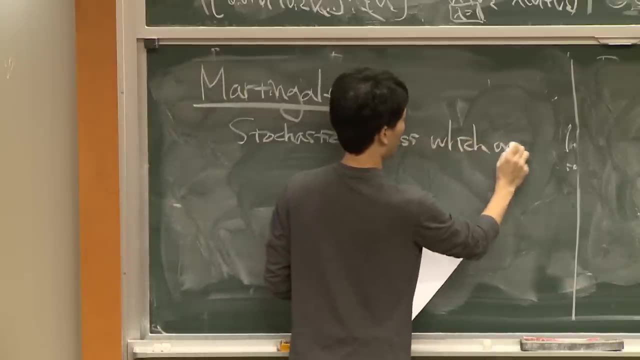 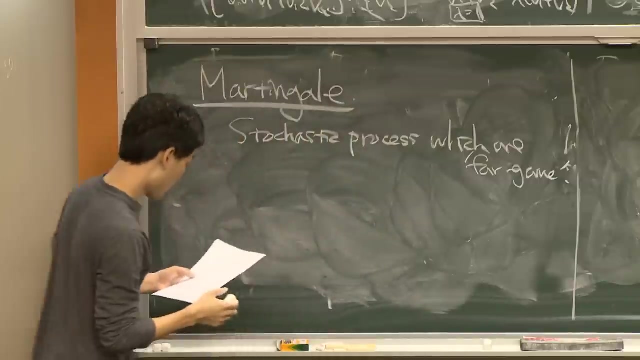 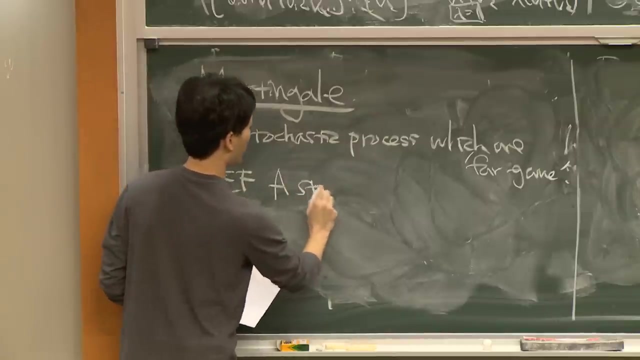 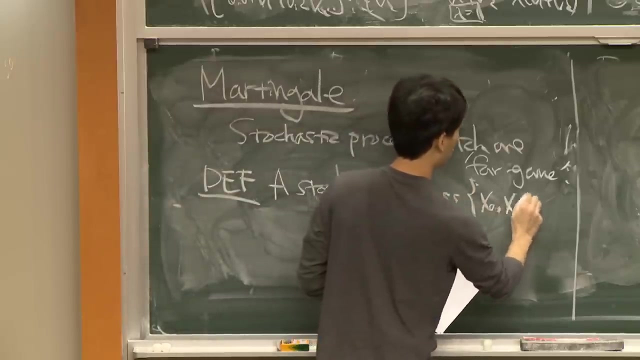 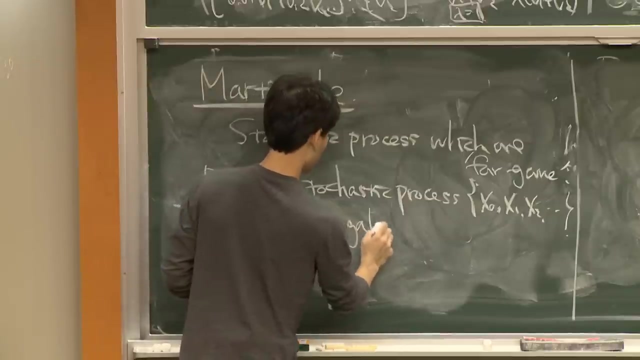 we're trying to model a fair game. stochastic processes- And formally, what I mean is a stochastic process- is we need to model a fair game. It's a game that's not going to be just a game. It's a game that's going to do some significant 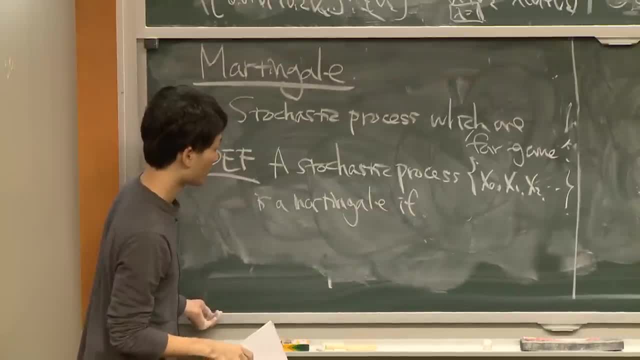 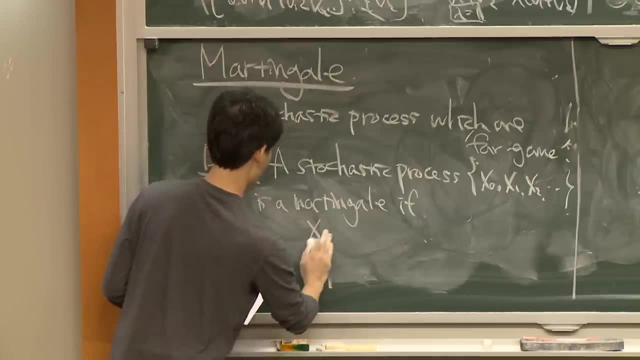 We'll talk about that later, But the idea is, if we've got f and we've got p and we've got f, And so we can do a quick analysis of what happens if we do that. And again, if we have f and we have F. 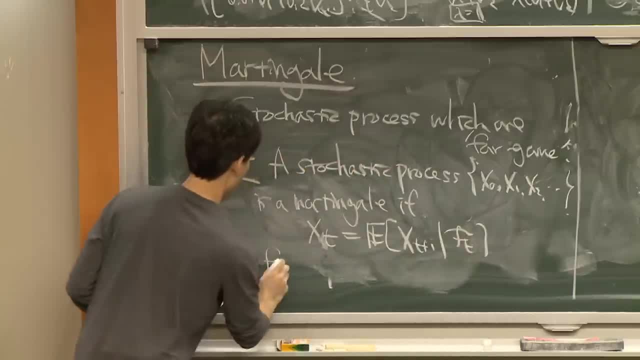 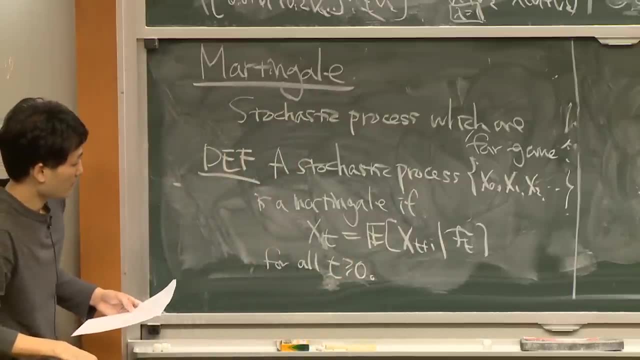 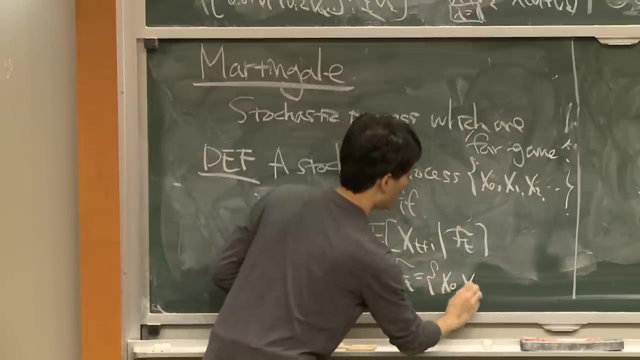 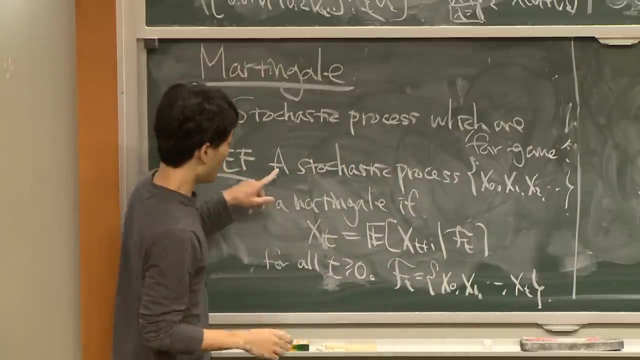 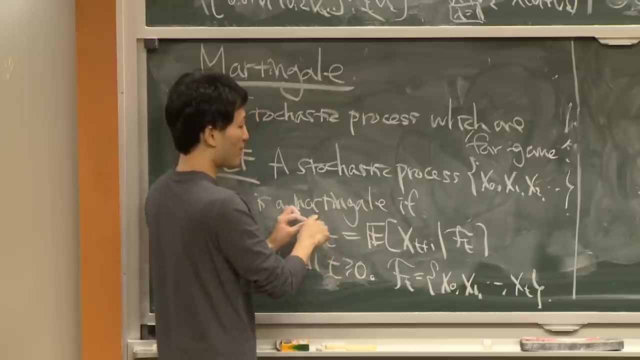 we can use the same f values to do the same thing here. If this is some random answer, then we can call this. Let me iterate it. So what we have here is, at time t, if you look at what's going to happen at time t plus 1,. 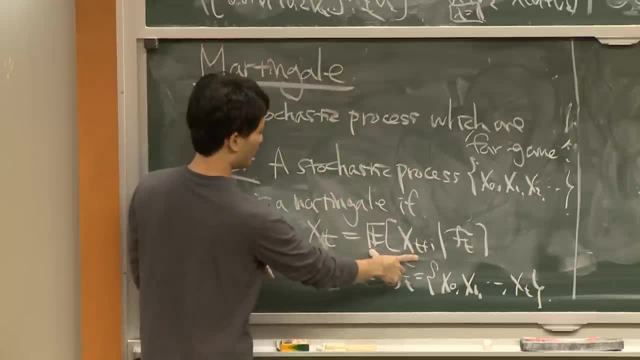 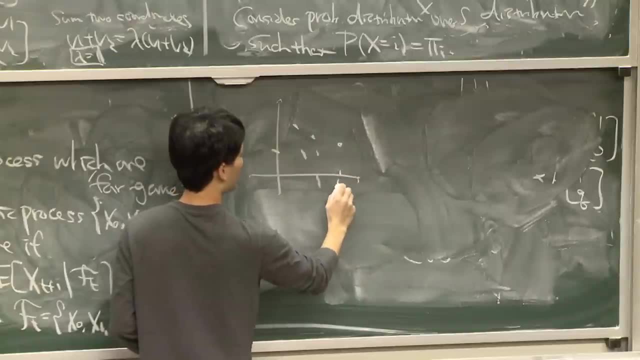 take the expectation that it has to be exactly equal to the value at xt. So you have this stochastic process And at time t you are at xt, At time t plus 1, lots of things can happen. You might go to this point, that point, that point or so on. 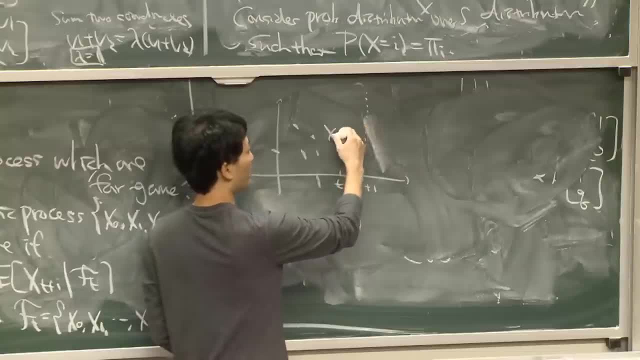 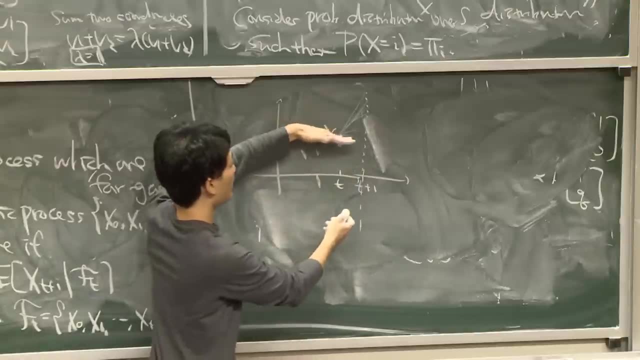 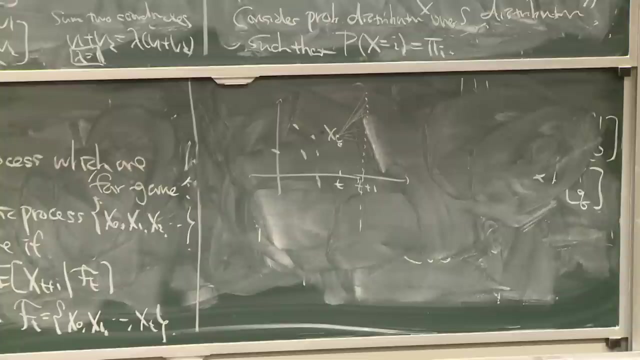 But the probability distribution is designed so that the expected value over all these points are exactly equal to the value at xt. So it's kind of centered at xt. A centered mean in the probabilistic sense, not just the expectation, is equal to that. 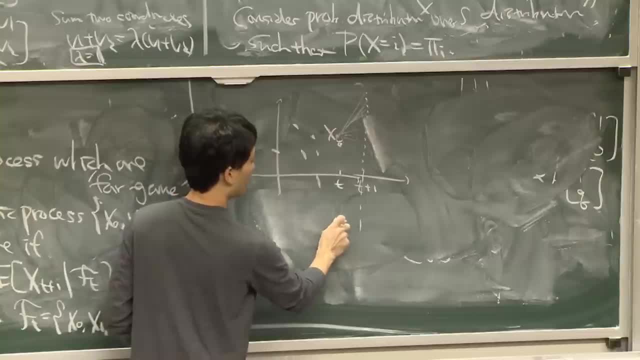 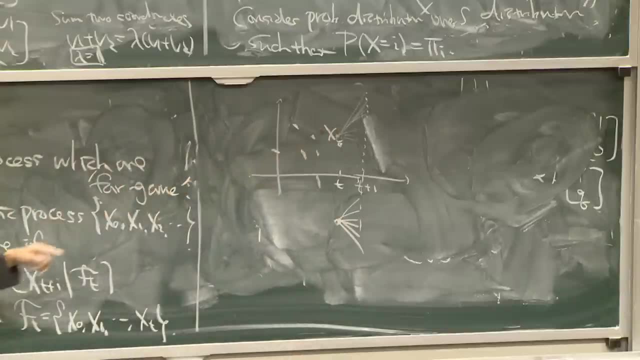 So if your value at time t was something else, your values at xt plus 1,, at time t plus 1, will be centered at this value instead of that value. And the reason I'm saying it models a fair game is because, in expectation, if this 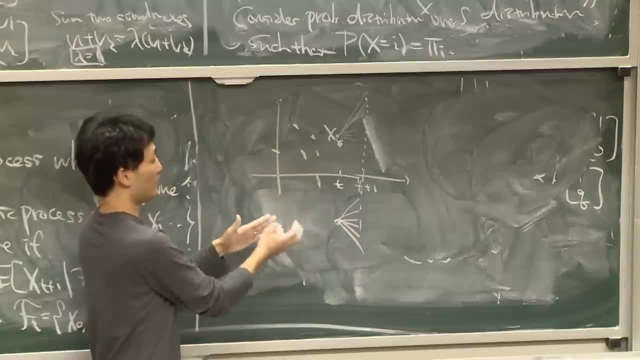 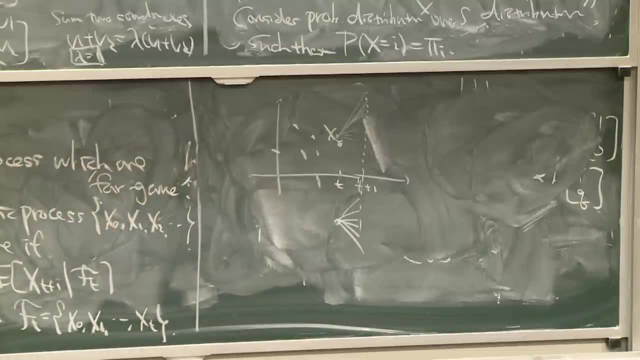 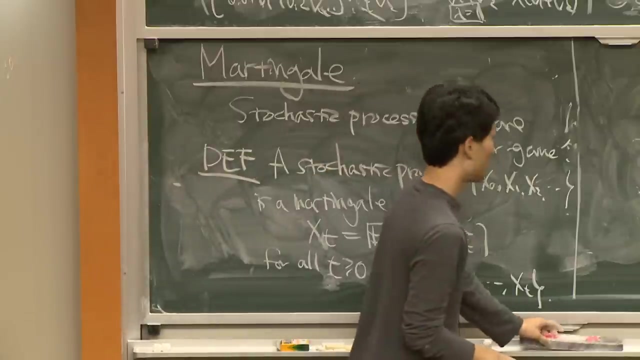 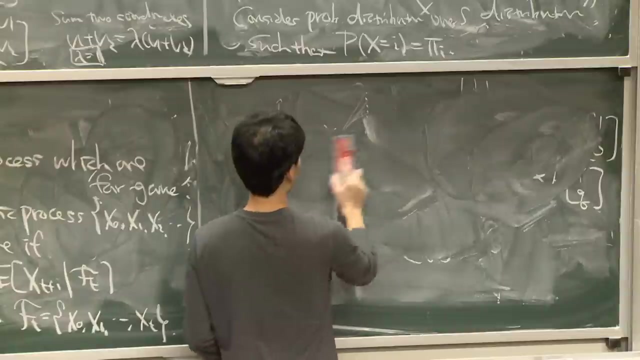 is like your balance in expectation. if it's like a balance over some game in expectation, you're not supposed to win any money at all, And I will later tell you more about that. So example: a random walk is a martingale. 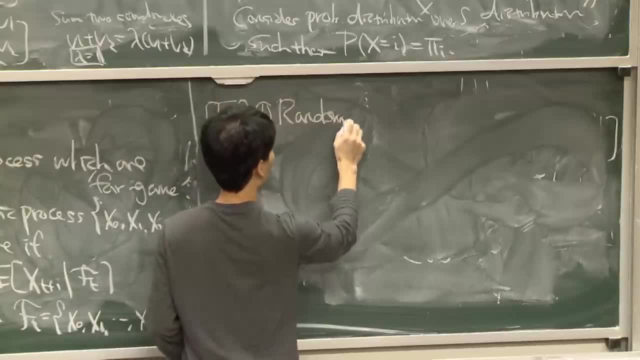 So it's a trading who to steal- And then that's dealing straight to the casino You talk about. if your hand is three times that column with a card in the blinds hat. That doesn't have to be. that's not a good trade. 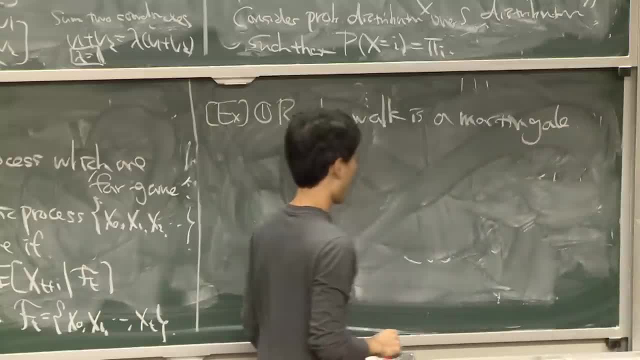 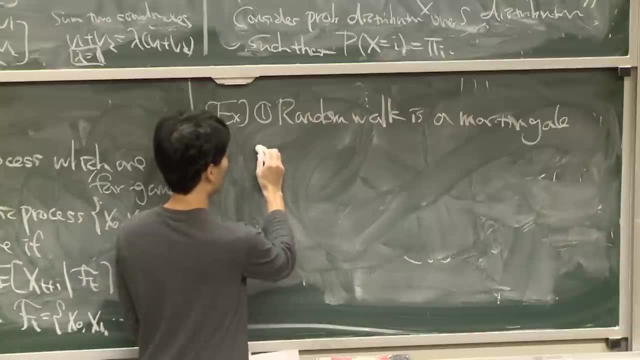 It becomes a What else? OK. second one: OK, let's say you're at the casino and you're playing roulette, Balance of roulette. Let's imagine you're in a casino, You're playing roulette, Balance of roulette. yeah. 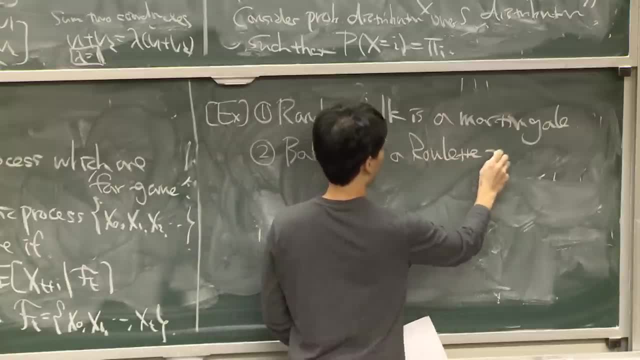 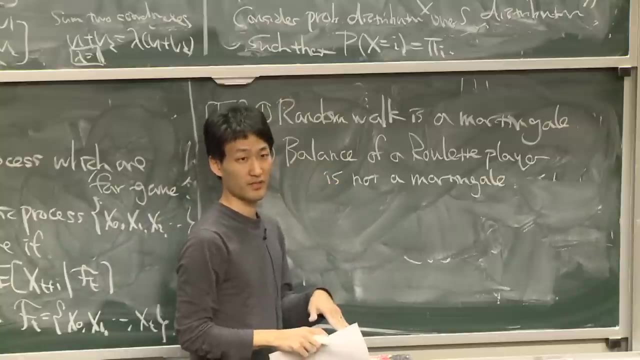 Bonus aiming. So you're playing roulette опредино. It's a solid game. Is that presentations a player is not a martingale, because it's designed so that the expected value is less than 0. You're supposed to lose money. 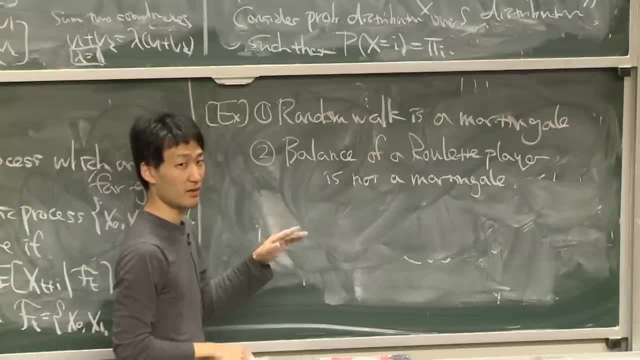 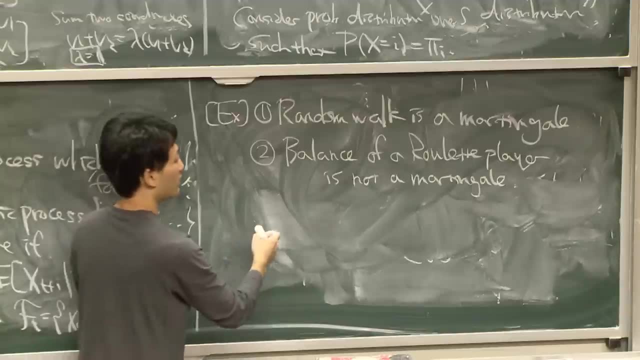 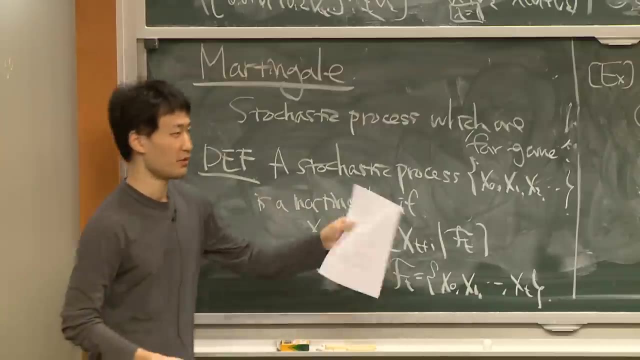 Of course, at one instant you might win money, But an expected value you're designed to go down. So it's not a martingale, It's not a fair game. The game is designed for the casino, not for you. 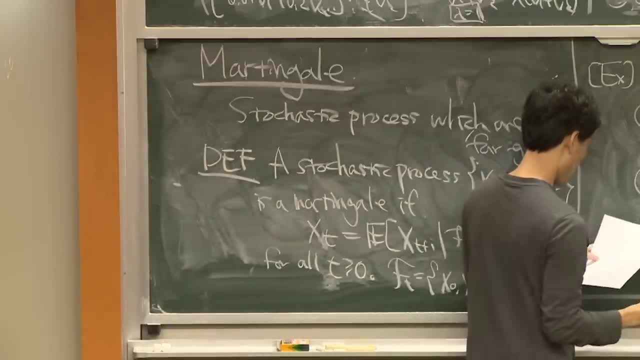 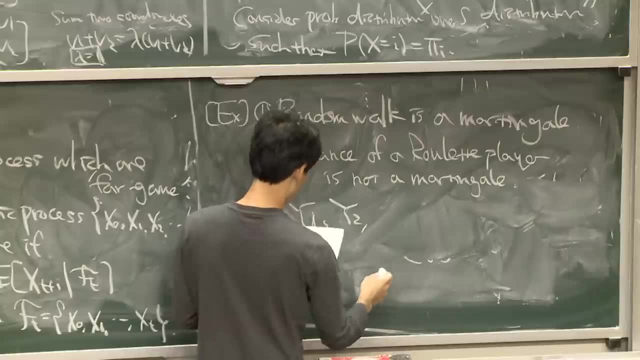 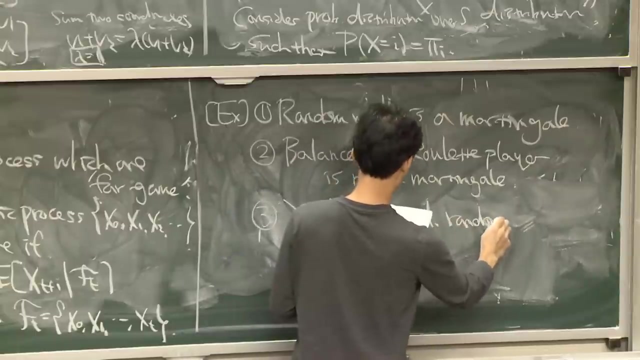 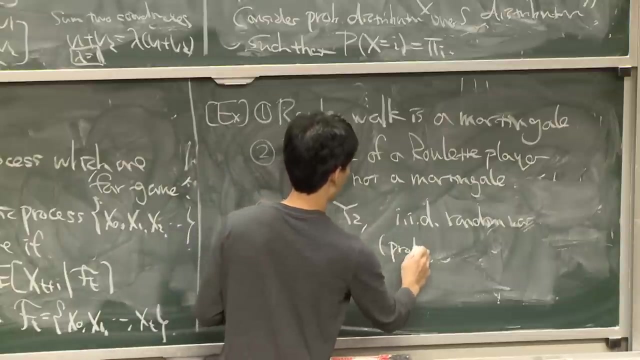 Third one is some funny example I just made it up to show that there are many possible ways that a stochastic process can be a martingale. So if yi are iid random variables, such that yi is equal to 2 with probability 1 over 3,. 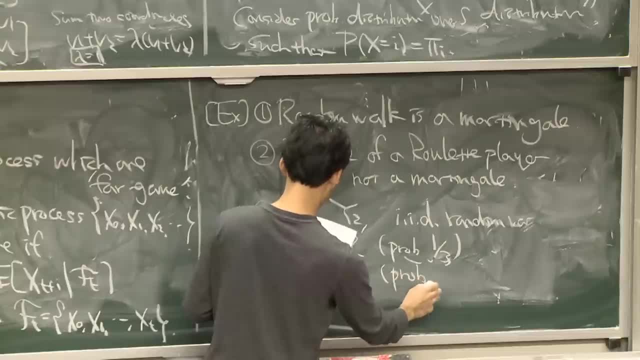 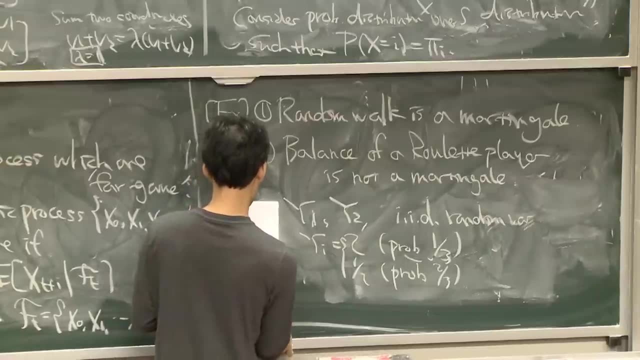 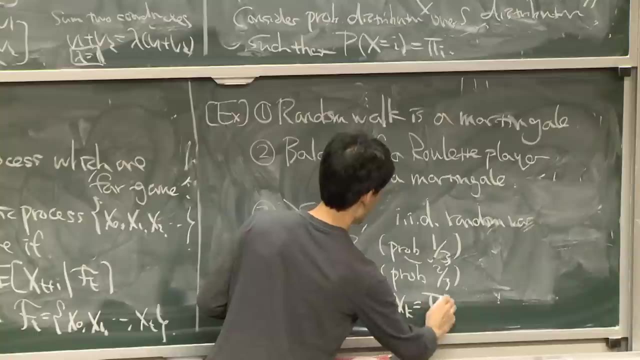 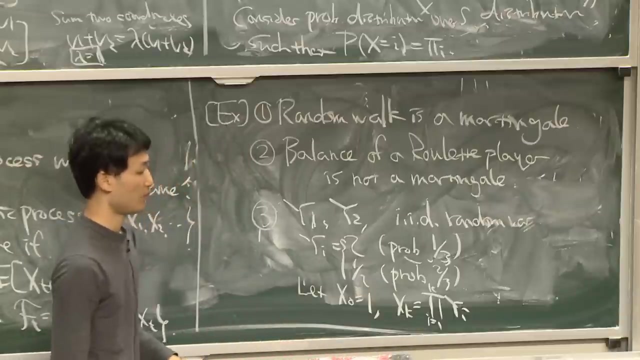 and 1 half, with probability 2: third. then let x0 equals 1, and xk equals i. Then that is a martingale. So at each step you'll either multiply by 2 or divide by 2.. And the probability distribution is given as 1. third and 2. 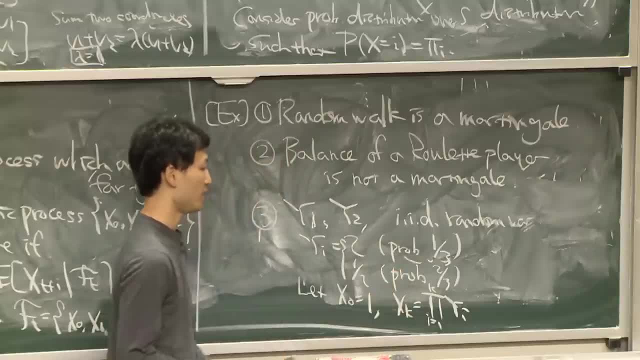 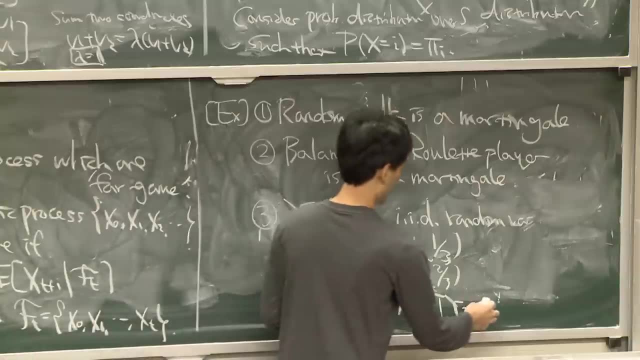 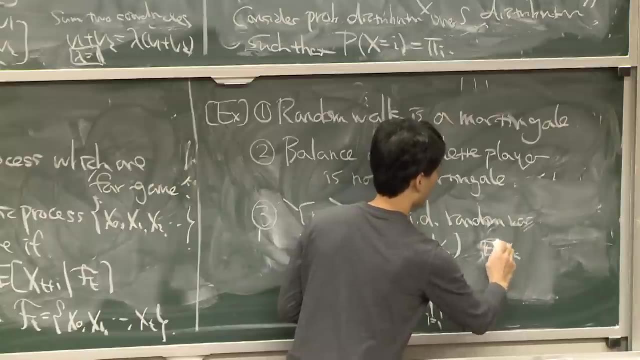 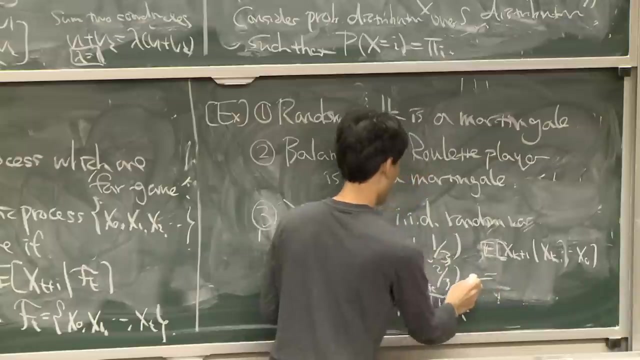 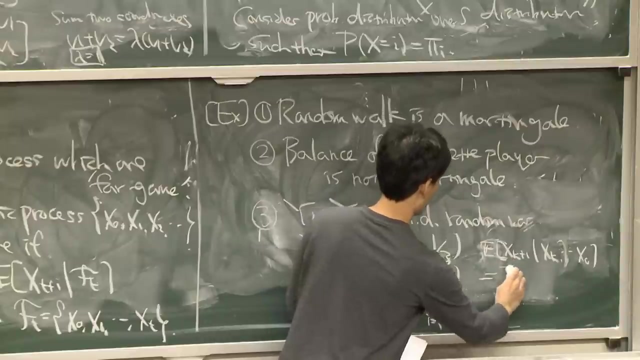 thirds, Then xk is a martingale. The reason is you can compute the expected value. The expected value, The expected value of xk plus 1, given xk up to x0, is equal to what you have is expected value of yk plus 1. 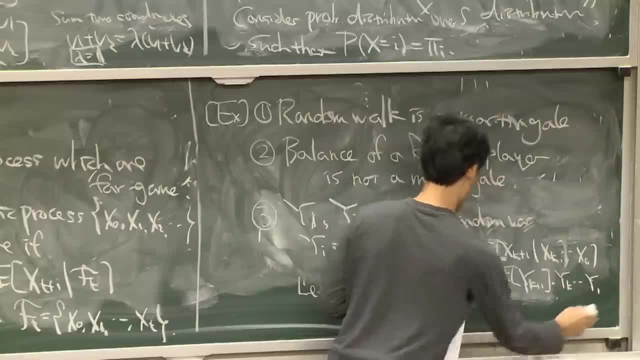 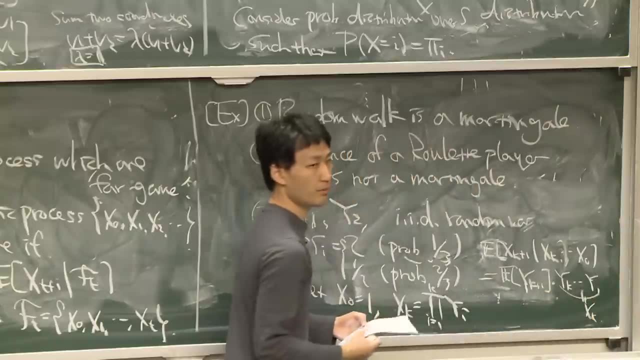 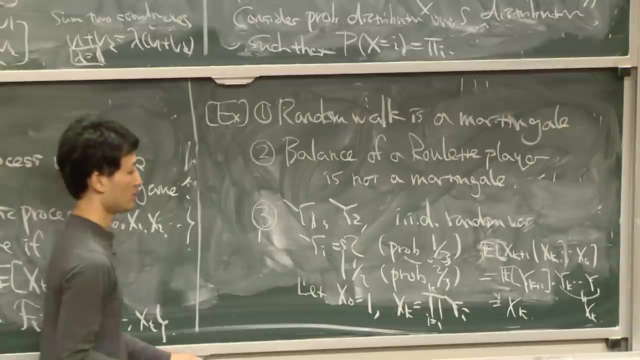 times yk up to 1.. That part is xk, But this is designed so that the expected value is equal to 1.. So it's a martingale. I mean it will fluctuate a lot your balance. Double, double, double, half, half, half and so on. 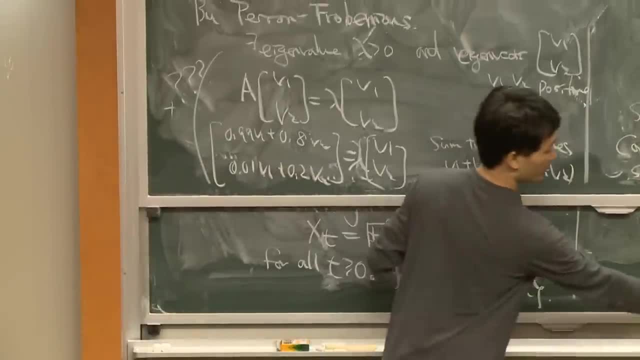 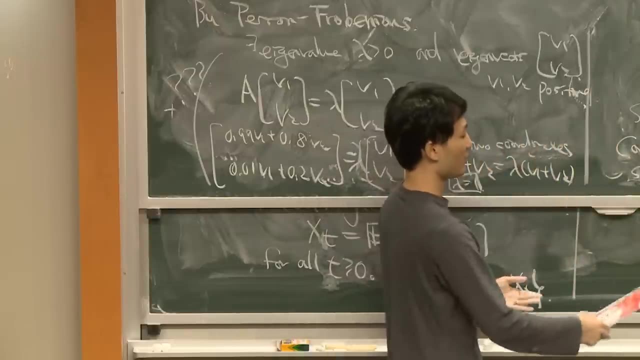 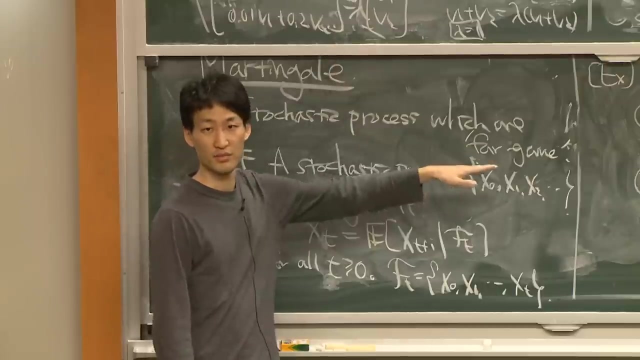 But still An expectation you will always maintain. I mean, the expectation at all time is equal to 1. if you look at it from the beginning, Look at time 1,, then the expected value is x1, and so on. Any questions on definition or example? 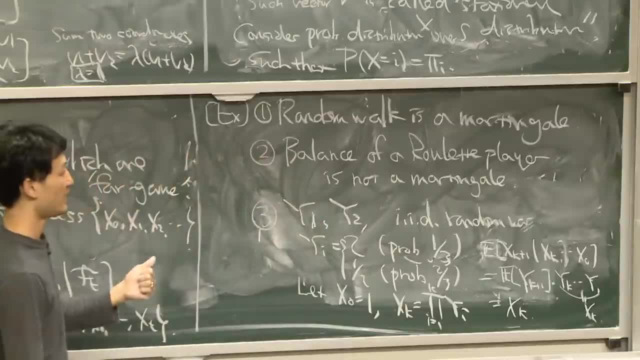 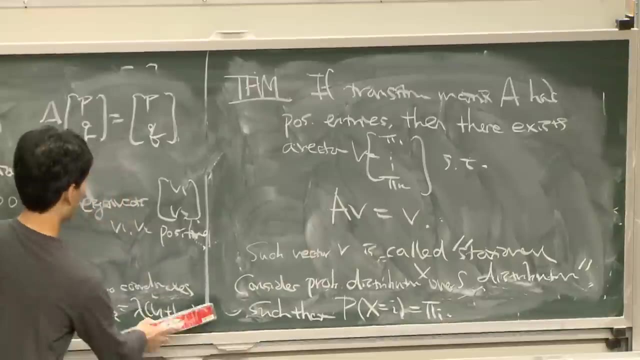 So the random walk is an example which is both Markov chain and martingale, But these two concepts are really two different concepts. Try not to be confused between the two. They're just two different things. There are Markov chains which are not martingale. 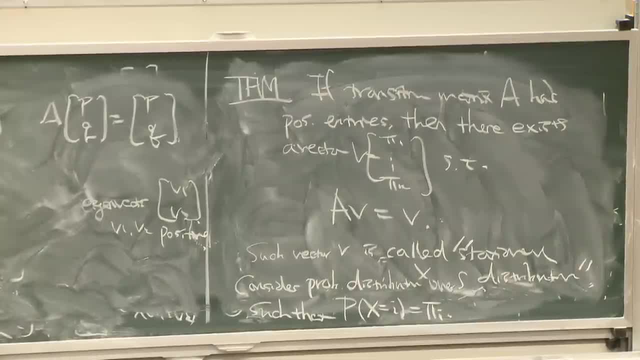 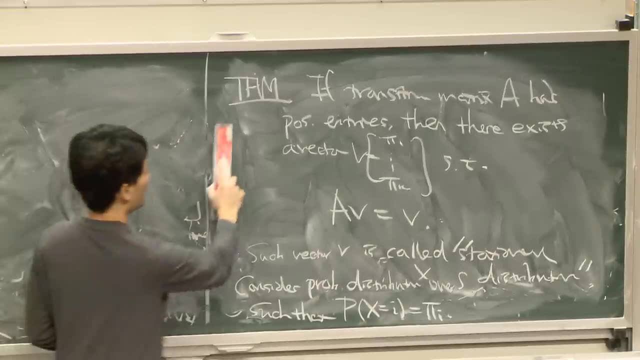 There are martingales which are not Markov chain And there are something which are both like simple random walk. There are some stuff which are not either of them. They really are just two separate things, Thank you. Thanks, You're welcome. 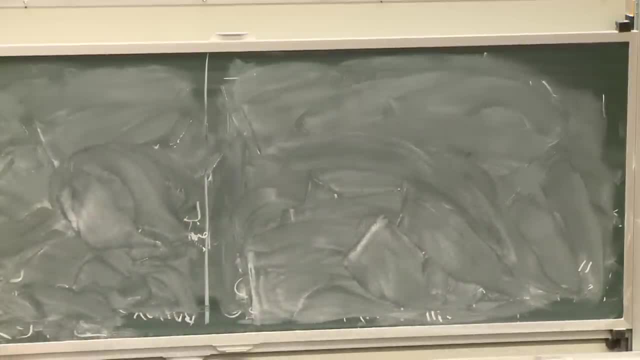 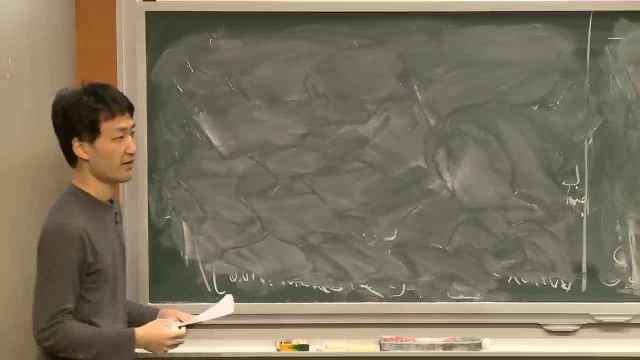 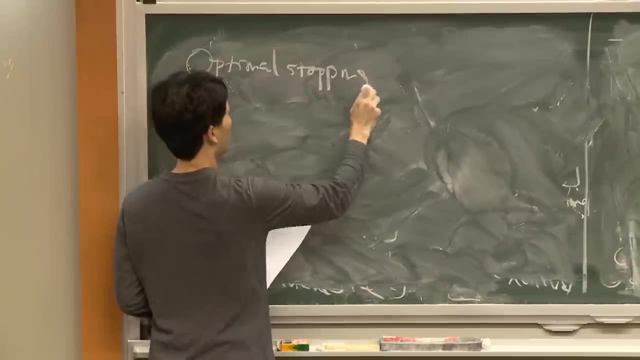 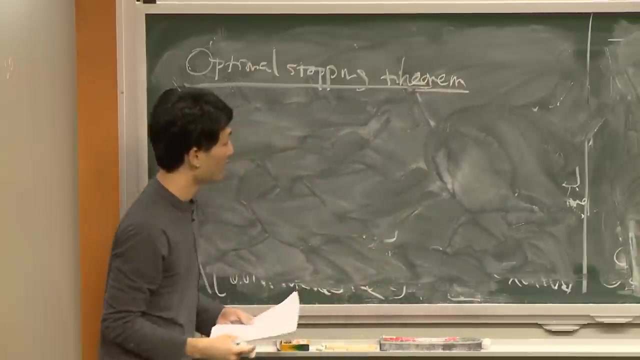 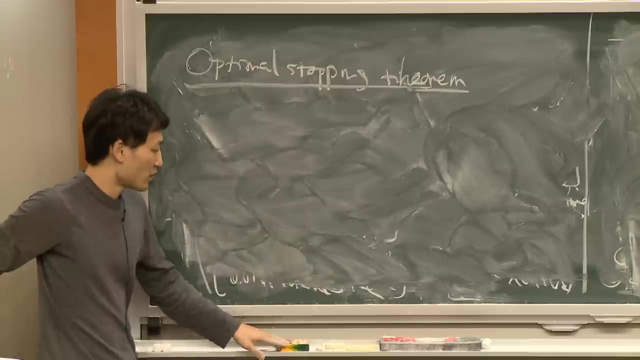 intuition of the definition that martingale is a fair game. It's called Optional Stopping Theorem And I will write it down more formally later. But what it says is the message is this: If you play a martingale game, if it's a game you play and 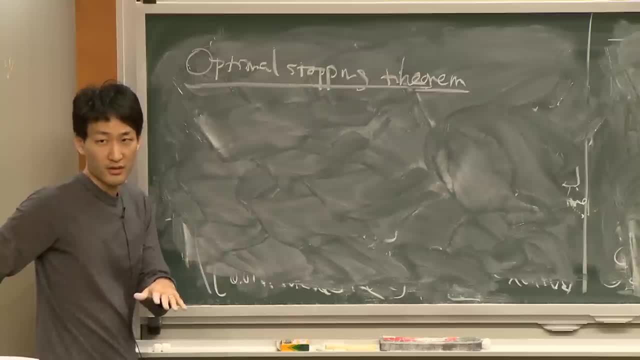 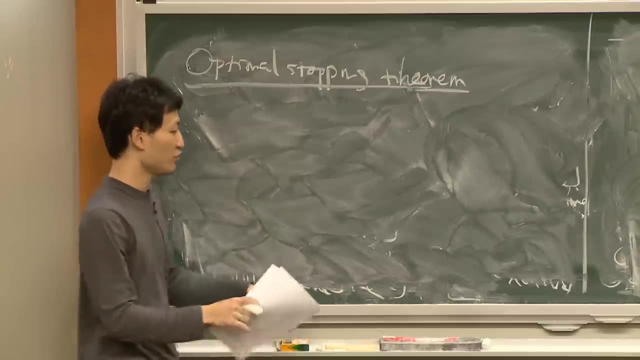 it's your balance. no matter what strategy you use, your expected value cannot be positive or negative. Even if you try to lose money so hard, you won't be able to do that. Even if you try to win money so hard like try to invent. 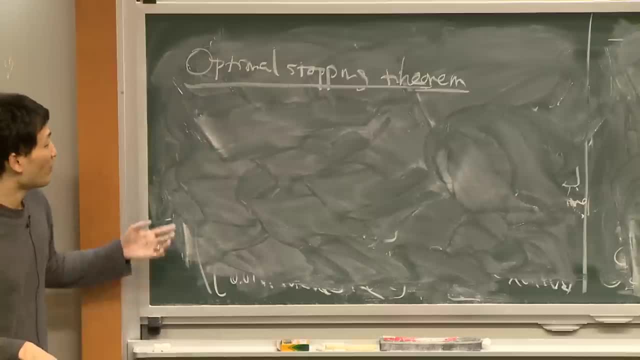 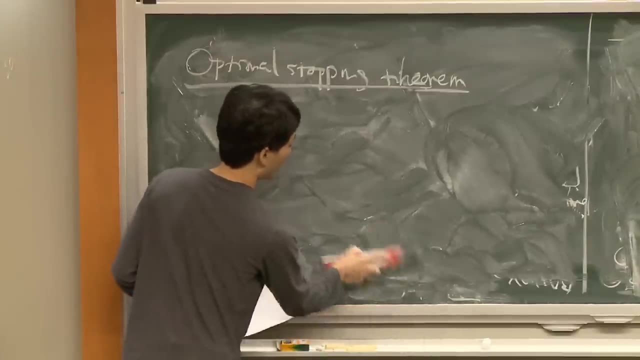 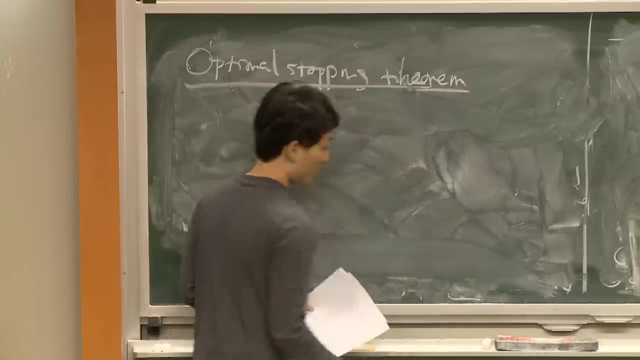 something really, really cool and genius. you should not be able to win money. Your expected value is just fixed. That's the content of the theorem. Of course, there are some technical conditions that have to be there. So if you're playing a martingale game, then you're. 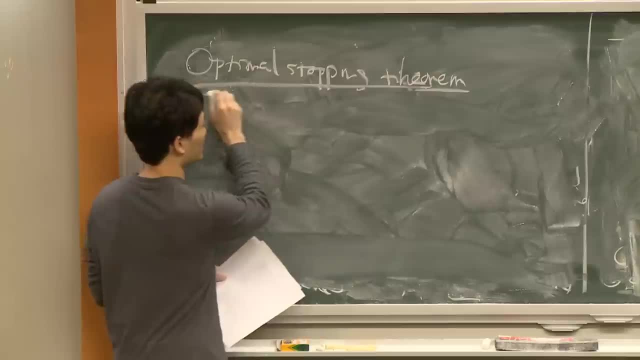 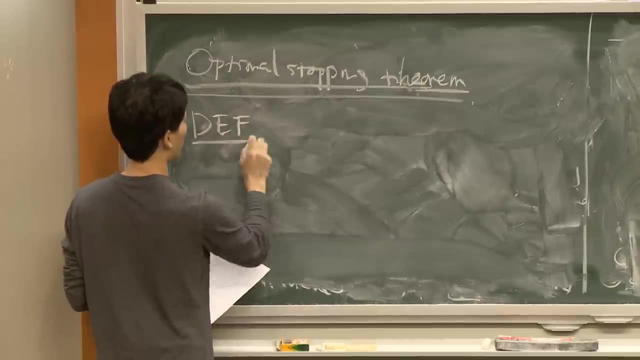 not supposed to win or lose, at least in expectation. So before stating the theorem, I have to define what a stopping time is. It's one of those things that you can do by using a over-the-top formula to solve that. So you need a step. 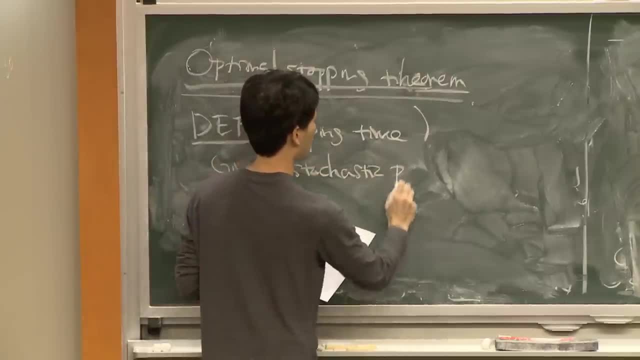 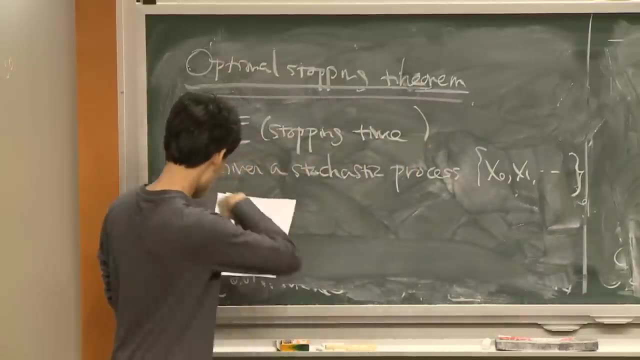 If it's a step, it's a move, It's a move And it's a move, It's a move, Then a step, It's a move. It's going to be one, two, three, okay, And then you need a stop. 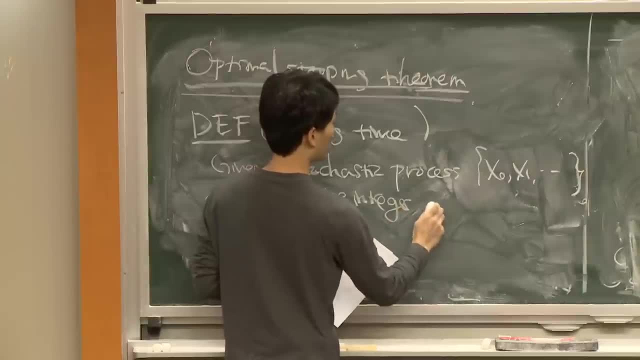 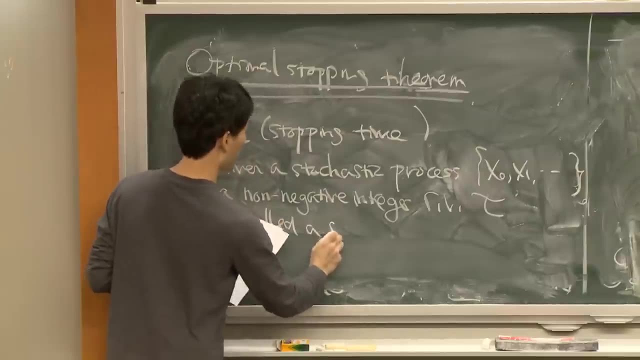 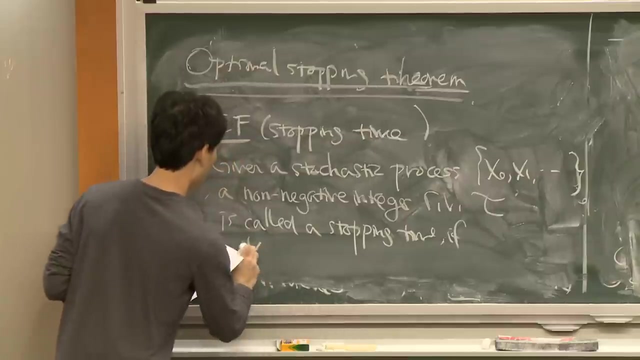 You have a couple of steps that you have to make, So maybe it's first step, Or it could be second step. Okay, So, given a stochastic process, tau is called a stopping time if for all integer k is equal to 0,. 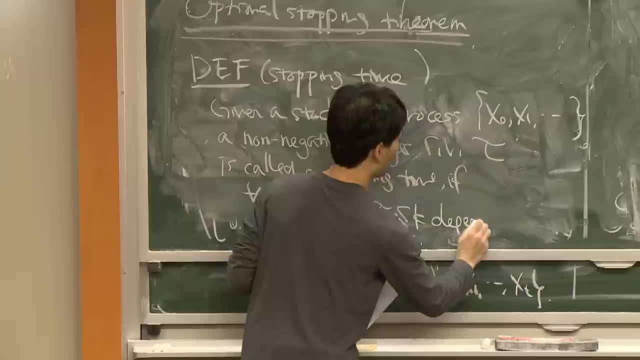 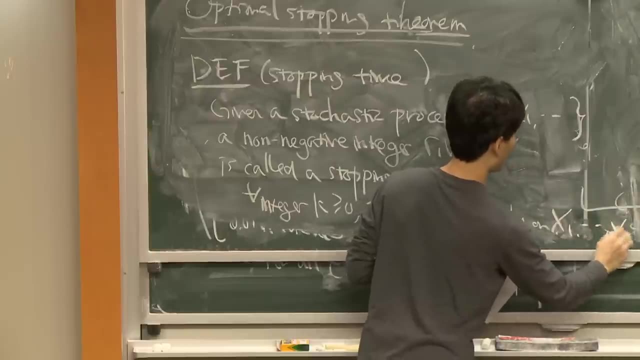 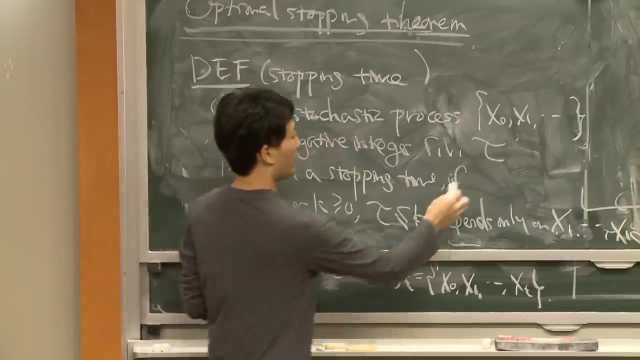 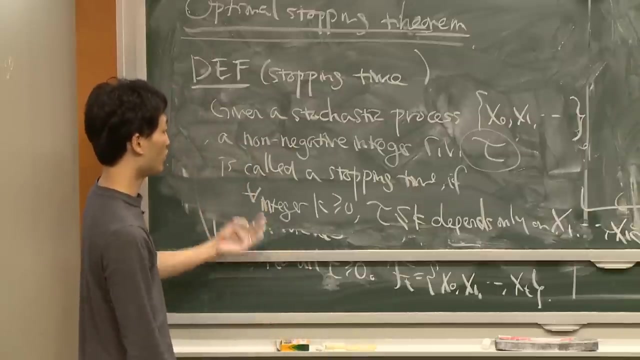 tau less than or equal to k depends only on x1 of xk. OK, that is something very, very strange. I want to define something called a stopping time. It will be a non-negative, integer-valued random variable, So it will either be 0,, 1,, 2, or so on. 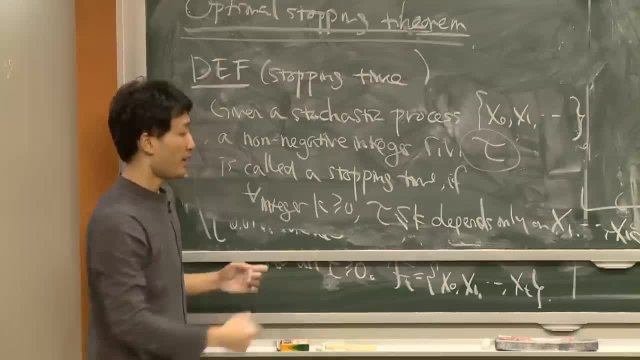 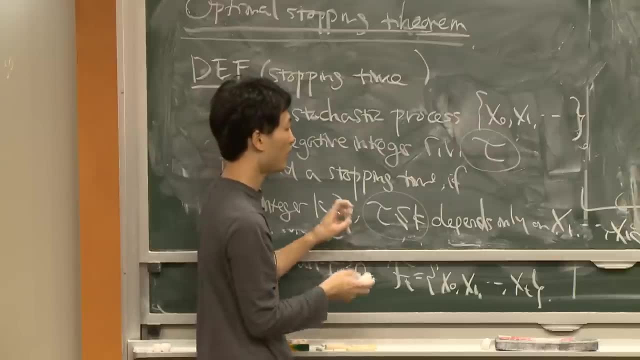 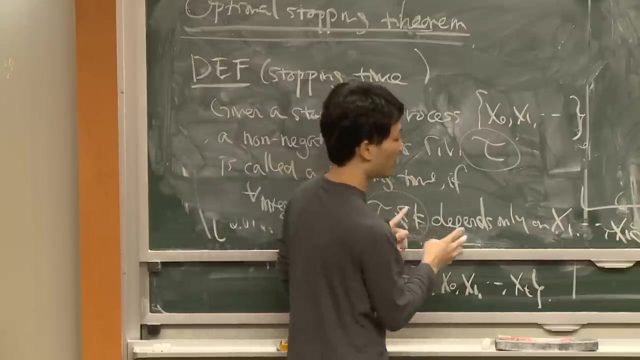 That means there will be some time index And if you look at the event, that tau is less than or equal to k. so if you want to look at the events when you stop at time, less than or equal to k, Your decision only depends on the events up to k. 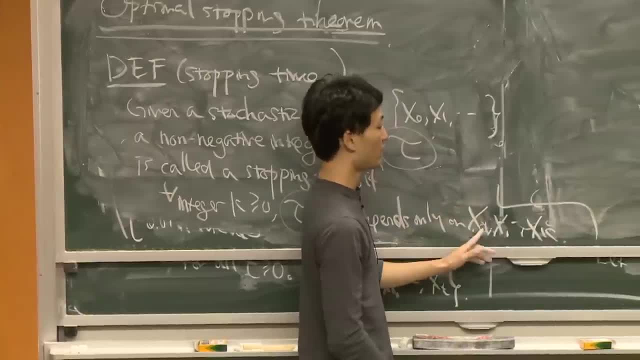 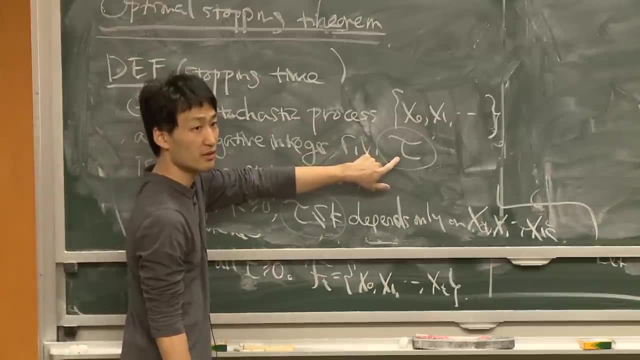 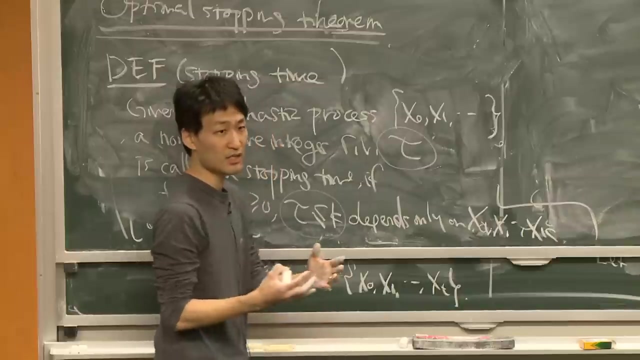 on the stochastic processes, the value of the stochastic process up to time k. In other words, if this is some strategy you want to use. by strategy I mean some strategy that you stop playing at some point. You have a strategy that is defined as you stop playing. 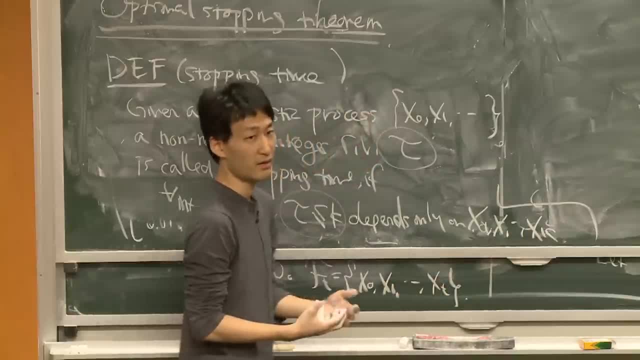 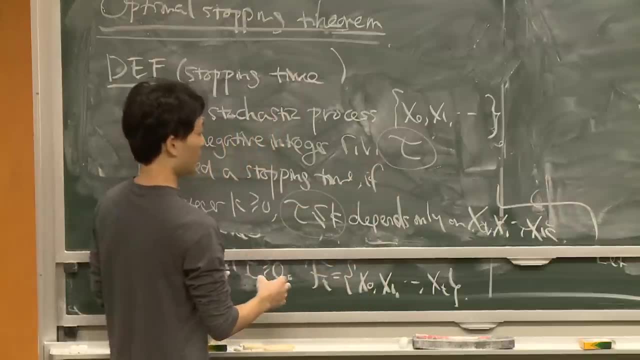 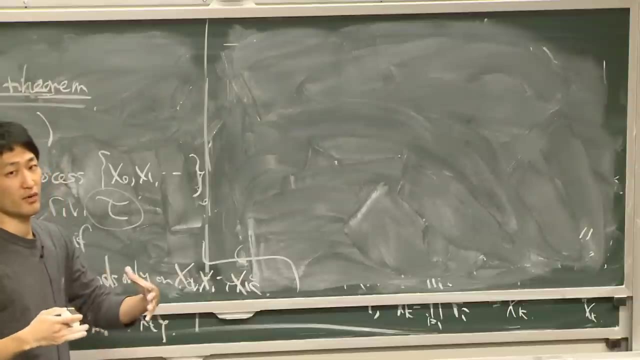 You play some k rounds and then you look at the outcome. You say, OK, now I think it's in favor of me, I'm going to stop. You have a predefined set of strategy, And so if that strategy only depends on the values of the stochastic process up to right now, 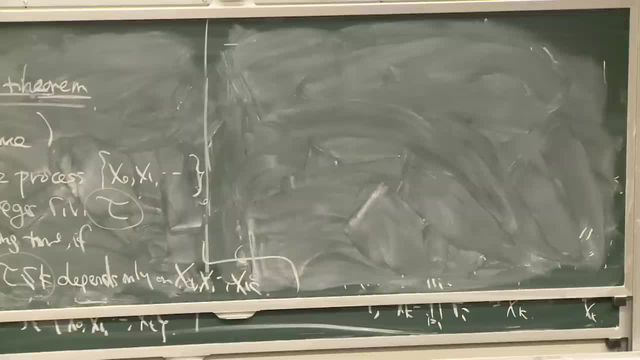 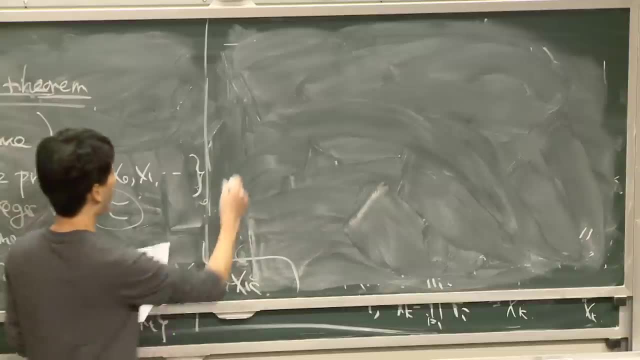 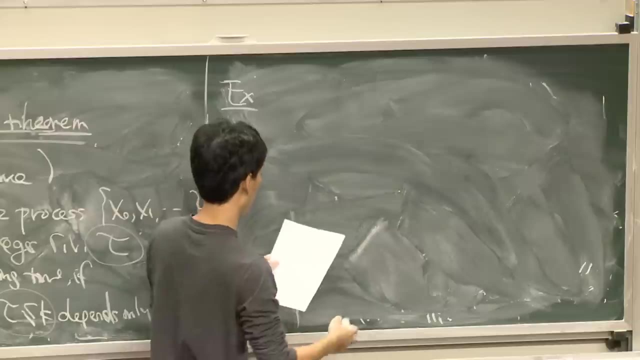 then it's a stopping time. If it's some strategy that depends on future values, it's not a stopping time. Let me show you by example. Remember that coin toss game which had random walk value. So you either win $1 or lose $1.. 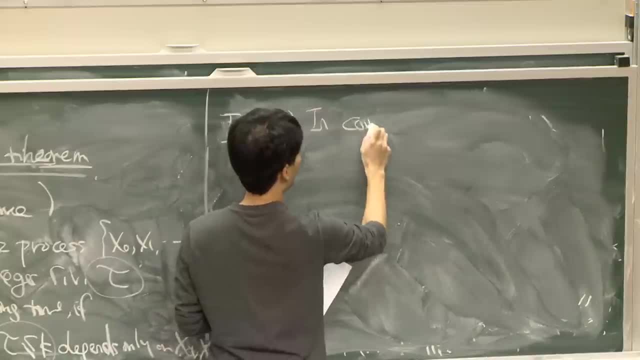 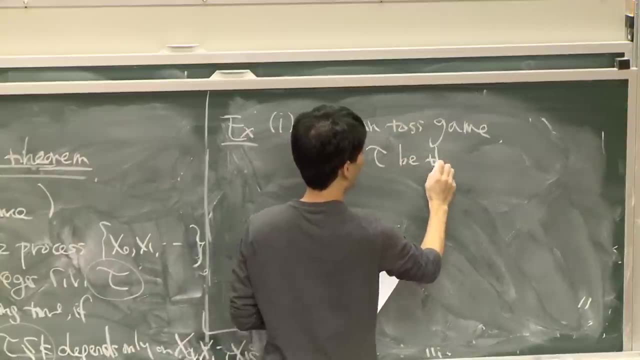 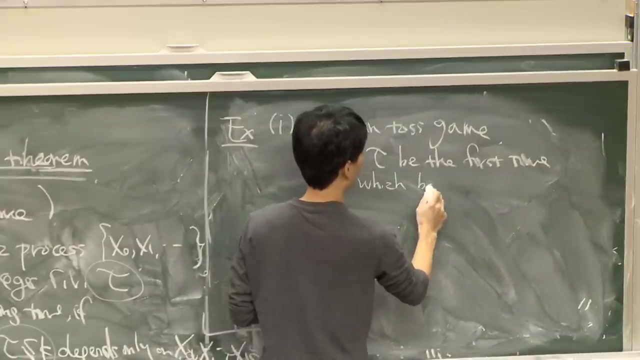 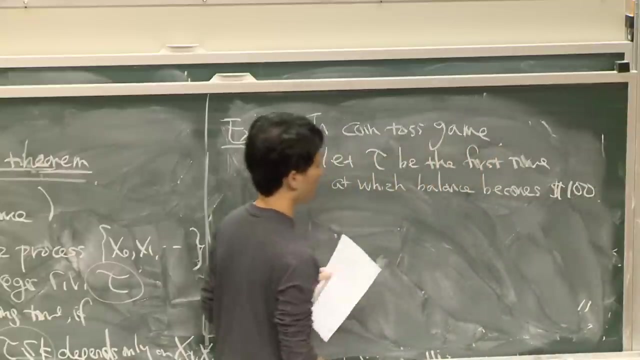 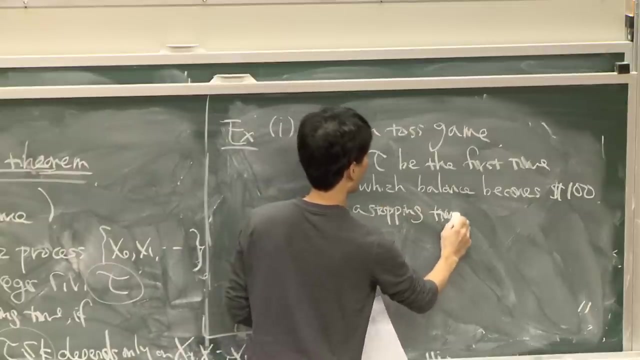 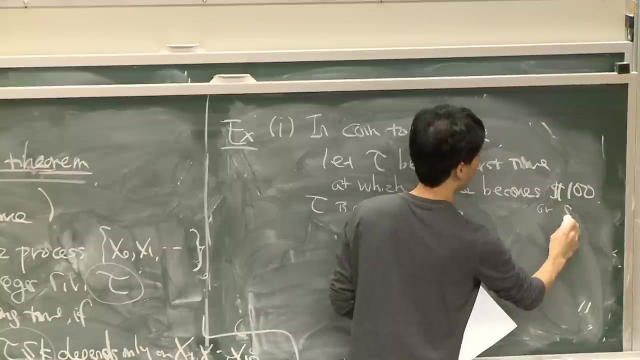 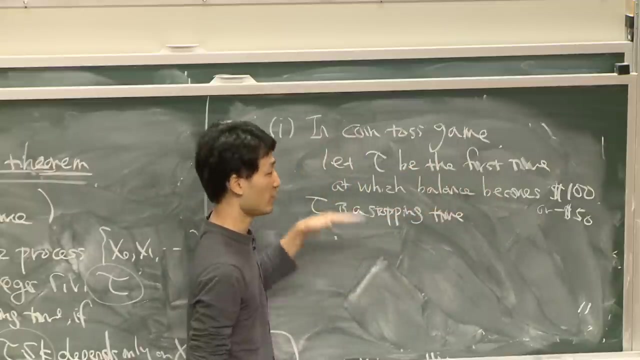 So in the coin toss game, let tau be the first time at which balance becomes under $1. Then tau is a stopping time. Or you stop at either $100 or negative $50.. That's still a stopping time. Remember that we discussed about it, that we look at our balance. 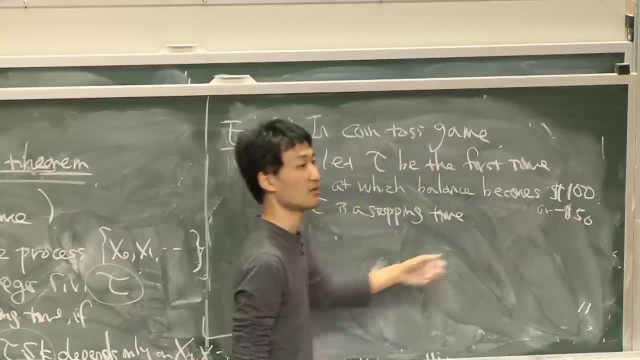 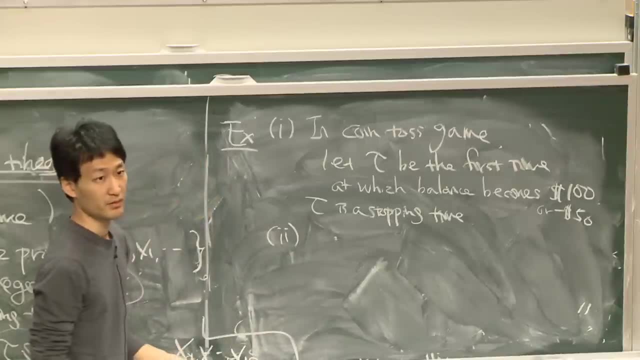 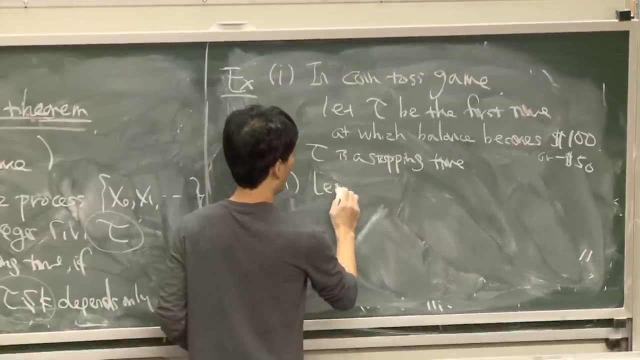 We stop either at the time when we win $100 or lose $50.. That is a stopping time, But I think it's better to tell you what is not a stopping time, for example. That will help really. So let tau in the same game, let. 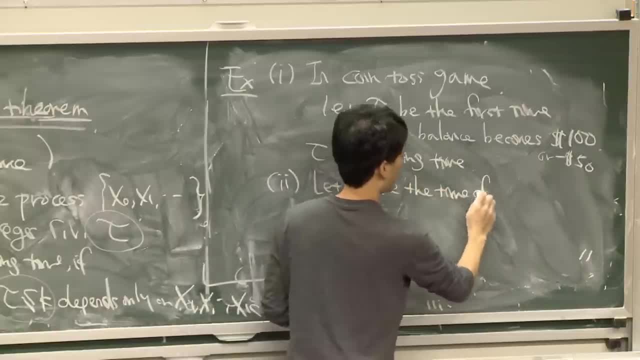 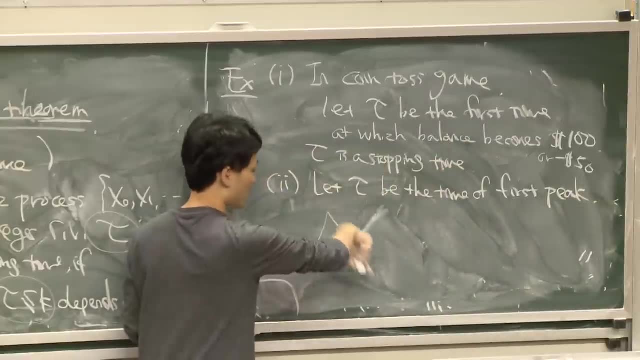 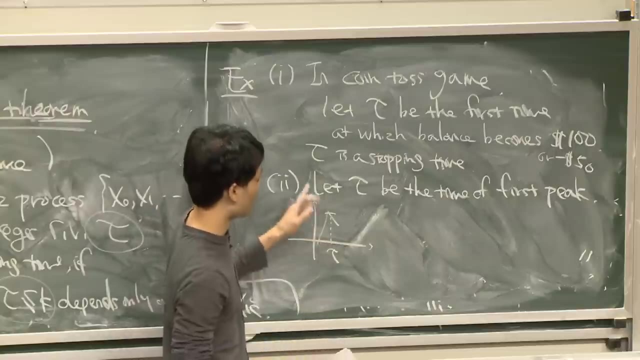 tau be the time of first peak. By peak, I mean the time when you go down. So that will be your time. So the first time when you start to go down, you're going to lose $100.. The second time when you start to go down, you're going to stop. 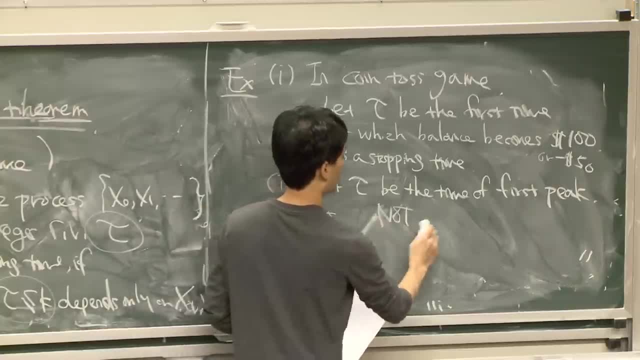 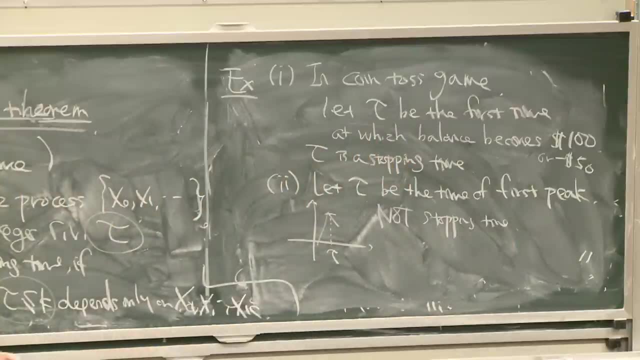 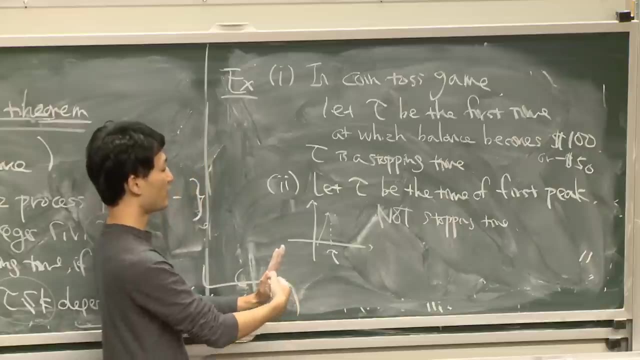 That's not a stopping time. Not a stopping time To see formally why it's the case. first of all, if you want to decide if it's a peak or not at time t, you have to refer to the value at time t plus 1.. 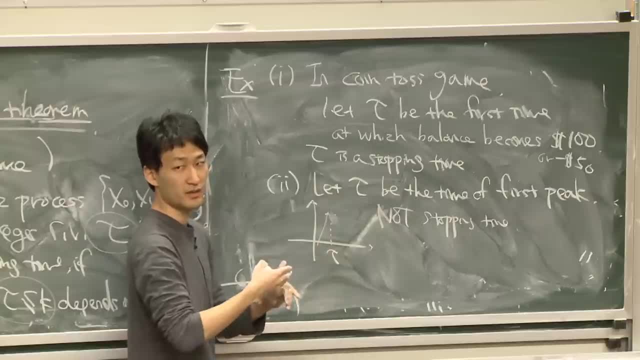 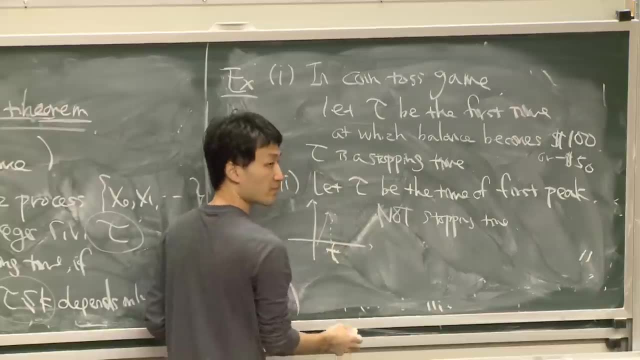 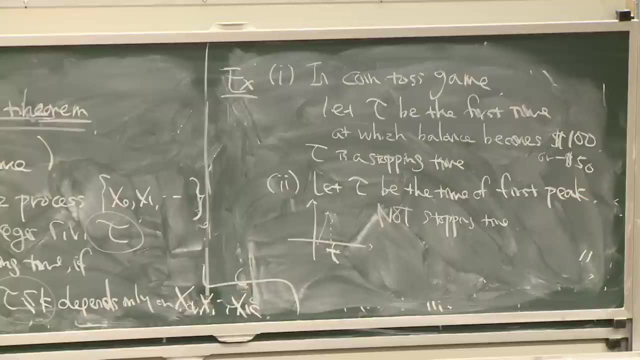 If you're just looking at values up to time t, you don't know if it's going to be a peak or if it's going to continue. The event that you stop at time t depends on t plus 1, as well, which doesn't fall into this definition. 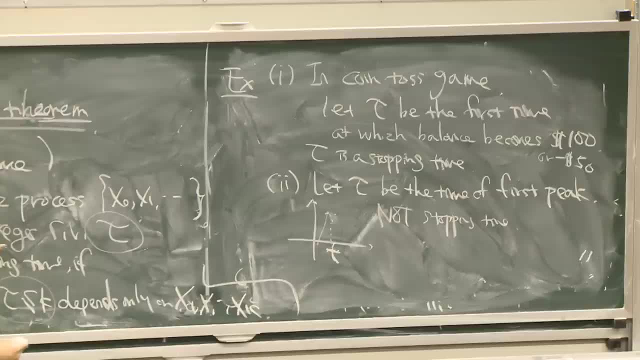 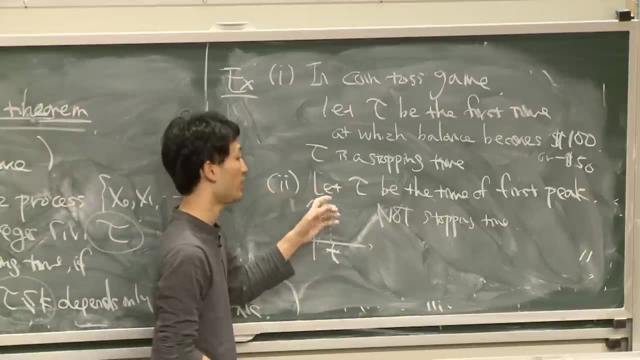 That's what we're trying to distinguish by defining a stopping time. In these cases, it was clear At some time you know if you have to stop or not. But if you define your stopping time in this way and not stopping time, if you define tau in this way, 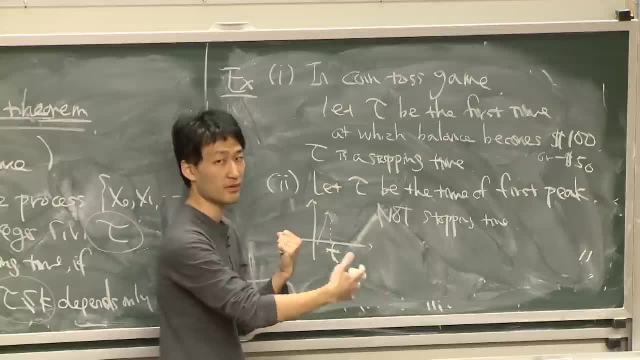 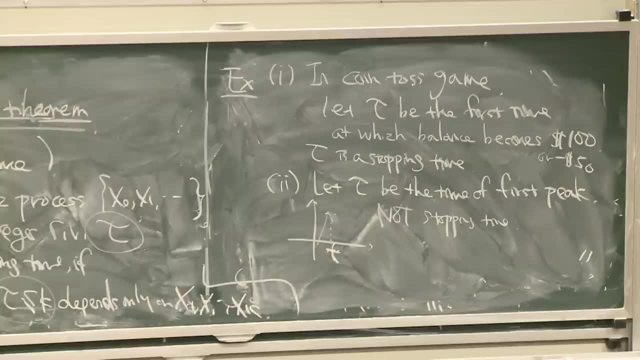 your decision depends on future values of the outcome. OK, OK, So it's not a stopping time under this definition. Any questions? Does it make sense? Yes, Could you still have tau as a stop time if you were referring to t and then t minus 1? 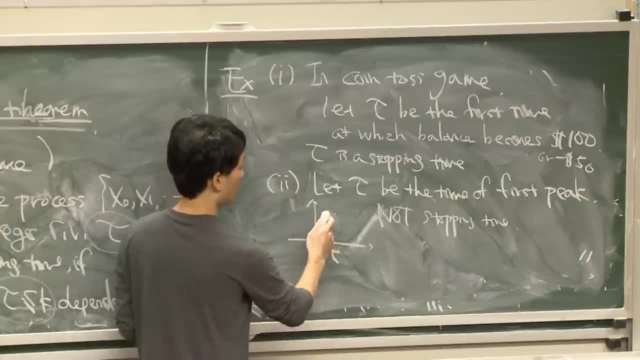 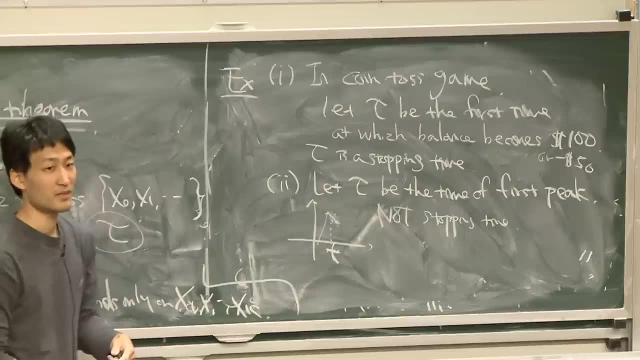 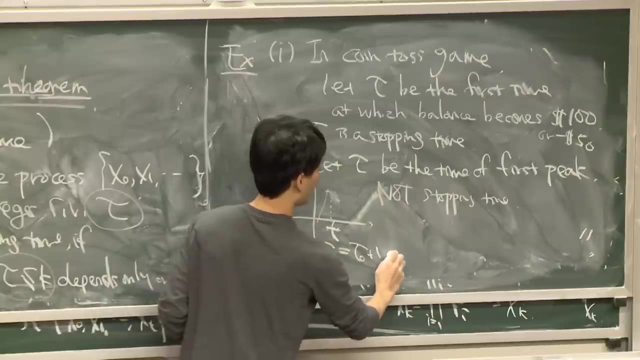 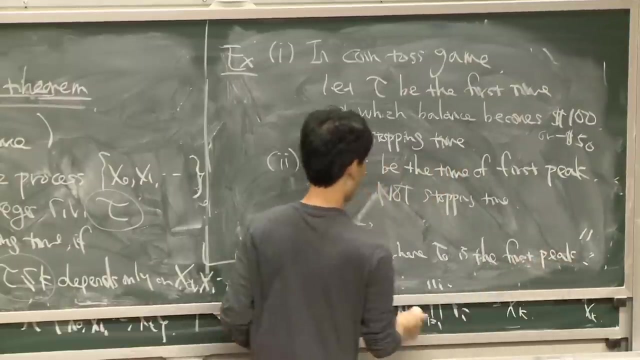 was greater than t. Oh, so time after peak, The first time after peak. yes, that will be a stopping time. So three. So if time is tau 0 plus 1, where tau 0 is the first peak, then it is a stopping time. 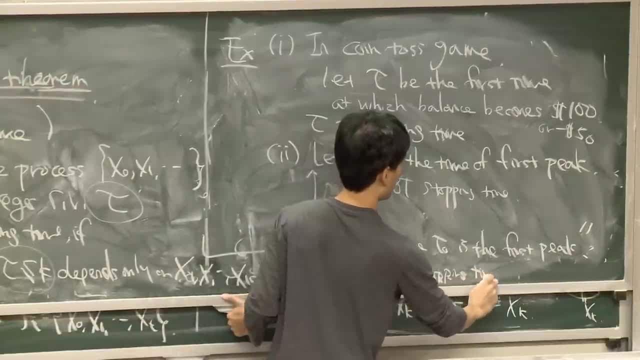 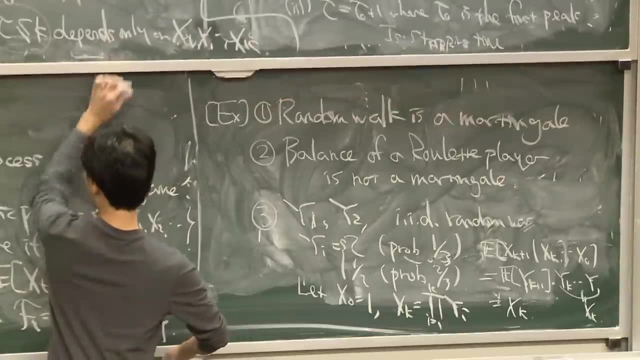 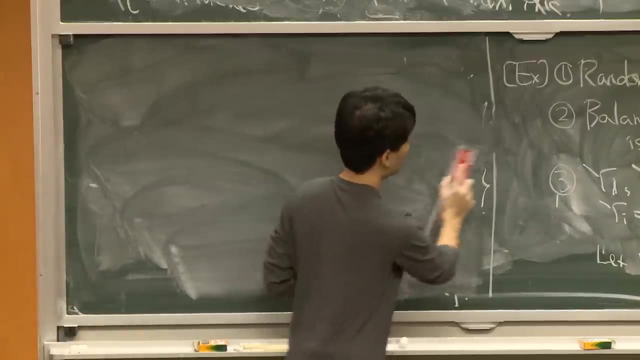 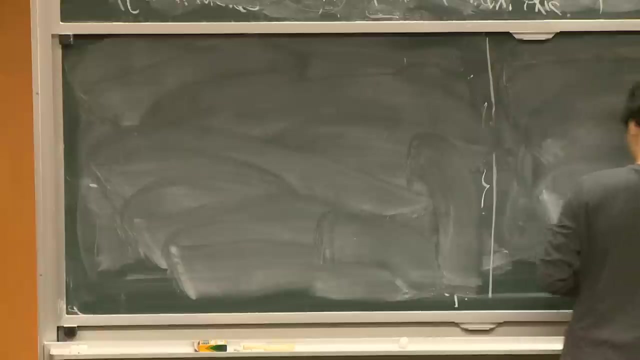 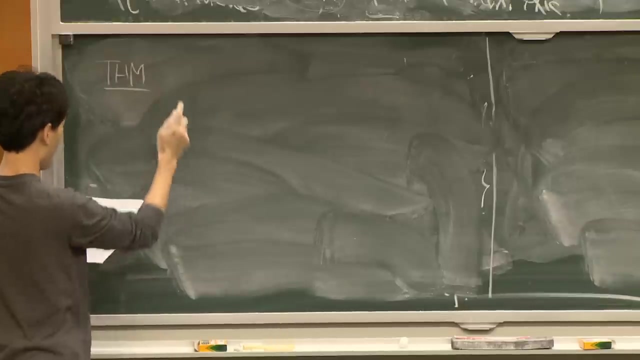 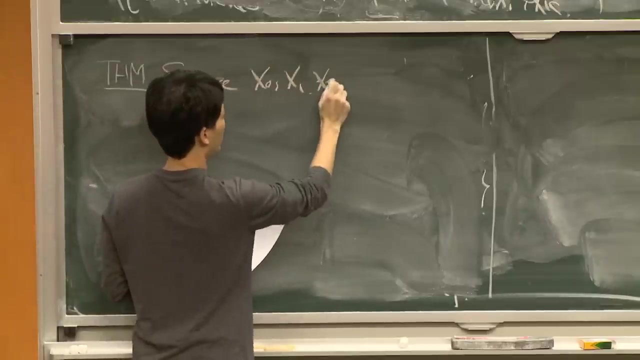 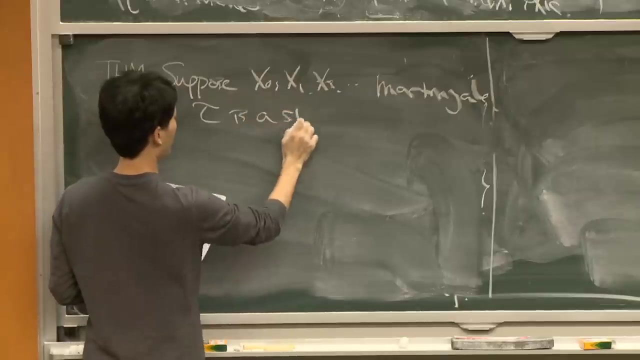 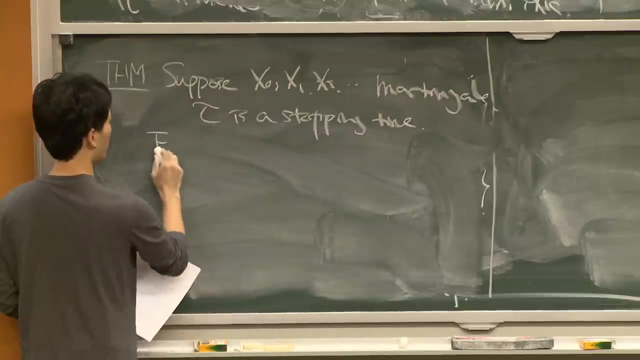 Is a stopping time. So as t's greater, it's a stopping time. OK, So the optional stopping theorem that I promised? that's a problem. Suppose we have a martingale Martingale And further suppose that furthermore, 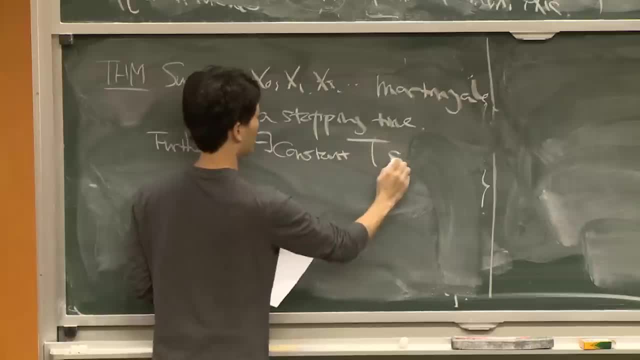 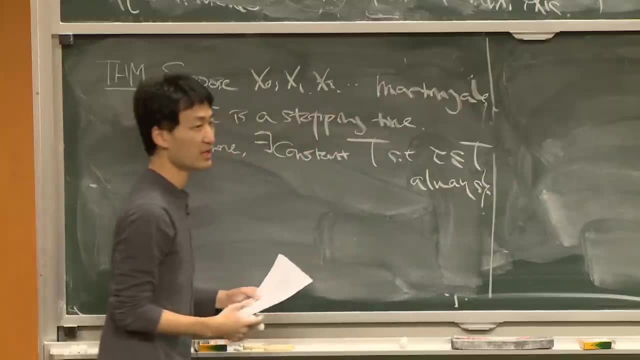 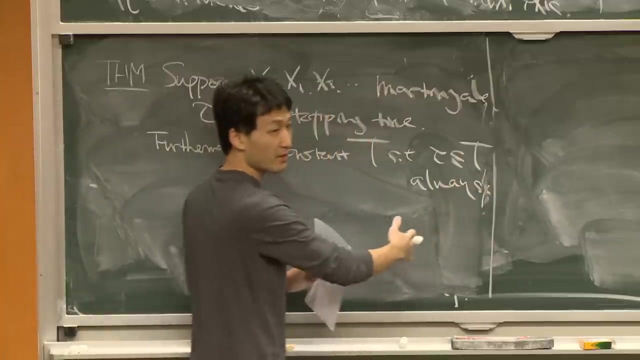 there exists a constant t, such that tau is less than or equal to t always. So you have some strategy which is a finite strategy. You can't go on forever. You have some bound on the time And your stopping time always ends before that time. 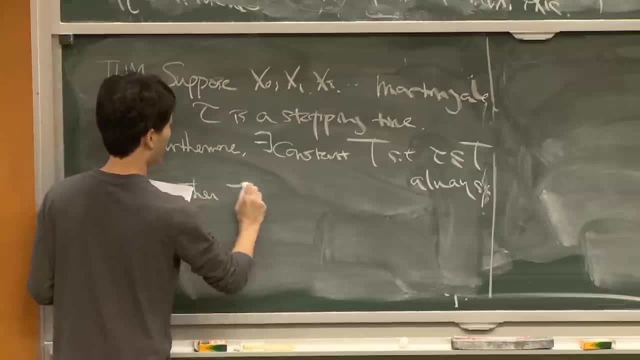 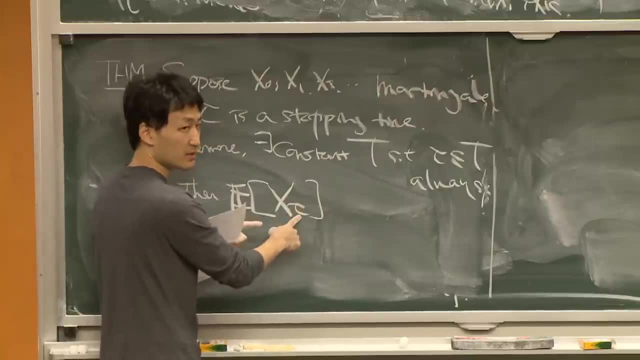 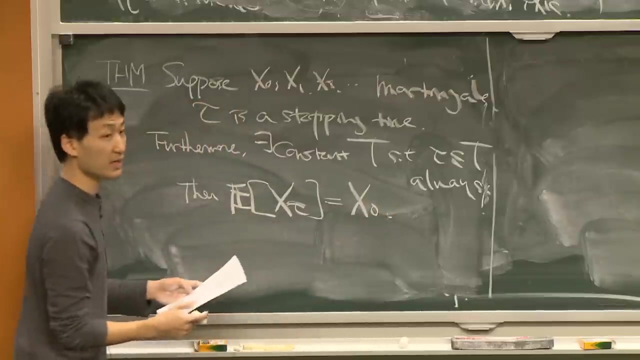 In that case, then, expectation of your value at the stopping time when you stopped your balance- if that's what it's modeling- is always equal to the balance at the beginning, No matter what strategy you use if you are a mortal being. 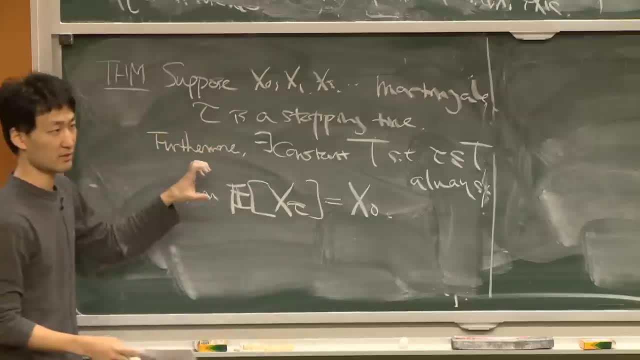 then you cannot win. That's the content of this theory. So, All right, I wanted to prove it, but I'll not because I think I'm running out of time. But let me show you one very interesting corollary of this. 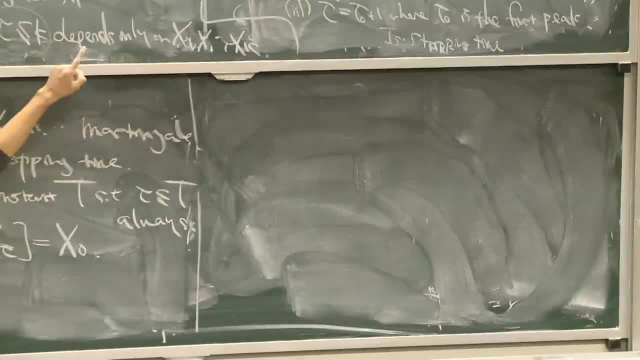 Apply to that number one. So number one is a stopping time. It's not clear that there is a bounded time where you always stop before that time, But this theorem does apply to that case. So I'll just forget about the technical issue.